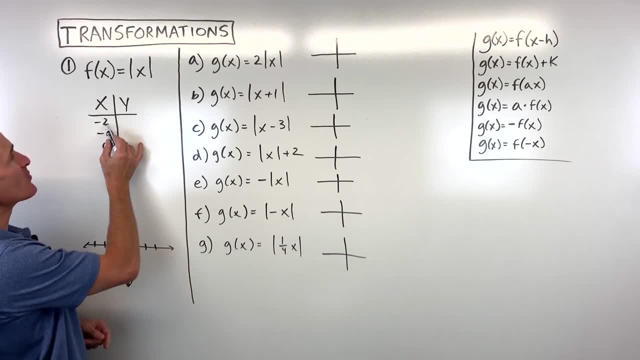 plug in some negative values- zero- and a couple positive values. remember, when you put this number in, it's always going to end up making it a positive in the end. So the absolute value of negative two is just going to be positive two. The absolute value of negative one is one. 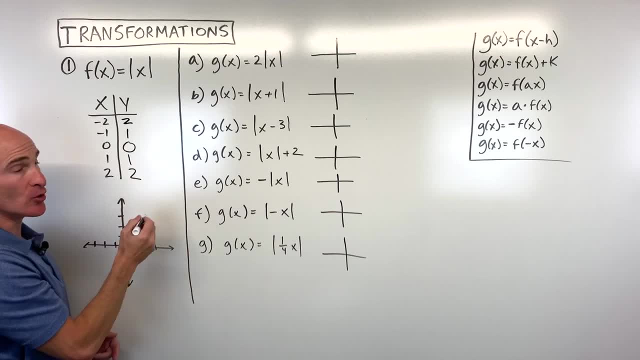 Absolute value of negative two is one. The absolute value of negative two is one. The absolute value of zero is zero, one and two. So if we plot these points here, you can see this is going to be negative two, two, negative one, one, zero, zero one, one, two, two, etc. And what? 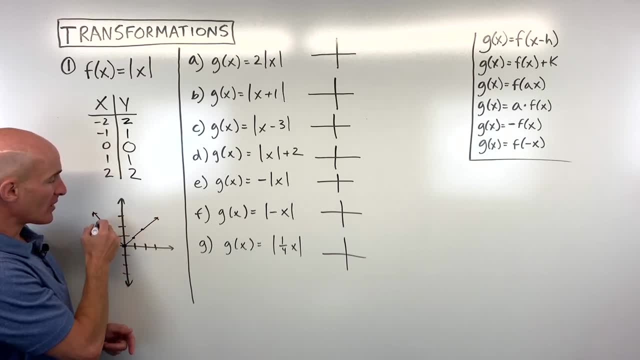 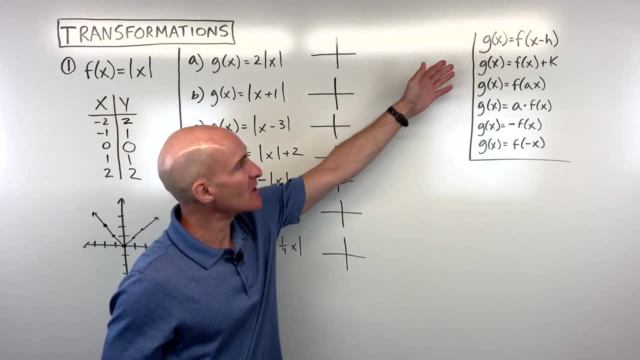 this graph looks like it's a real sharp corner here, like a v-shaped graph. But now let's go ahead and take a look at some different transformations here, And we're going to be using this function notation. a little bit later in the video We're going to be talking about how to 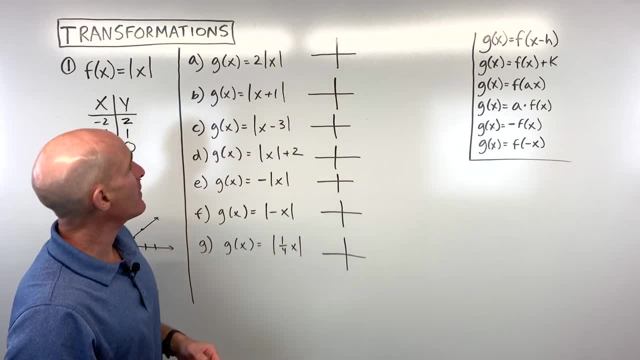 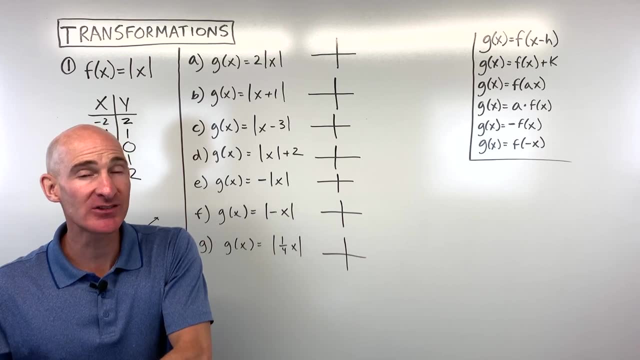 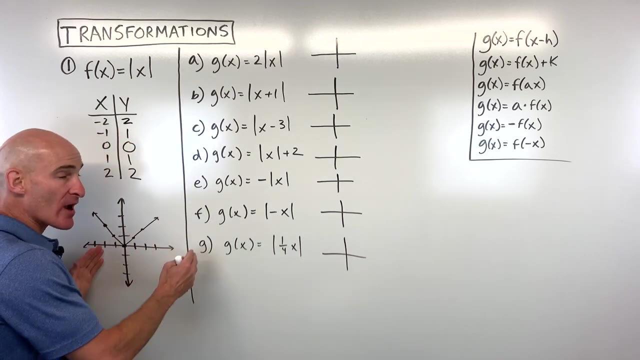 work with the transformations using this. But for just starting off here now, what we want to do is we want to ask ourselves: is the number grouped with the x or not grouped with the x? This is the way I like to think about it. If it's grouped with the x, it's going to affect the x-axis direction, the horizontal. 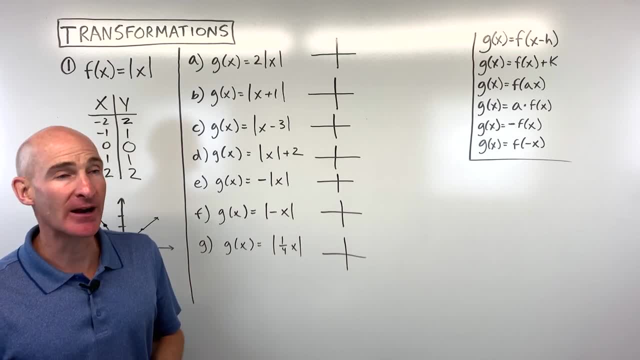 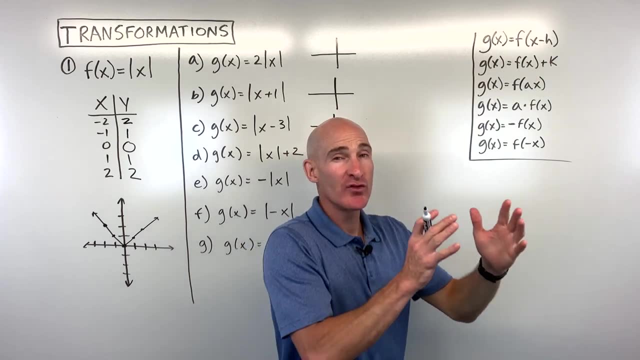 direction, but it's going to have the opposite effect. What I mean by that is see, like here, how we have f of x minus h. If it was x minus two, it actually would move the graph positive two to the right. If it was plus two, it actually would move the graph positive two to the right If it was plus two. 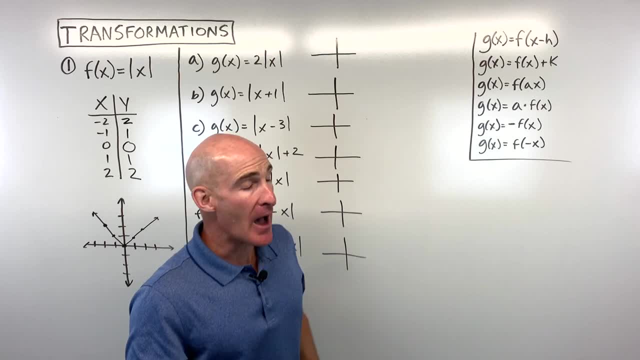 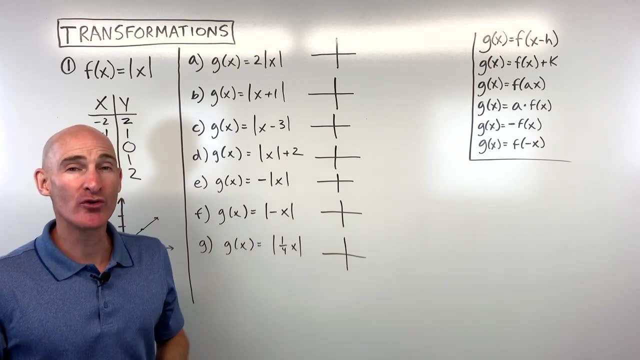 it actually would have the opposite effect. It would move it two to the left. But if it's not grouped with the x- meaning it's not in the absolute value bars or not underneath the square root or not in the parentheses- it's not grouped with the x and it's going to affect the y values and it's going to 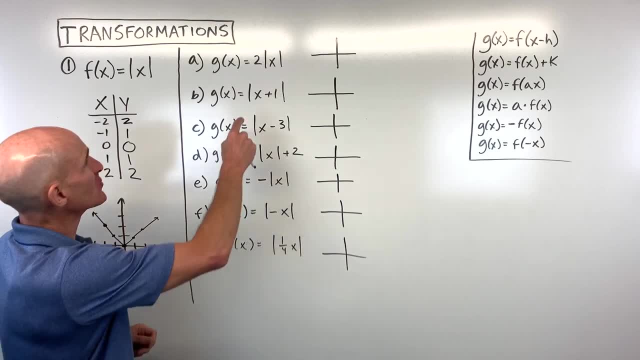 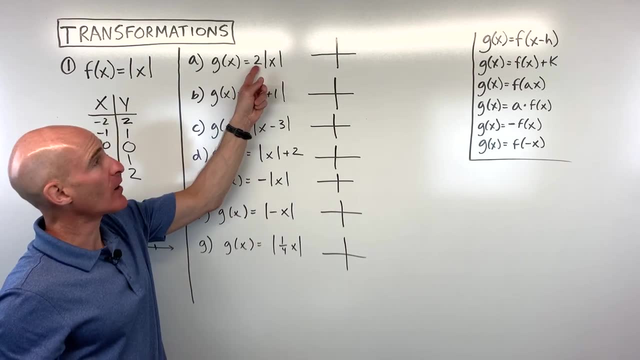 have what we call the same effect, And so we're going to talk about this. So in this first example, see how the two is not grouped with the x. This is going to be affecting the y values. It's going to be multiplying all the y values by two. We could multiply all these y values by two, but we're going to. 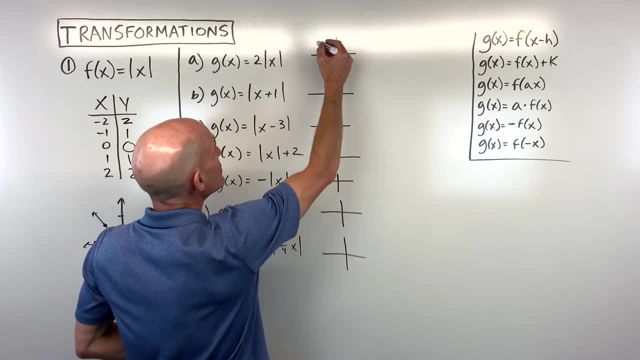 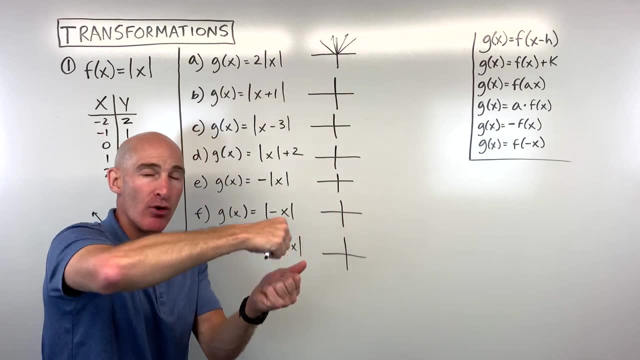 values in our table by two. but essentially, what's going to happen? if this is our original graph, this is actually going to be a vertical stretch by a factor of two. so it's like you're pulling on the graph in this y direction, the vertical direction which is going to make the graph. 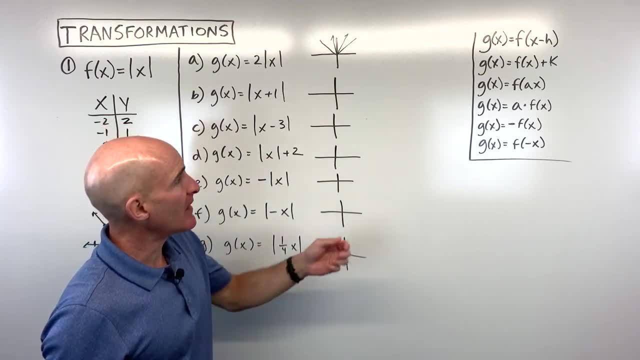 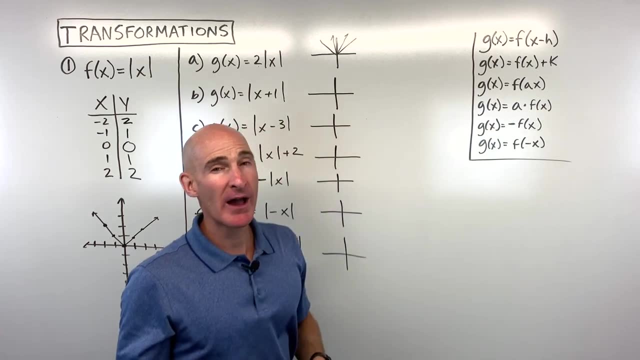 narrower, it's going up, you know, faster and again that's going to be. this one here in function notation, see how that a value is in front of the f of x, it's multiplied. when it's multiplied or divide is going to be a stretch or a shrink. when you're adding and subtracting, that's going to be. 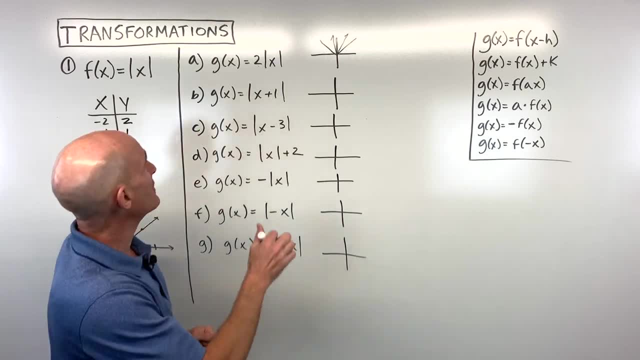 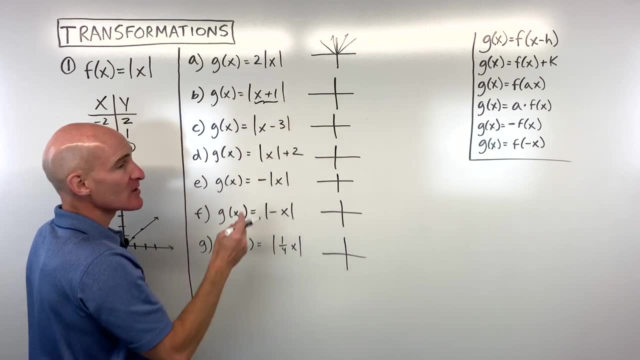 a shift, like you're picking it up and you're moving it. so let's go to the next one. g of x is equal to the absolute value of x plus one. now notice it's grouped with the x, so it's going to affect the x direction, the horizontal direction it's in addition, so adding and subtracting we're. 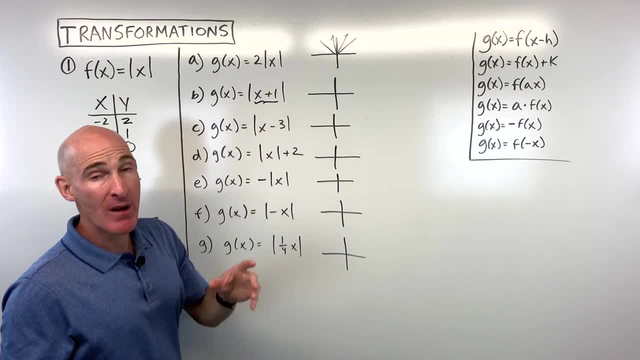 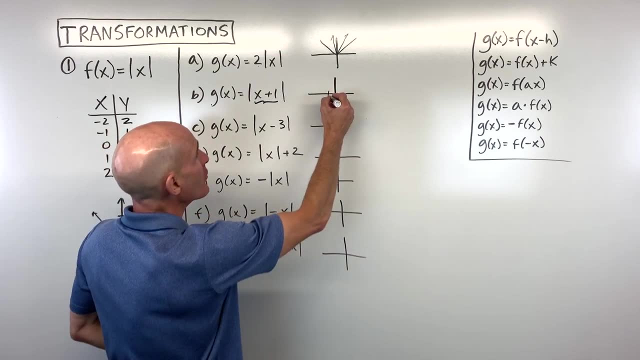 thinking of shifting right, picking it up and shifting. but remember, when it's grouped with the x, it has the opposite effect. so the plus one is actually going to move it to the left one. so now your graph is going to look something like this: where it's been shifted one unit to the 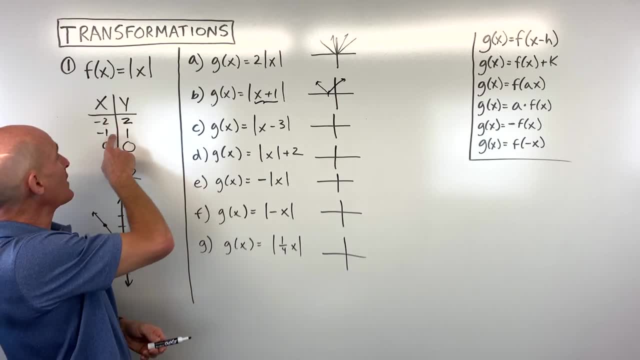 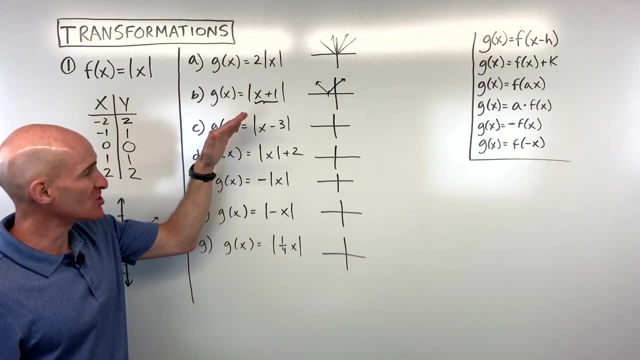 left. now, if you're working with the table, you can just subtract one from all these x values and then that would be your new point that you would want to graph, and we're going to do more problems as we go through this lesson. this is just kind of an introduction here. now for letter c. what do? 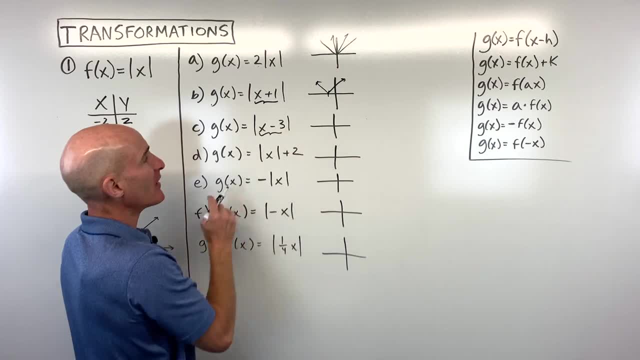 you think is happening on this one, g of x is equal to the absolute value of x minus 3, just like this one. it's grouped with the x, so it's going to affect the x direction. so it's going to affect the x direction. the x variable has the opposite effect when it's grouped with the x. the 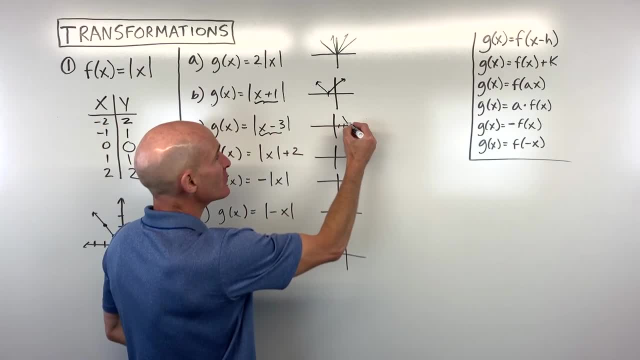 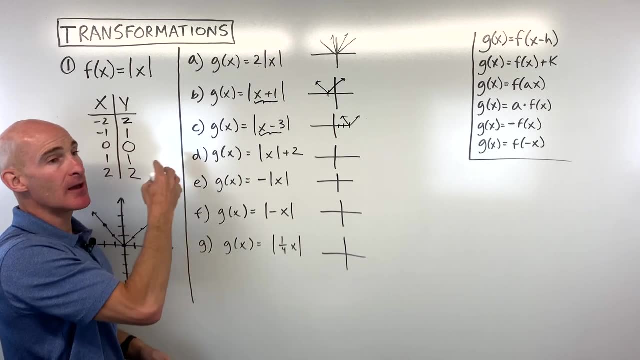 minus 3 is going to shift everything right 3, and so now our graph is going to look something like this: if you want to be a little bit more accurate with your table, you can just add 3 to all your x coordinates. plot those new points. that would be your graph. for letter d. we've got g of x equals. 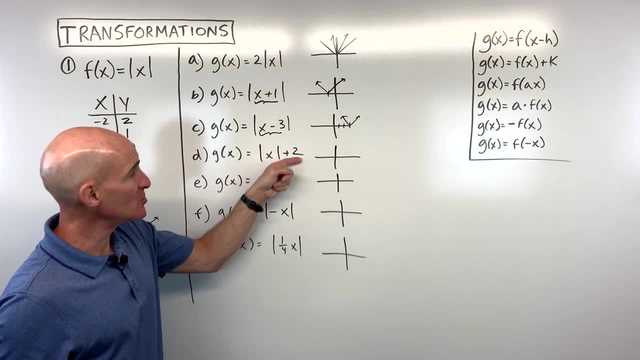 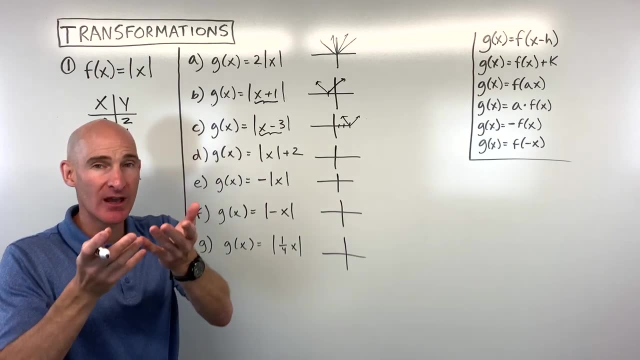 the absolute value of x plus 2. now notice that this 2 is not grouped with the x. it's not in the absolute value there. that means when it's not grouped with the x, it's going to affect the y values. okay, up and down, we're adding. that's going to be a shift. and when it's not grouped, 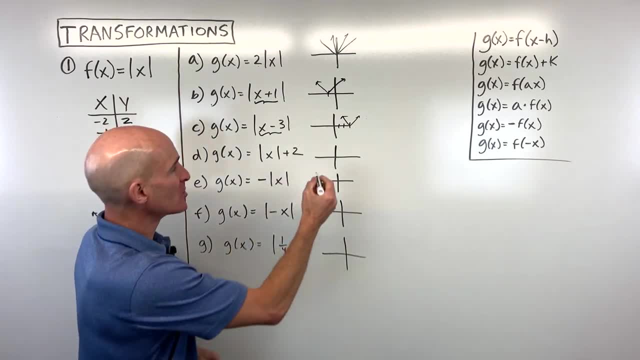 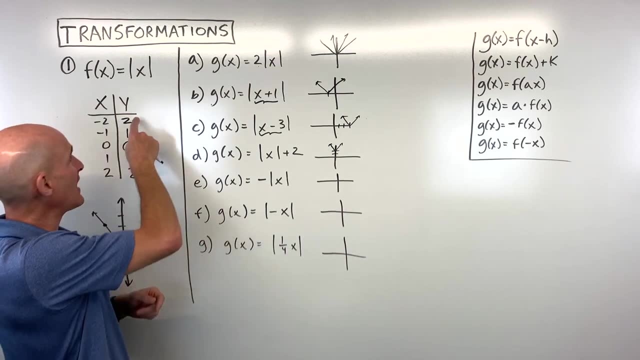 with the x, it has the same effect. so the plus 2 means we're going to shift this up 2 and it's going to have the same shape. it's just shifted up 2. now with the table, what you can do is just add 2 to all the y coordinates and then plot those new coordinates. that'll be your graph. 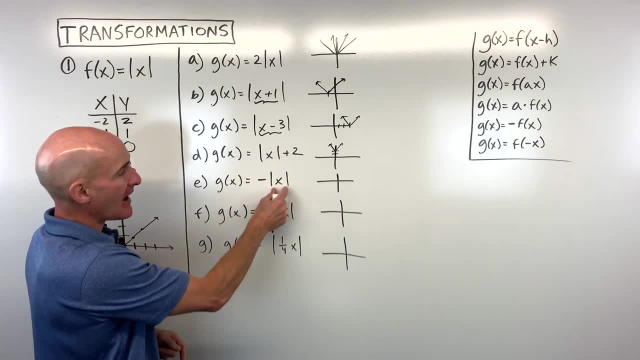 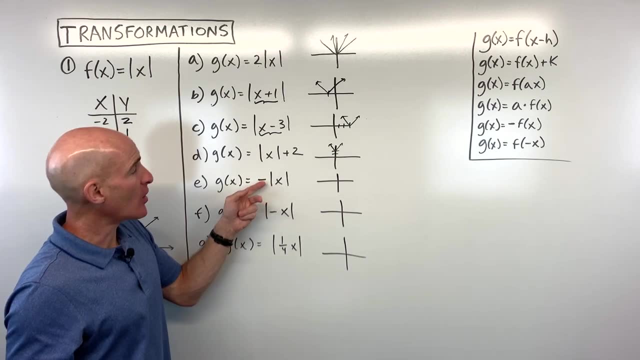 for letter e. notice: we have a negative on the outside. it's not grouped with the x. when it's not grouped with the x, it affects the y values, right? so it's going to make all the y values the opposite, or multiplied by negative 1. so what? 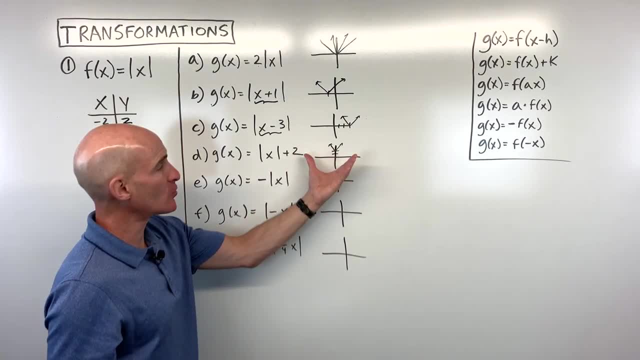 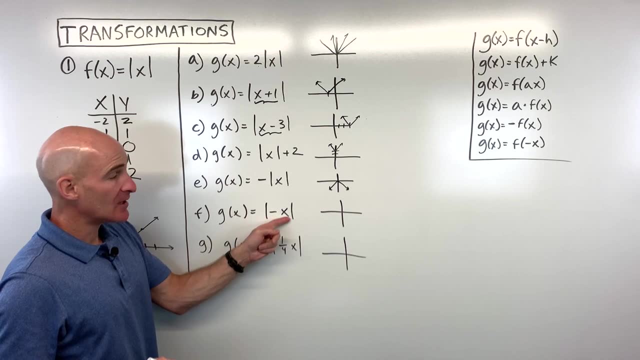 that's going to do is you multiply all these y values by negative 1. that's going to reflect it over the x axis, making it open down like that. whereas with letter f you see how the negative is grouped with the x, okay, see, it's inside those absolute value bars. that's going to affect the x. 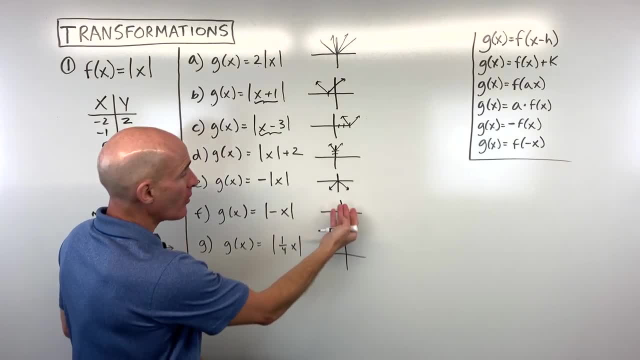 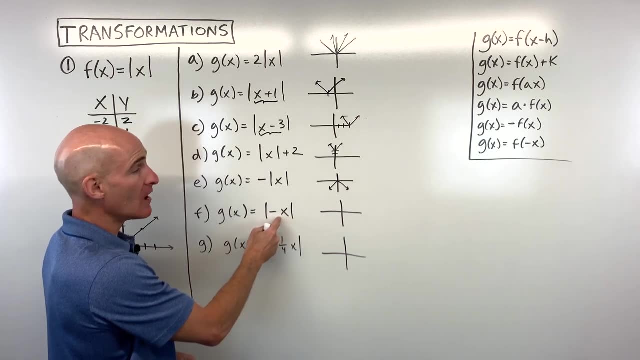 coordinates, or the x values, and it's going to make all the x values the opposite. so if they're positive, they become negative, if they're negative, they become positive. so this is actually a reflection over the y axis, because all the x's are opposite. now, when you take this graph, 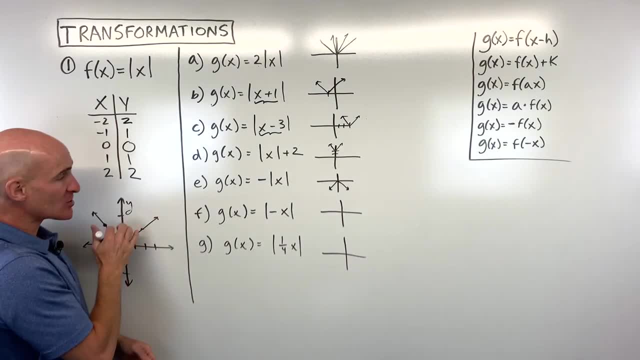 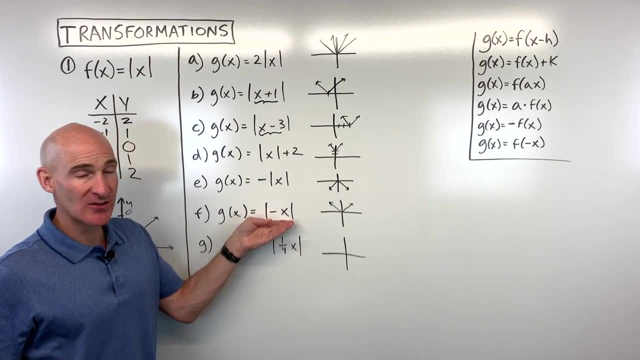 and you reflect it over the y axis. here it's just going to match to itself. so you're not really going to notice that the graphs changed in any way when you graph it. but as far as describing the transformation, you would say: oh yes, this is a reflection over the y axis. and then our last: 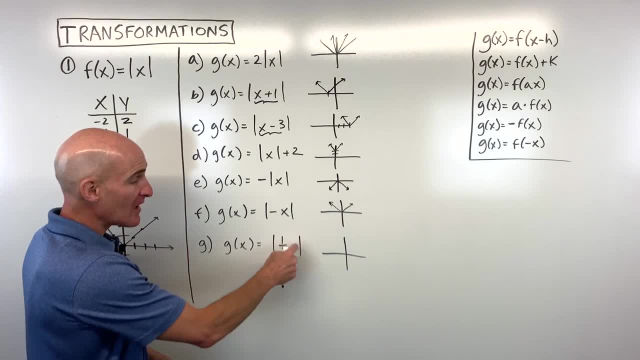 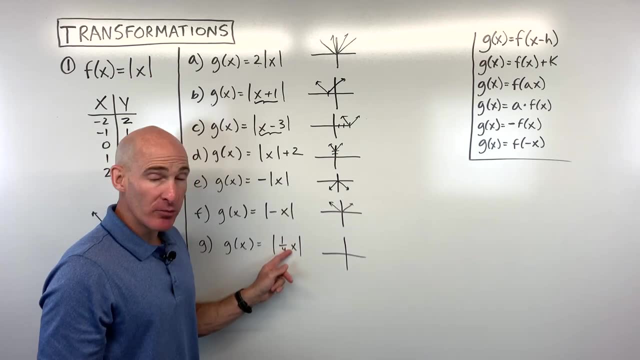 introductory example. here we have this: 1, 4th, grouped with the x. now, remember, when it's grouped with the x, it's affecting the x values. this horizontal line is what we're going to do here. direction, Notice it's multiplied. Remember: adding and subtracting is shifting, Multiplying. 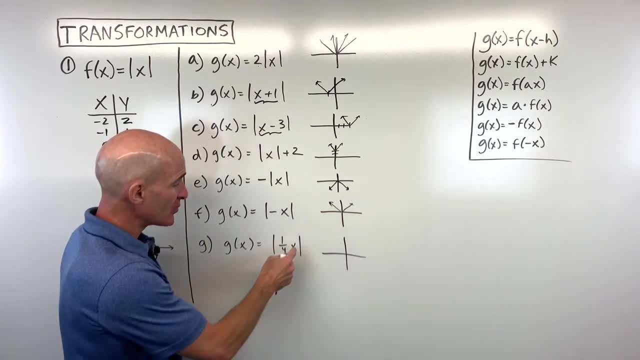 or dividing is like stretching or shrinking. But the important thing to remember, group with the x has the opposite effect, right? So the 1 fourth is actually going to multiply the x's by the reciprocal 4 over 1.. So this is actually going to be a horizontal stretch by a factor. 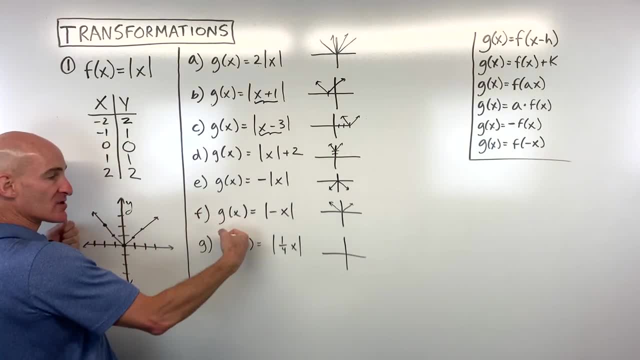 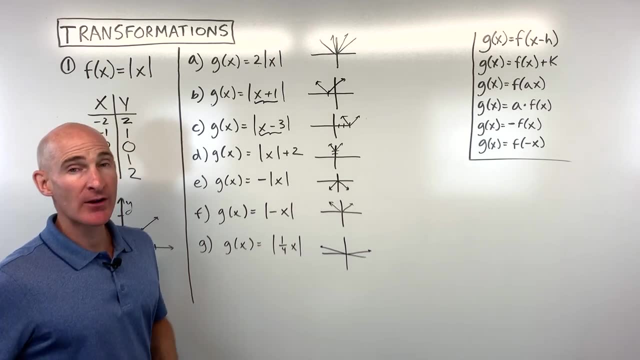 of 4.. So imagine taking this graph and pulling on it in this horizontal direction. That would make it wider, like so? Now, if you want to be more accurate, we're going to be more accurate. some of the next problems that we're going to be doing. I would just multiply all these x values. 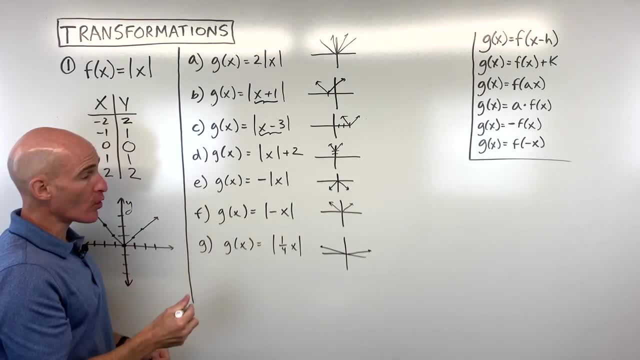 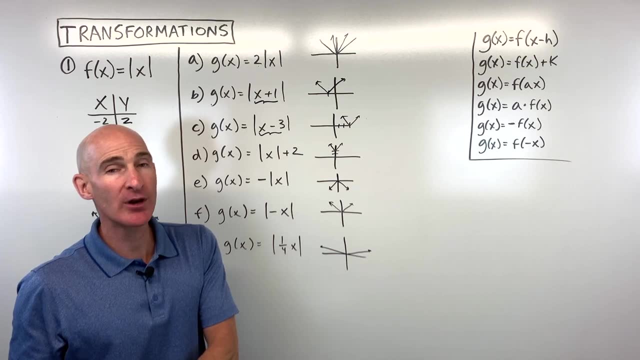 here by 4.. The y values would stay the same. Those would be our new coordinates and we can plot those and be real precise and get a nice graph. So let's take a look at some other parent functions that you're going to be encountering. Let's talk about how to graph them. Let's go to the next example. 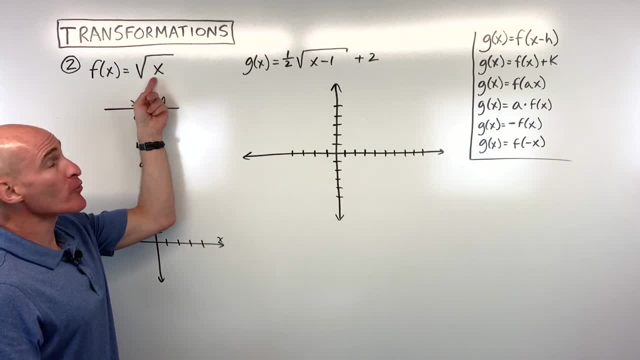 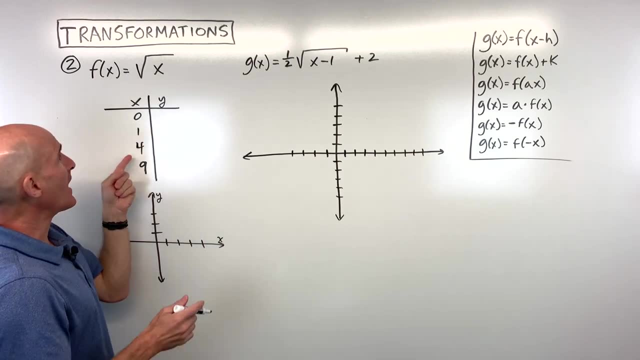 Okay, for example, number two. now let's look at this square root function. Let's plot this square root function. Let's plot this square root function. Let's plot this square root function. Let's plug in some easy numbers, Numbers that are easy to take the square root of, like 0,, 1,, 4, and 9.. 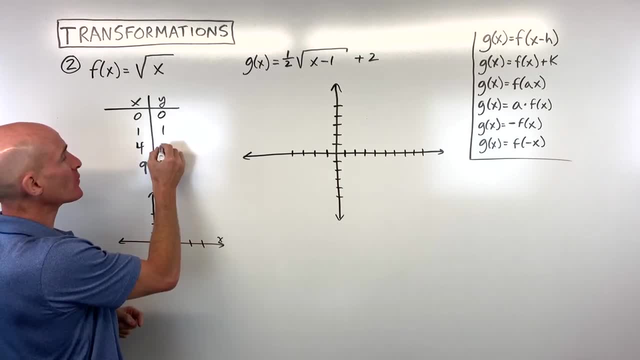 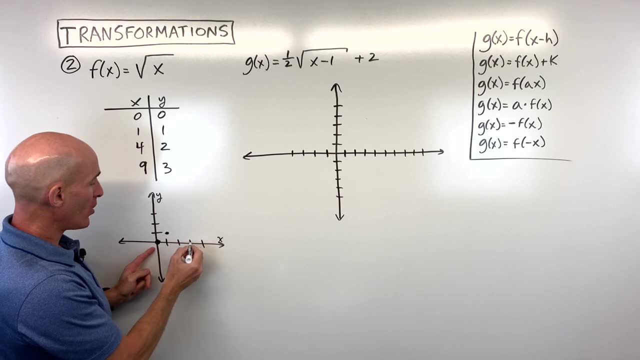 So the square root of 0 is 0,, square root of 1 is 1,, square root of 4 is 2, and square root of 9 is 3.. If we plot these points, we get 0,, 0,, 1,, 1,, 4,, 2, 9, 3.. Kind of goes off my graph a little bit here. 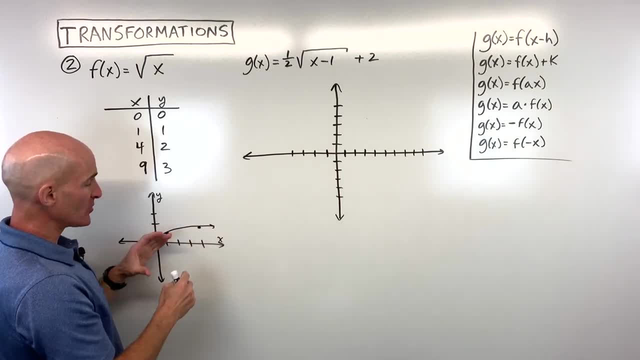 But you can see, this graph is just going to the right. It almost looks like a, like half a parabola on its side, like this. So it's gradually going up and it just goes to the right. Okay, like that. Now, what we want to graph now is this one here: g of x equals 1 half times the square root of x. 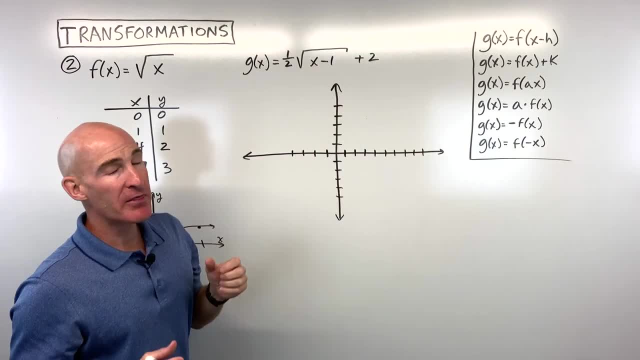 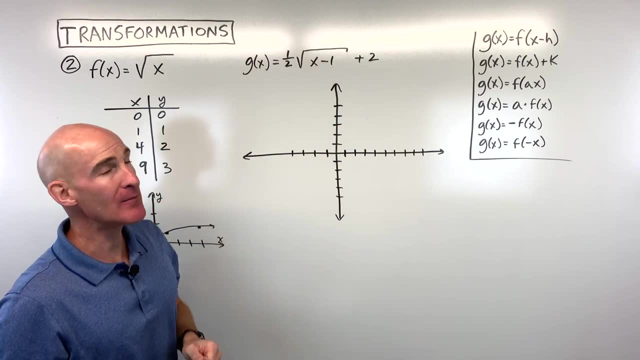 minus 1 plus 2.. So when I think about the order of transformations, the way I like to do it is, I like to think about working from the inside out. Okay, so what I mean by that is: you know, what are we? 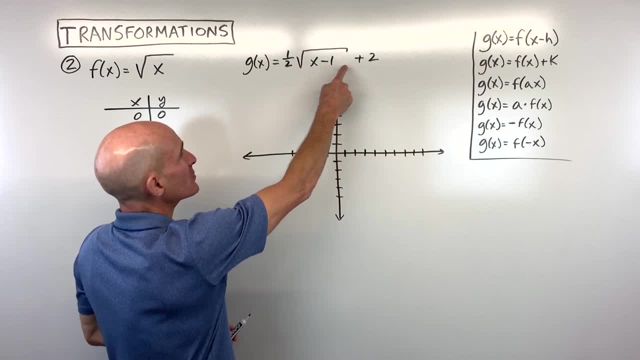 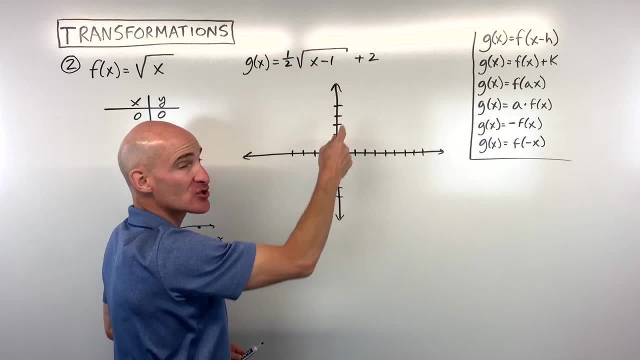 doing first? Are we doing the 1 first, the 2 first, the 1 half? What are we doing? So, starting from the inside out, I would say we're going to do the 1 first, then this 1 half and then this 2 last. So just to. 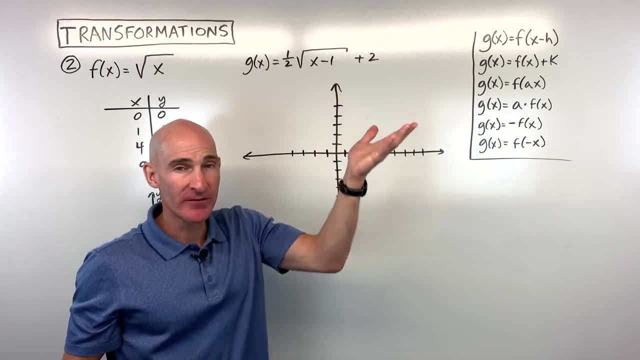 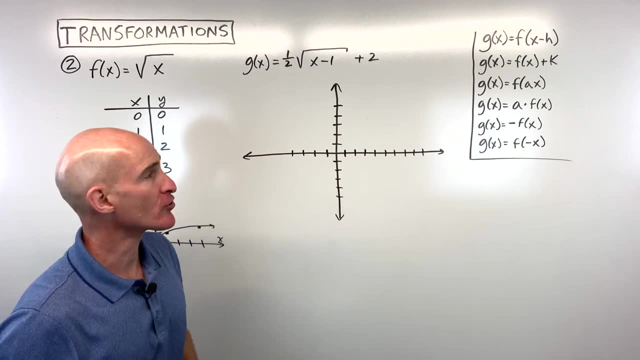 hint, you're going to want to do the vertical shift up or down last. Okay, some of the other transformations you can interchange and it's not going to affect the end result of your graph. Like, for example, I could do this 1, half and then the 1, or this 1 then the half. But in general, 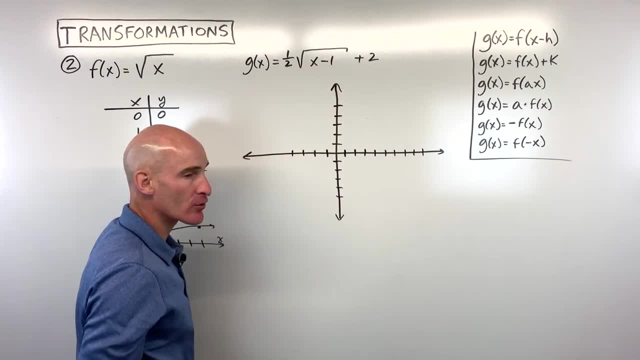 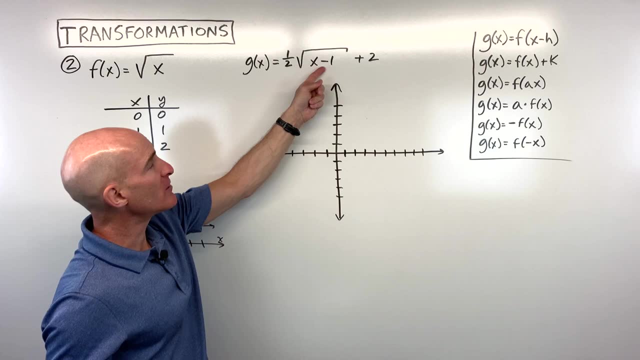 I kind of like to start from the inside and work my way out, making sure I do that vertical shift last. We're going to do some more challenging problems and we'll talk about it, But starting on the inside here, what do you think this minus 1 does to the graph? Well, I can see it's grouped. 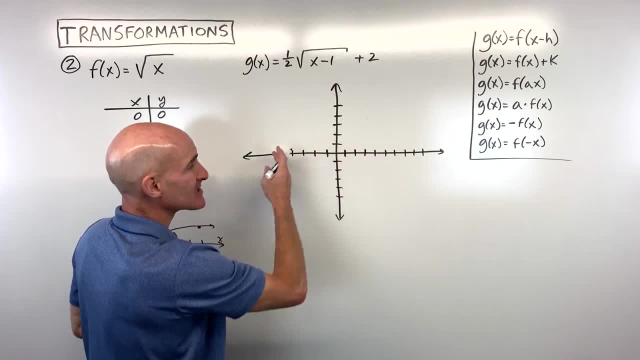 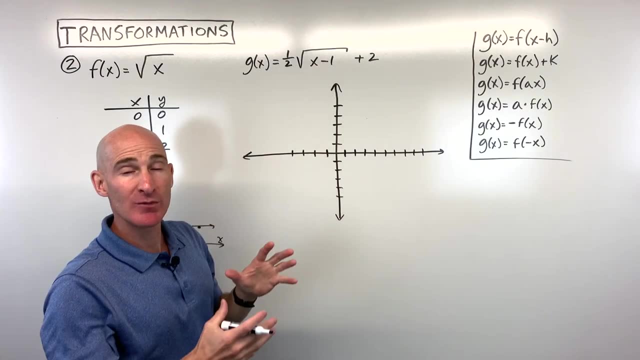 with the x. so that tells me it's going to be affecting the x variable, the horizontal component of the graph. It's subtracted. Remember, adding and subtracting is going to be a shift, like you're picking it up and you're like shifting it left or right, But remember when it's grouped with the x. 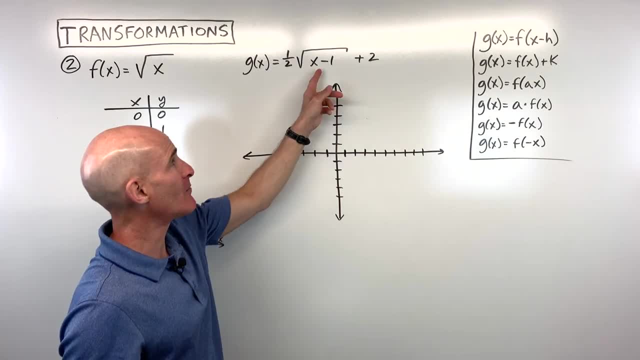 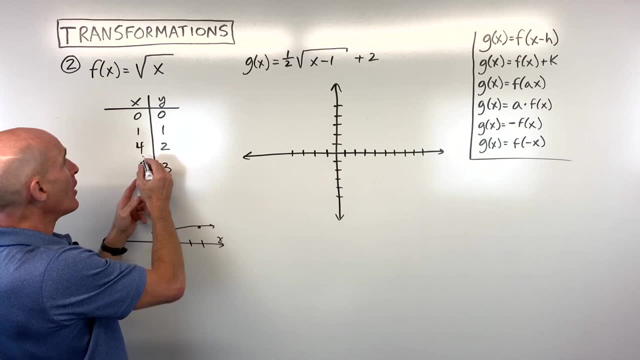 it has the opposite effect, right? So that means the minus 1 is actually going to shift this graph right 1.. Now, if we're looking at this from a perspective of the table, shifting right 1 means this is going to be 1, 1 plus 1 is 2,, 4 plus 1 is 5, and 9 plus 1 is 10.. So I'm going to cross out. 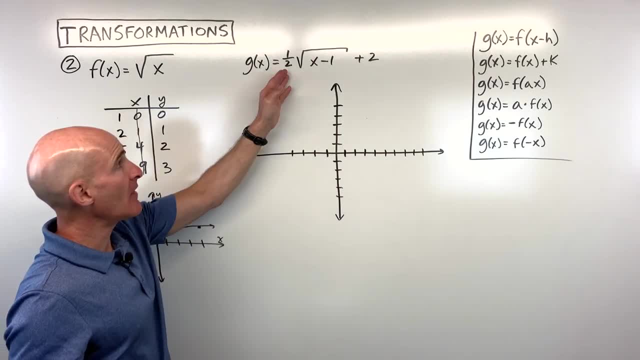 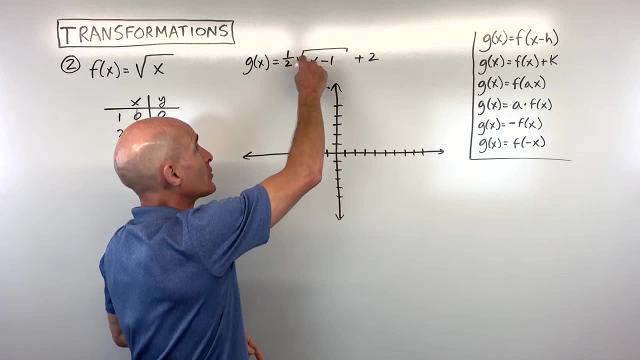 those old x values. These are our new ones. And then we're going to say the next thing, which is the 1 half. Now, the 1 half, is it grouped with the x? No, You can see, it's not underneath the square. 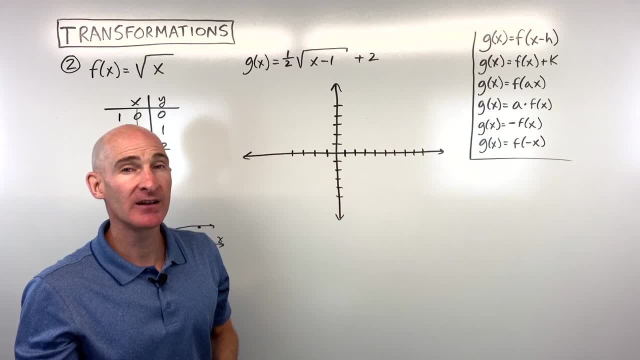 root. That means when it's not grouped with the x. which variable does it affect? The y values, right? If it's grouped with the x, it's affecting the x values. If it's not grouped with the x, it affects. 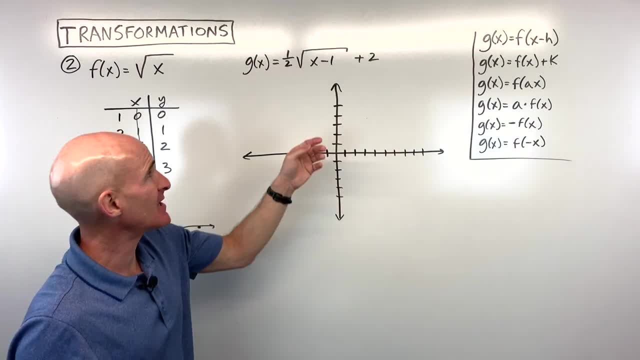 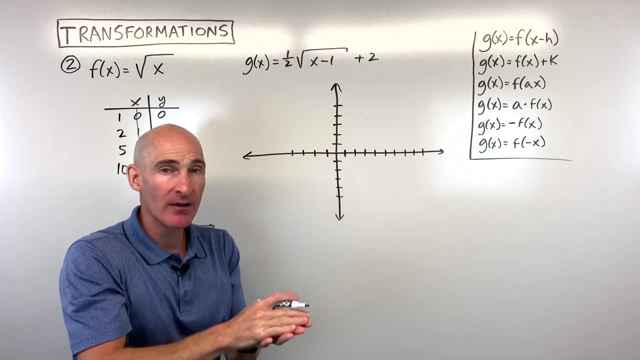 the y values, It has the same effect. What does that mean? the same effect. Well, see how the 1 half is less than 1? It's between 0 and 1? We say that this is a vertical shrink by a factor of 1 half. So that means we're going to multiply. 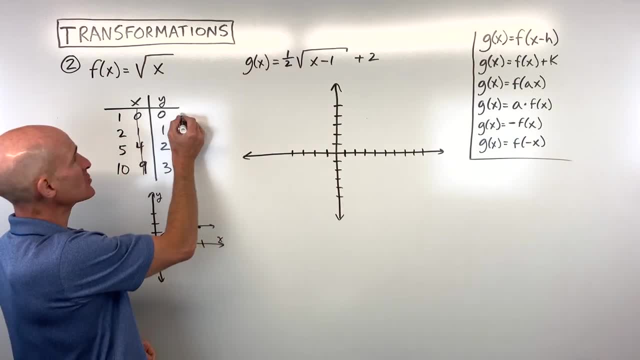 all the y values by 1 half. So that means this is going to be 0 times 1 half, which is 0.. 1 times 1 half, which is 1 half. 2 times 1 half is 1.. And 3 times 1 half is 1.5, or 3 halves. 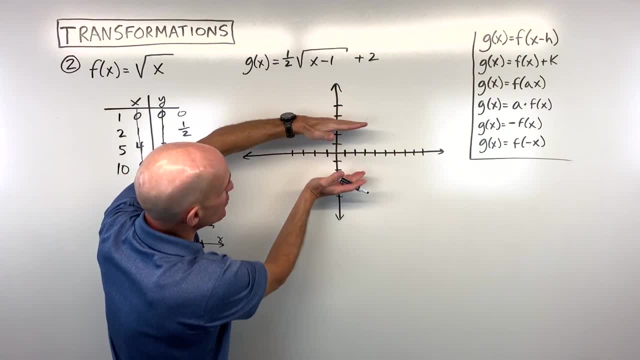 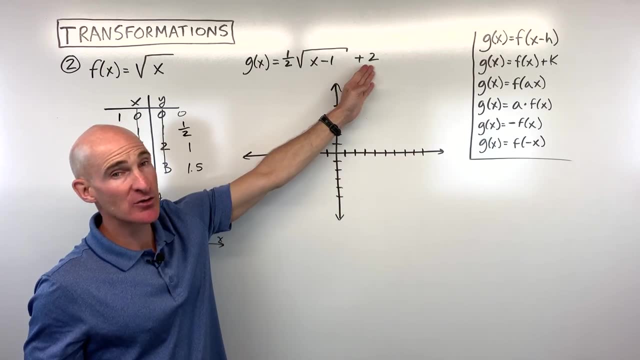 They cross out the old ones. But as far as the graph's concerned, it's like we're squeezing it towards the x-axis because that's a vertical shrink. So we're going to cross out the old ones, Vertical shrink by a factor of 1 half Now, lastly, remember we said we always want to do that. 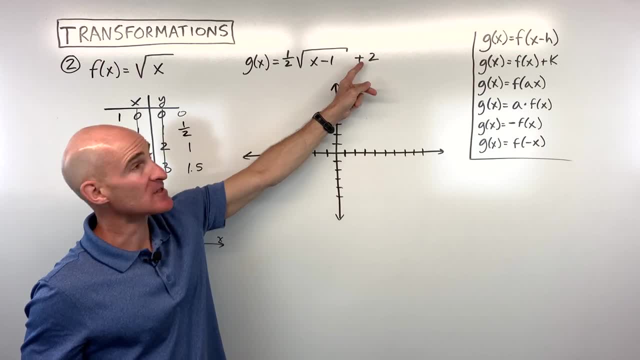 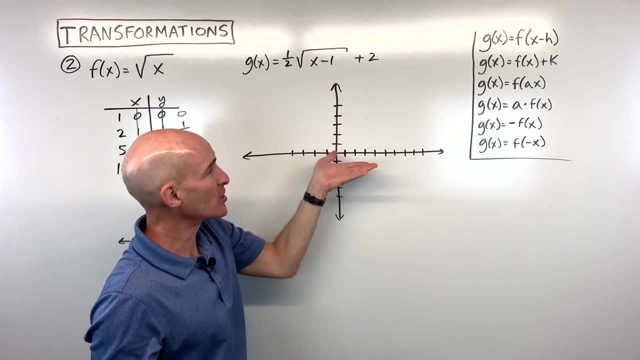 vertical shift up and down. last Notice: the 2 is not grouped with the x. So remember, when it's not grouped with the x, it affects the y values. It has the same effect, meaning plus 2, we're going to go up 2.. And notice, when you're adding, that's going to be a shift. So adding or subtracting. 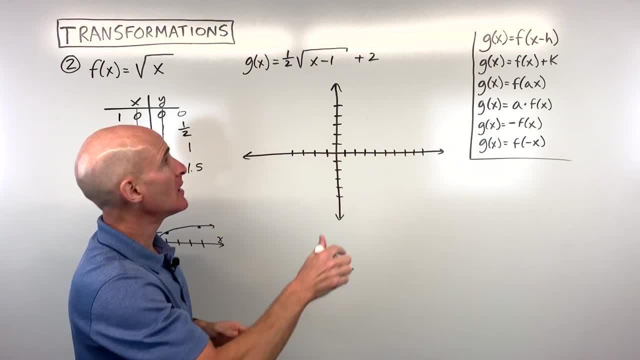 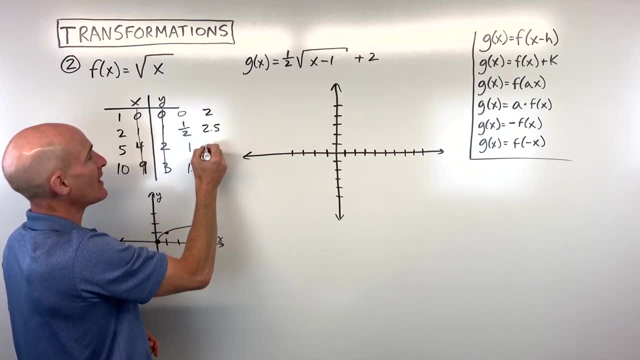 is a shift. Multiplying or dividing is like a stretch or a shrink, And so here we're going to be adding 2 to all the y values, because it's shifting up 2.. So that's going to be a shift. That's going to be 2, 2.5, 3, 3.5.. Let's cross out those old y values. Now we have everything we. 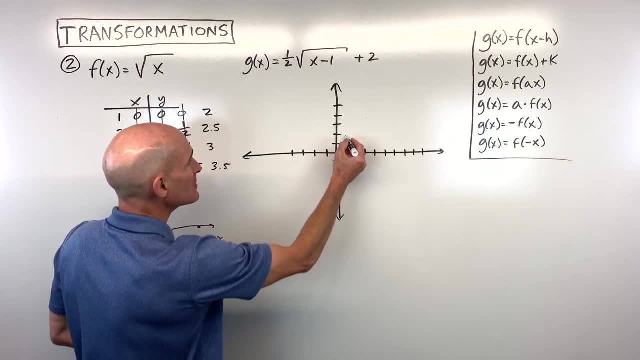 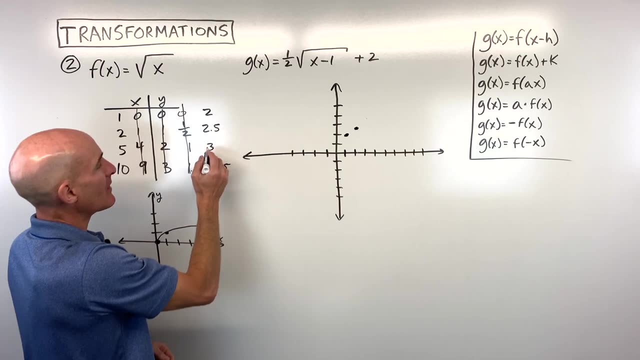 need to graph our graph. 1, 2 is where we're starting. 2, 2.5, right about here- 5, 3.. So let's see: 1, 2, 3, 4, 5, 3 is right about here And 10, 3.5.. Kind of goes off the graph a little. 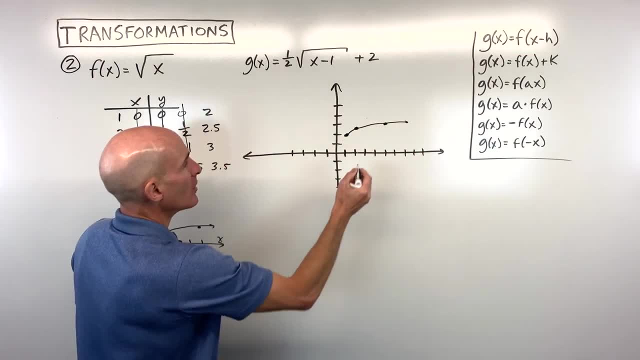 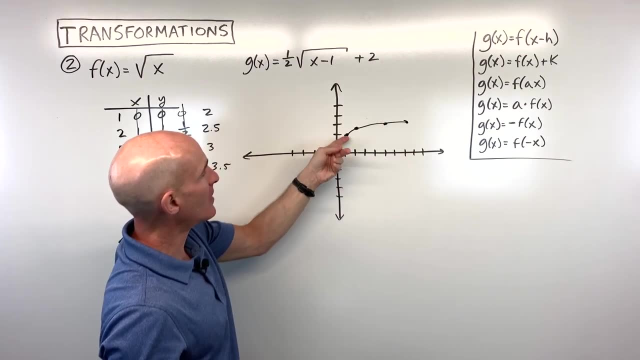 bit Basically. you can see our graph now. You can see it's a little bit squished. That was what the 1.5 did And the 1, you can see- shifted at right 1.. The 2 shifted it up 2. And that's our graph. So great job, Let's. 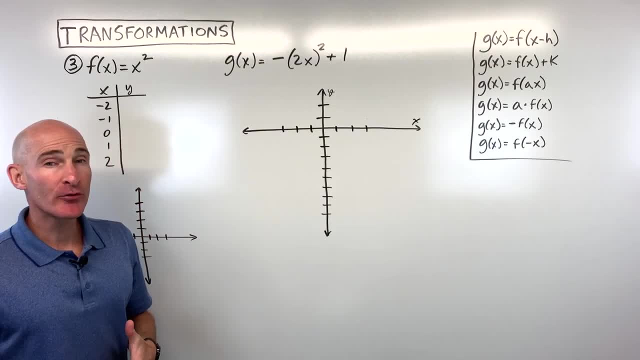 go. look at another example. Okay, for example number 3. now we're working with this function: f of x equals x squared. This is called our quadratic function, And let's make a table, like we've been doing. We'll plot some easy numbers. So negative 2 squared is negative 2 times negative. 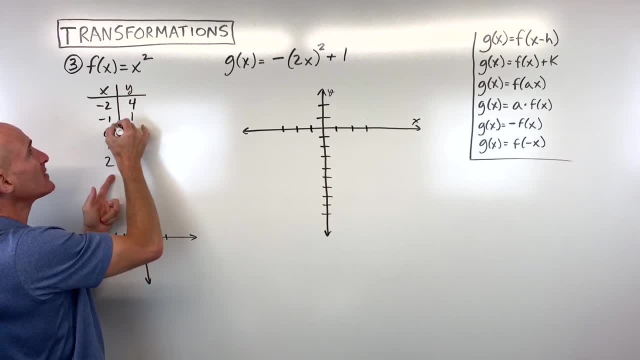 2, or positive, 4.. Negative: 1 squared is 1.. 0 squared is 0.. 1 squared is 1.. 2 squared is 4.. 3 squared is 9, etc. Now, if we plot these points, you're probably already familiar with this graph, But this is: 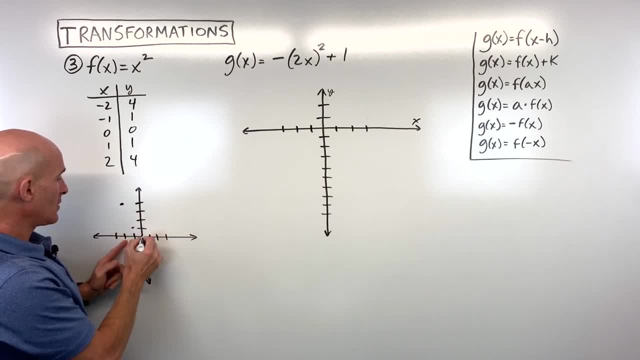 going to look like a parabola, which is basically a u-shaped graph, And you can see kind of what that's doing. It's going up kind of like steeper and steeper. So this is our parent function. Now we want to graph this one: g of x equals negative the. 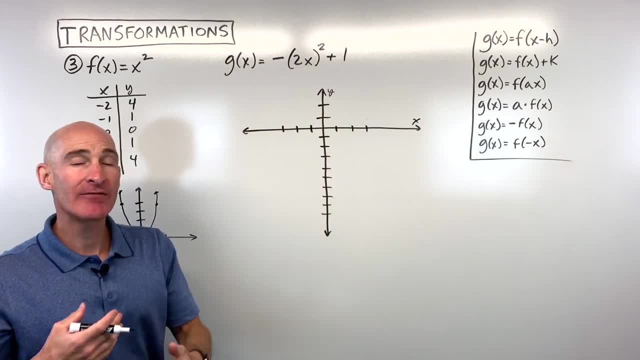 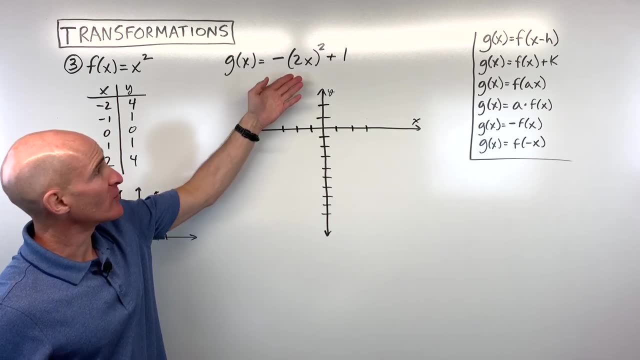 2x squared plus 1.. And we want to identify the order of transformations, meaning what do we do first and second and third, etc. So what I like to do is I like to work from the inside out. I look at where that variable x is, The x represents like our input, And we say, well, what's happening to? 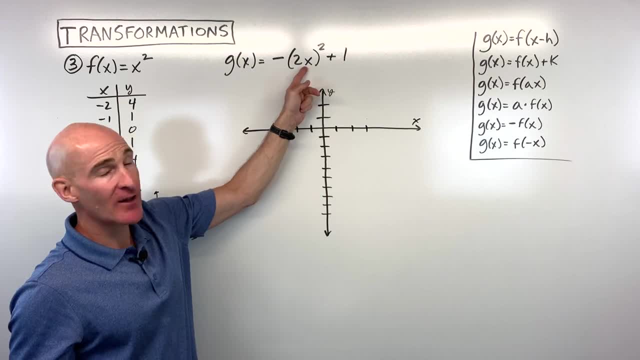 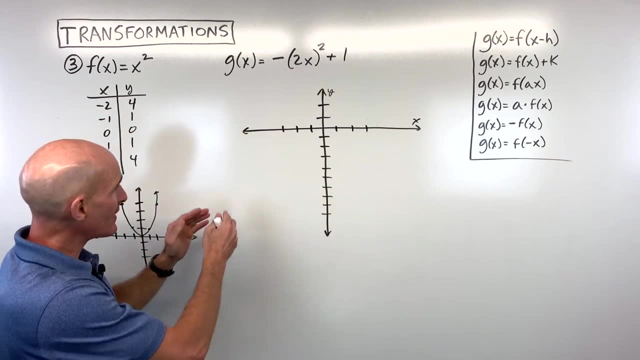 that input. Well, it looks like we're multiplying the x values by 2.. But remember we say: is it grouped with the x? Yeah, this 2 is grouped with the x. So that means it is going to be affecting the x direction, the x variable, the x value. So we're going to work from the inside out And we're 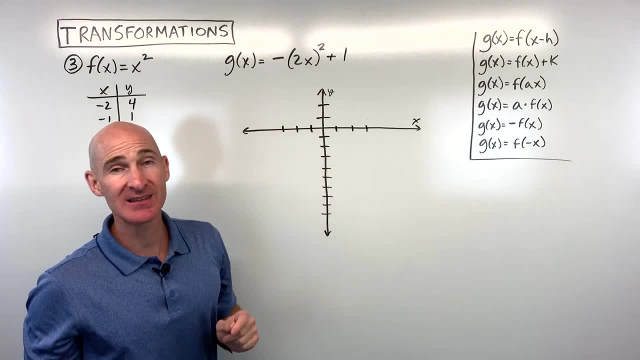 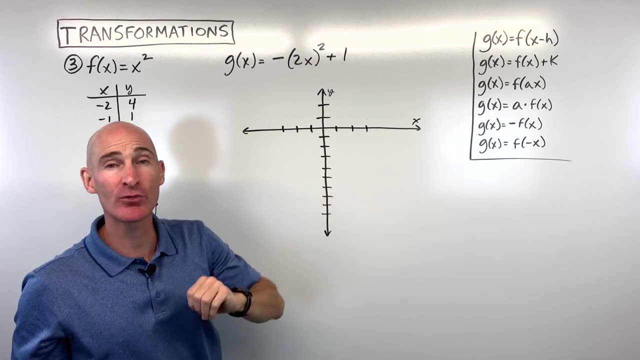 going to look at the horizontal component, But when it's grouped with the x, it has the opposite effect. So we're actually dividing the x's by 2.. Or you could say: dividing by 2 is like multiplying by the reciprocal 1 half. So I would say that the first step is that this is a horizontal shrink. 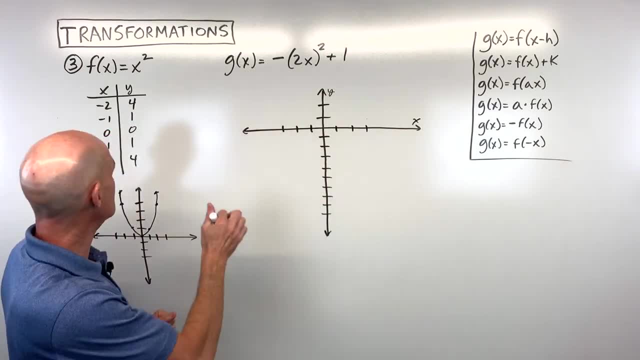 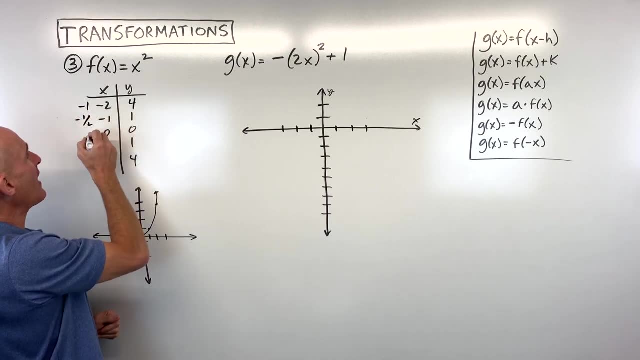 by a factor of 1 half. Now what that does to the table here. it's going to multiply all these x values by 1 half, which is going to make this negative 1, negative 1 half. 0 times 1 half is. 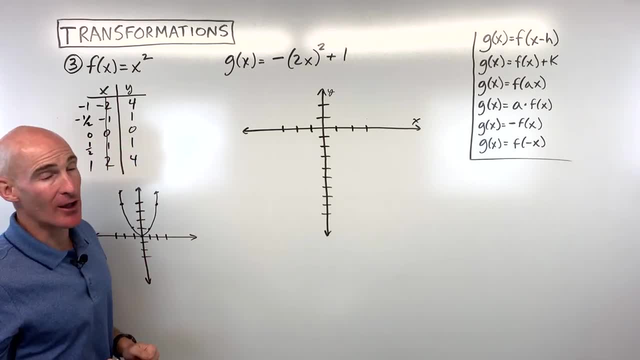 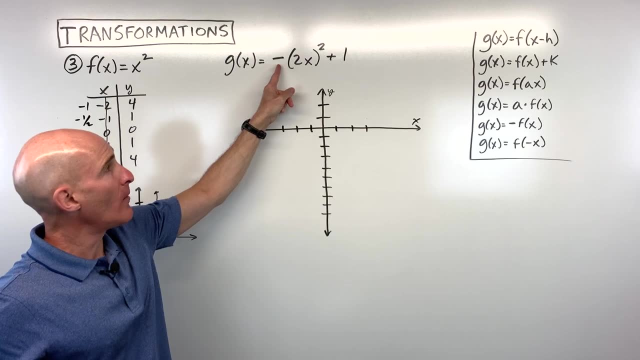 0,, 1 half and 1.. Let's cross out those old x values Now. the next thing, kind of working from the inside out, would be this negative here. Now, what does this negative do? Well, you can see that. 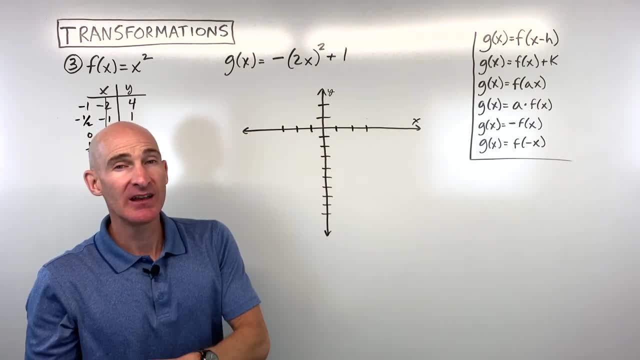 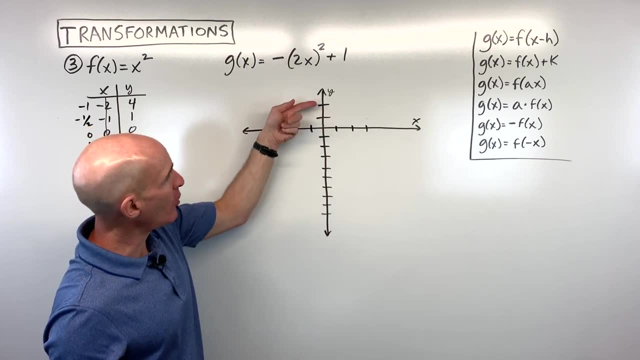 it's not grouped with the x. Remember, when it's not grouped with the x, it affects the y values, right? And so it's going to multiply all the y values by negative 1.. Now, when you multiply all the y values by negative 1, the positive y values become negative If they have negative y values. 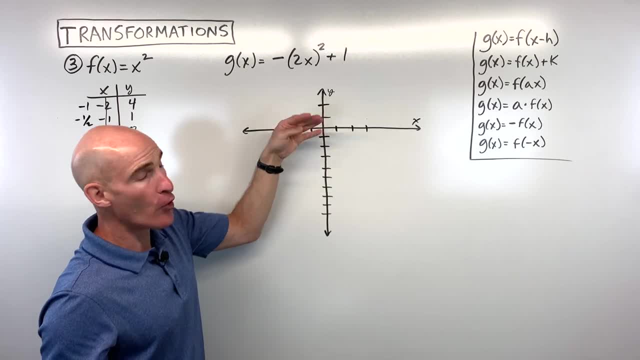 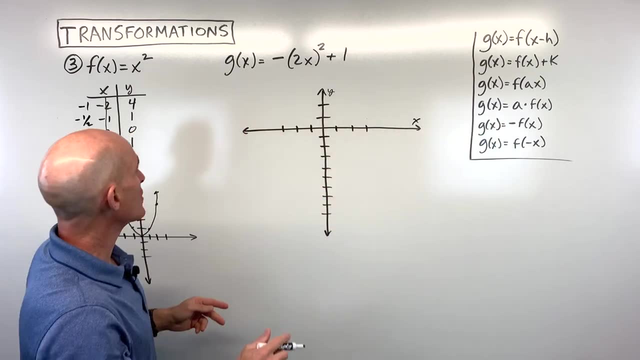 they become positive. So what that's doing is it's reflecting it over the x-axis. In function notation that would look like this, where the function is multiplied by negative 1.. So we're going to multiply all these y values by negative. 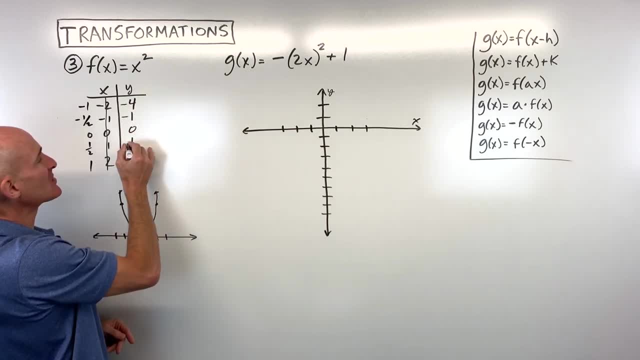 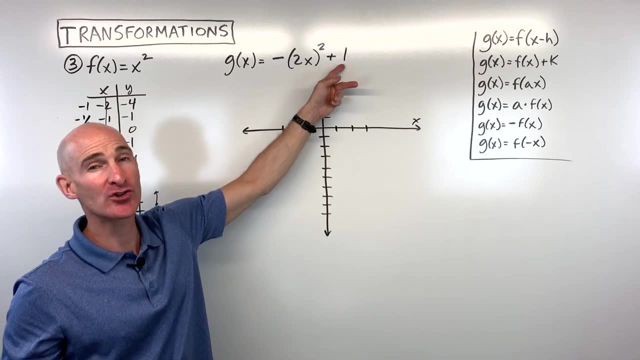 1. So this is going to become negative negative 0 times negative. 1 is still 0, negative negative. Okay. now, lastly, is the plus 1.. And remember, we said we always want to do that vertical shift. 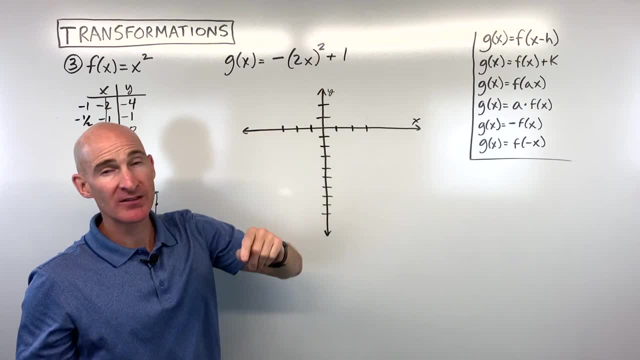 last right. So the plus 1, the way I like to think about it is, if you want, kind of like a decision tree and a lot of students want to know: what do I do? a, b, c, d, What do I do? 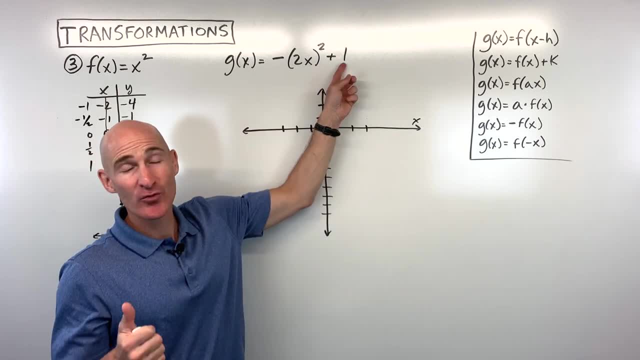 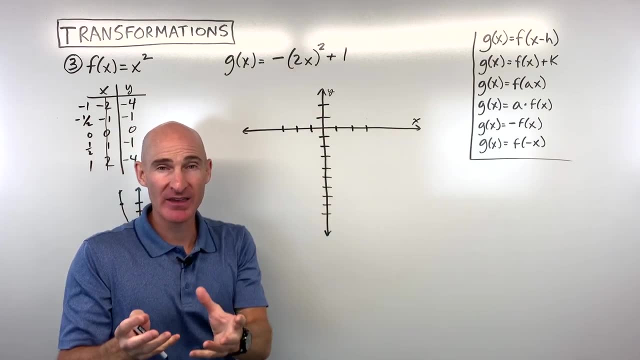 first, second, third, right. Ask yourself: is it grouped with the x? You might even want to write this down: Is it grouped with the x or not? grouped with the x? Not grouped with the x right. It's not in the parentheses, it's not with the x right, So that's going to affect the x values or the y. 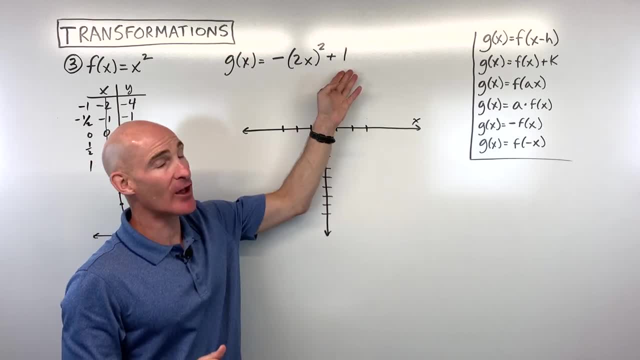 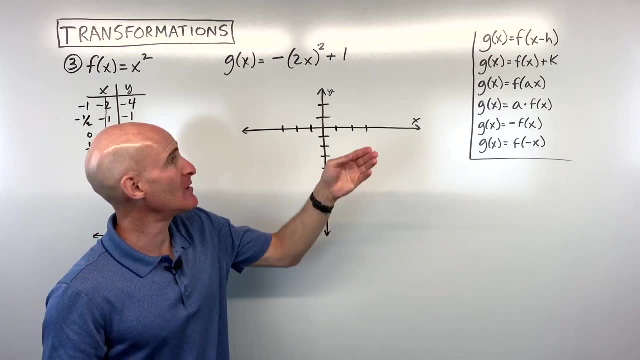 values, The y values, right. When it's not grouped with the x, it affects the y values. When it's grouped with the x, remember, it has the opposite effect. When it's not grouped with the x, it has the same effect. What I mean by that is see the plus 1,. intuitively, you'd think: oh yeah, plus 1,. 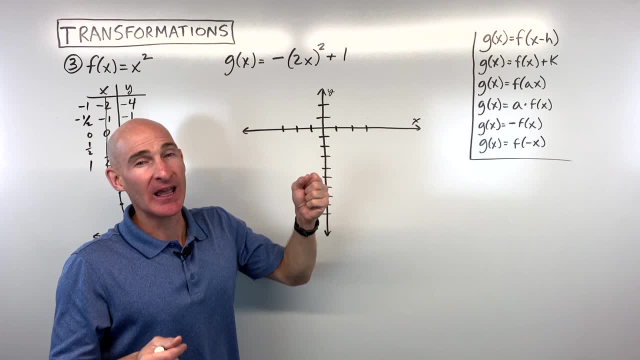 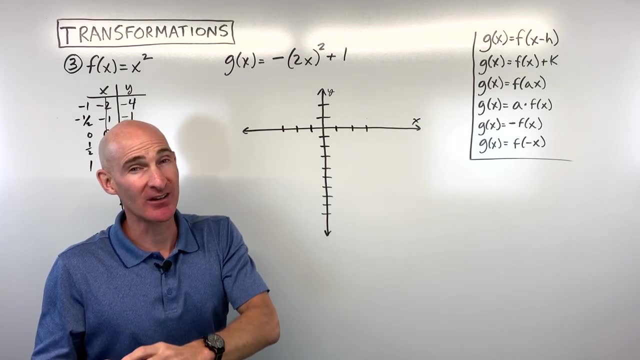 that means it's getting bigger by 1, it's shifting up 1, right, Okay. and the other thing you want to remember is: multiplying and dividing is stretching and shrinking okay. Adding and subtracting is shifting okay. So in this case, plus 1 means it's a shift, has the same effect. 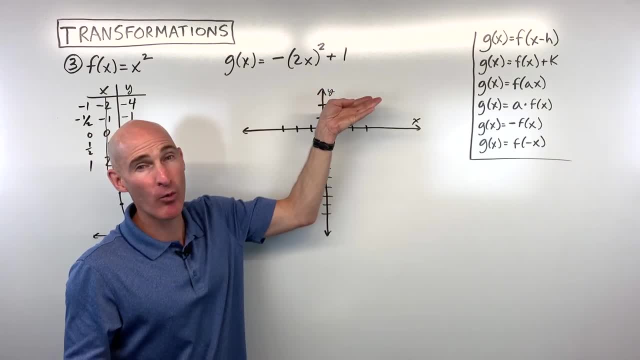 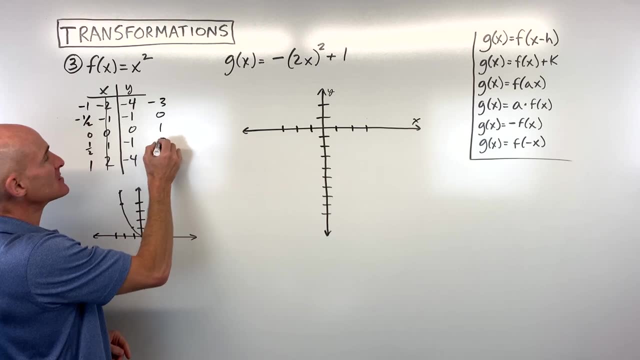 because it's not grouped with the x, it's affecting the y values. we're going up 1.. Do you follow that? So if I add 1 to all of these, this is going to be negative 3, 0,, 1, 0, and negative 3.. Cross. 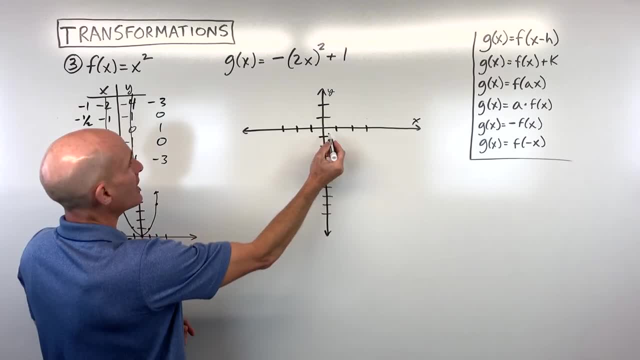 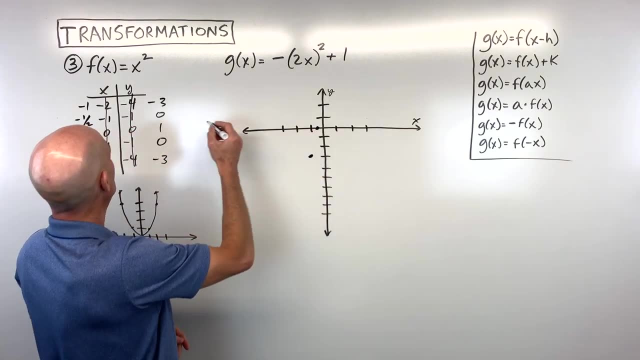 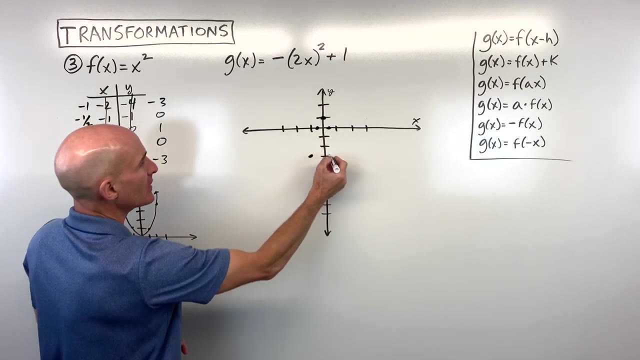 out the old y values. Let's go ahead and plot these. now We've got negative 1, negative 3, negative one-half 0, 0, 1, one-half 0, and 1, negative 3.. 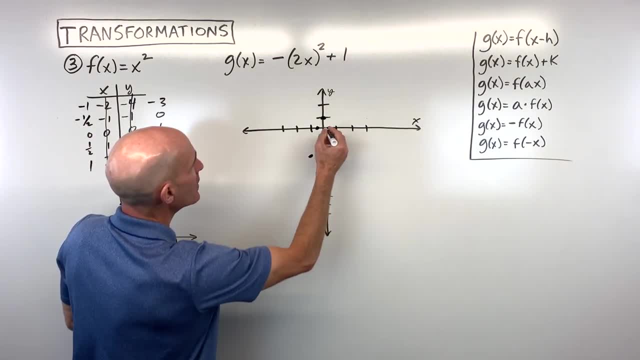 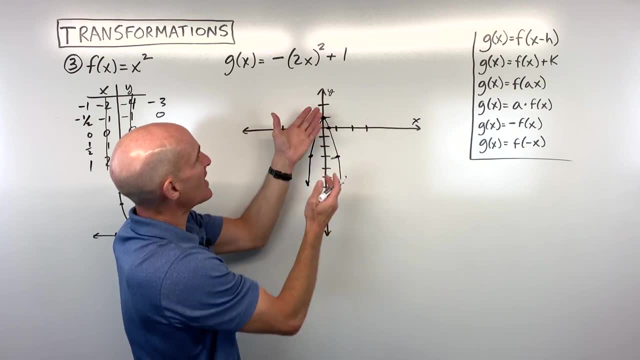 Let's see a little bit over here about right here. So basically what's happening is you can kind of see, well, the two basically shrunk it horizontally. so instead of being like this, it's more like this: The negative is reflecting it. 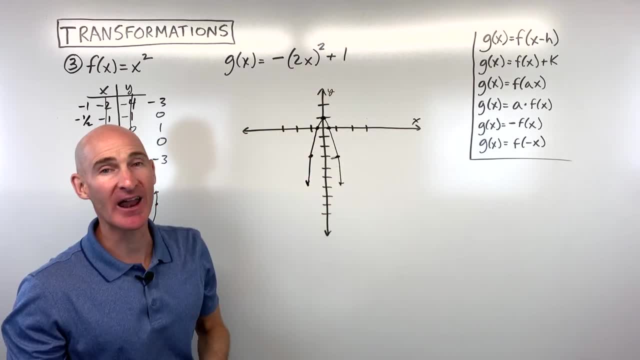 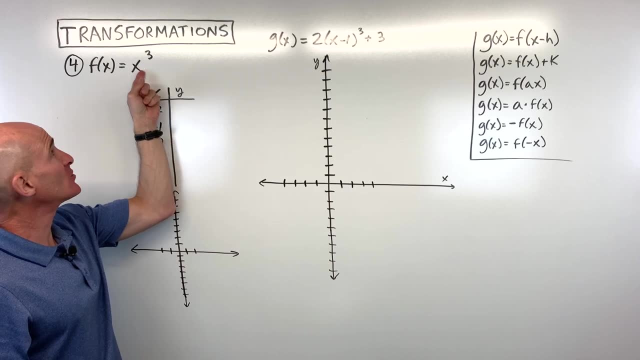 The plus 1 is shifting it up one. So there's our graph, and you got it. Let's look at another example. Okay, so for example number four, now we're working with the cubic function. f of x equals x to the third power. That's called our cubic function. Let's again plot some easy points. 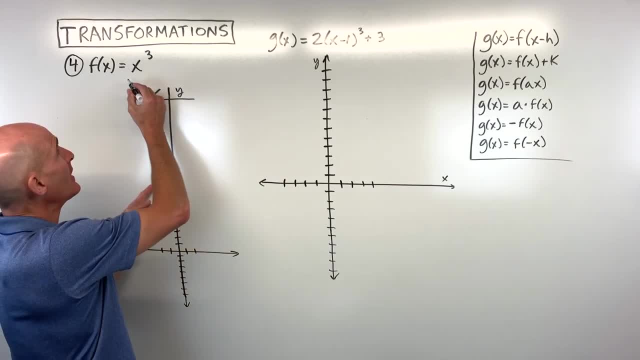 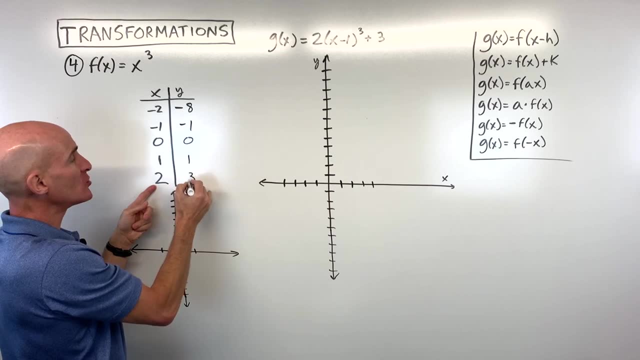 So negative 2, negative 1,, 0,, 1, and 2.. Negative 2 cubed is negative 8.. Negative 1 cubed is negative 1.. 0 cubed is 0.. 1 cubed is 1, and 2 cubed is 8.. And if we plot those points, let's see what we. 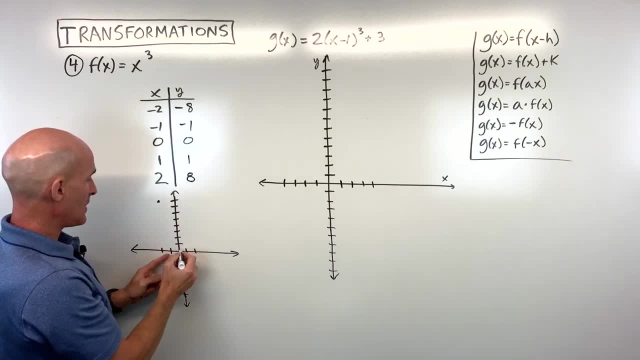 get here. So negative 2, up 8.. Negative 1 cubed is negative. oops, I made a mistake here. Negative 2, negative 8 is down here my mistake. Negative 1, negative 1,, 0,, 0,, 1, 1, and 2, 8.. So basically. 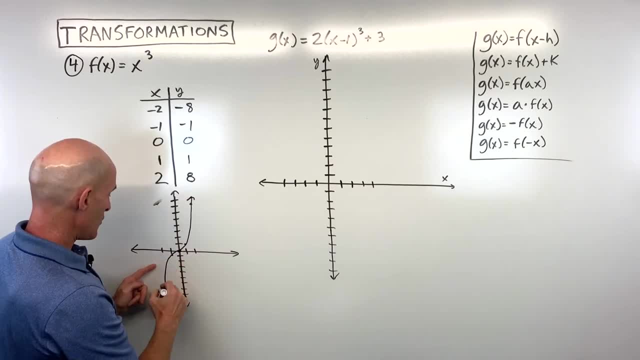 your graph looks like this, Okay, and it goes down and up forever and ever, Gradually goes to left and right forever and ever. Domain and range is all real numbers. So this is your parent function, your basic core graph. But now what we want to do is we want to look at what 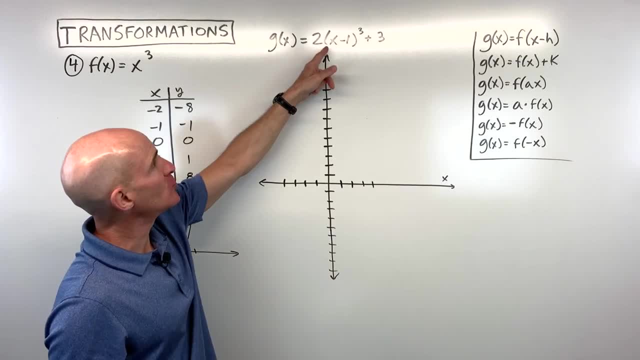 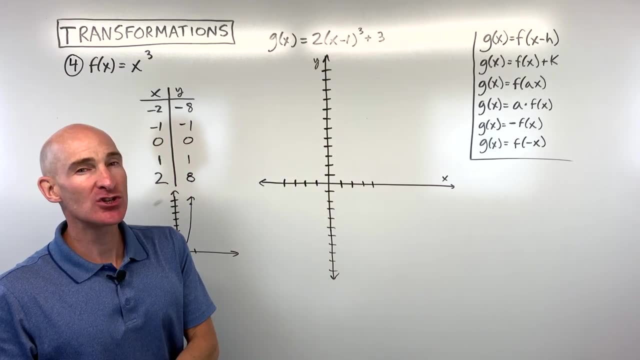 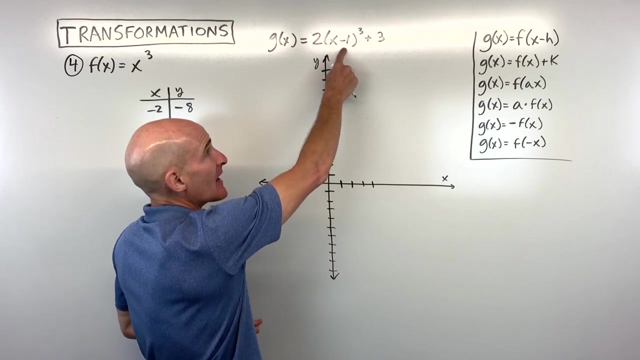 happens here for this g of x function 2 times the quantity x minus 1, cubed plus 3.. So just take a moment now. What do you think is the first thing we should do? What's the first transformation? Well, I like to work from the inside out. So the x minus 1, I would say let's do this part first. 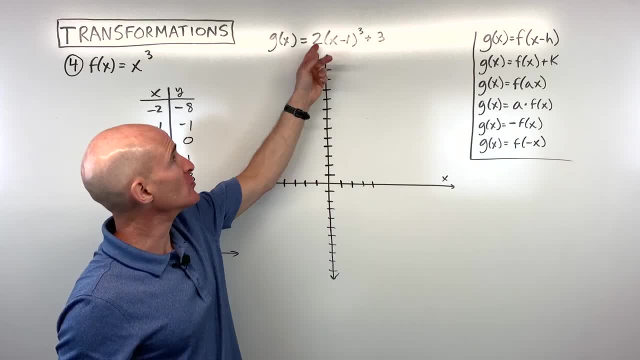 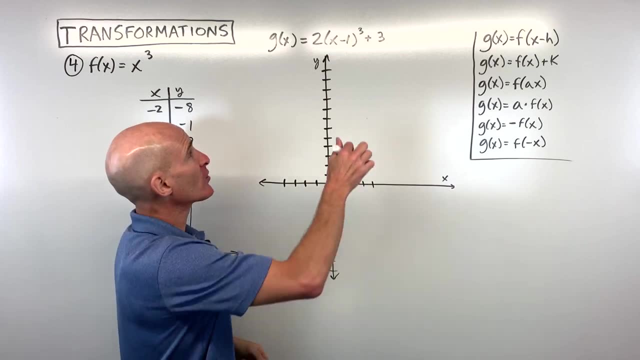 Now in this problem, it won't really matter in our final result if we do this 2 first and then this 1.. But you want to make sure you do this 3 here at the very end. But I again like to work from the inside out. So this x minus 1, let's go through the different steps. 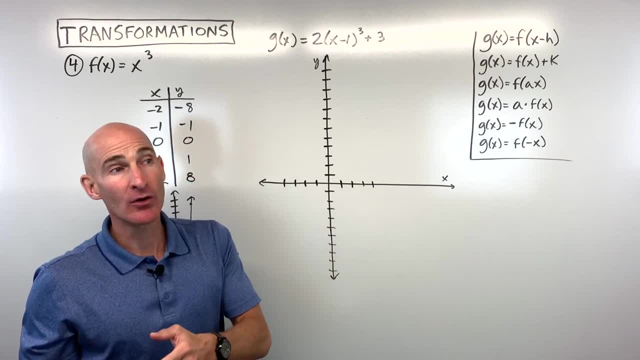 So we say to ourselves: is it group with the x or not group with the x? Well, it's in the parentheses. So that means it's a group with the x, which means it's going to affect the x values or the horizontal direction. 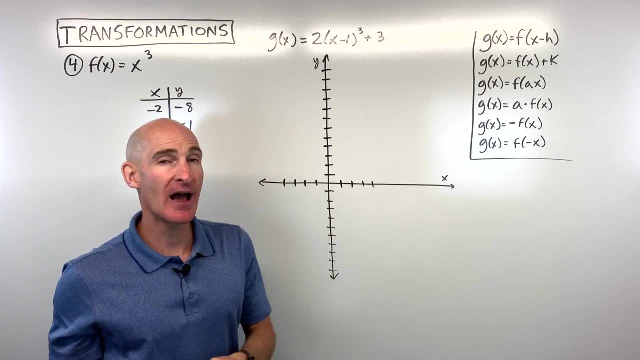 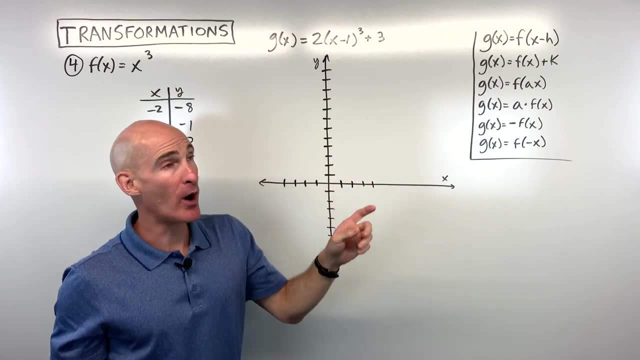 But remember, when it's grouped with the x, does it have the same effect or the opposite effect, Opposite effect. So the minus 1 is actually going to go positive 1.. Okay, so it's going to go to the right one. And remember, if you're adding or subtracting, we say it's a shift. 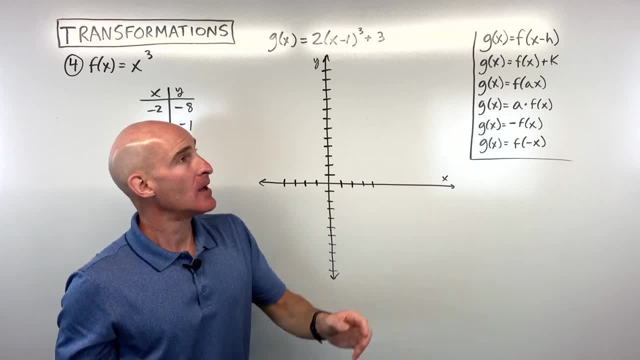 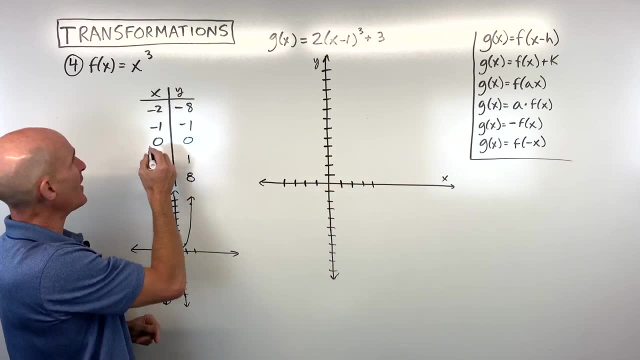 If it's multiplying or dividing, it's going to be like a stretch or a shrink. In this case you can see we're adding or subtracting, so it's a shift, So it's going to go right. 1, which means that we're going to add 1 to all these x values, right? 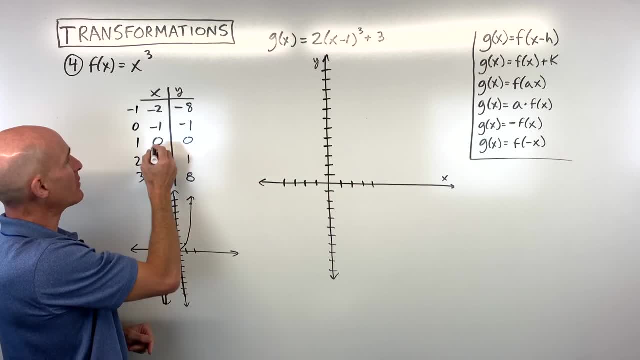 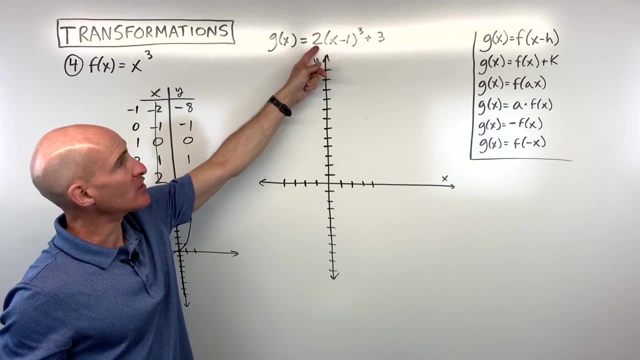 So negative: 1,, 0,, 1,, 2, and 3.. Let's cross out the old x values Now. let's work from the again inside out. The 2 is a little bit further away here, The 2,. 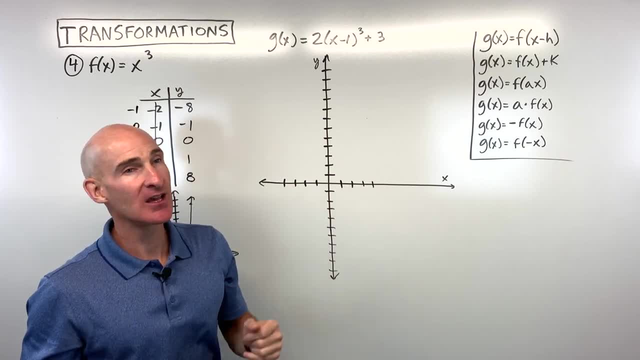 let's go through the steps. Is it group with the x or not group with the x? Well, it's not in the parentheses, so I would say it's not group with the x, which means when it's not group with the x. 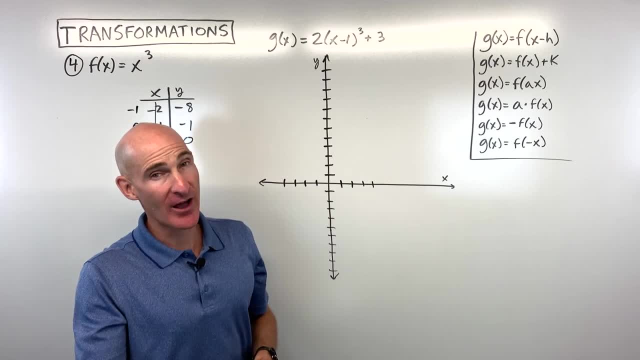 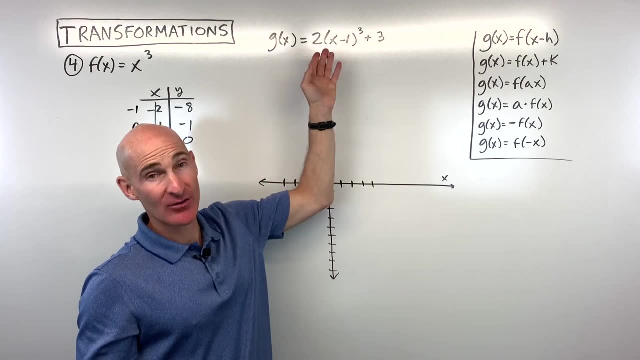 it affects which one, The x or the y, The y values, right. And when it's not group with the y, it has the same effect. When it's not group with the x, it has the same effect. right, It's affecting the y's. And one other thing: we're multiplying. See how it's right next to this, It's multiplying. 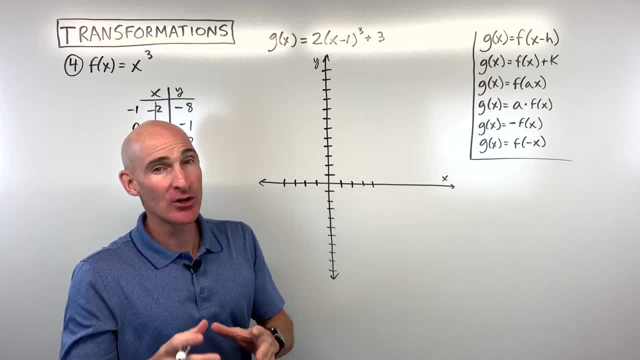 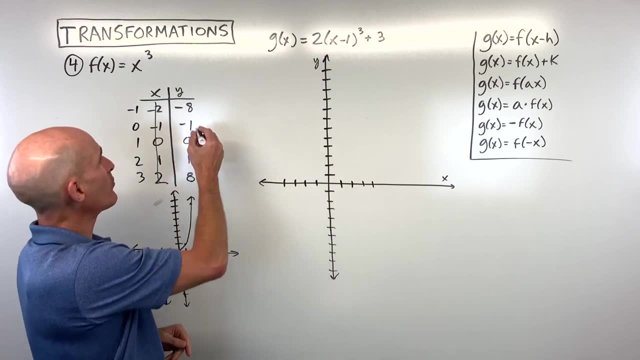 So when we multiply or divide, we're thinking stretch or shrink. So putting all that together, this is going to be multiplying the y values by 2. That's a vertical stretch by a factor of 2. In our table, we're going to multiply all these y values by 2.. 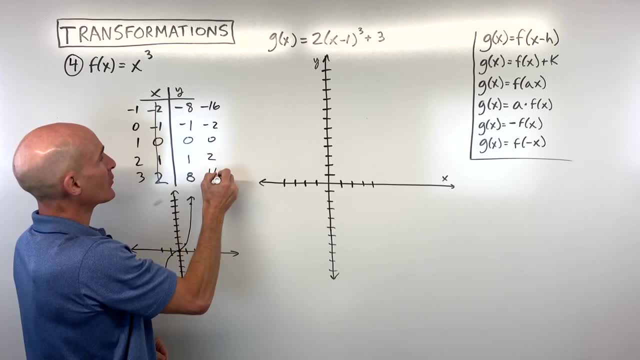 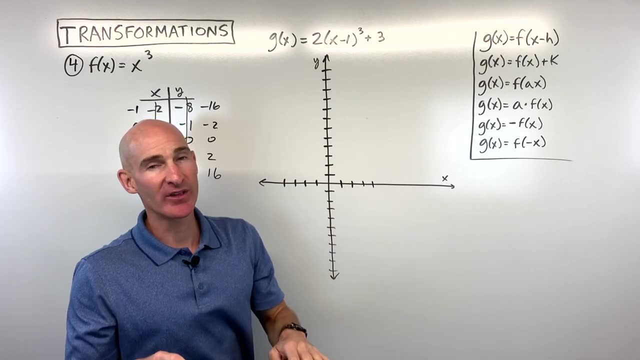 So let's do that and cross out the old y values. Lastly, last step, the plus 3, is it group with the x or not group with the x? Well, it's not in the parentheses, so I'd say it's not group with the x. Does it affect the x or the y values? 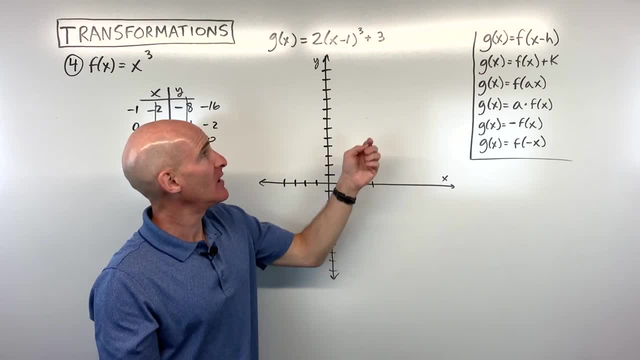 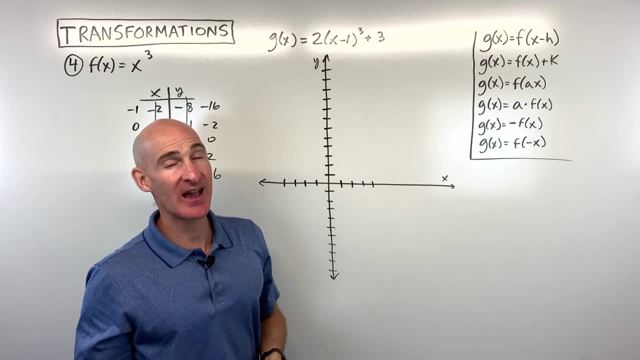 Well, if it's not group with the x, it's affecting the y values. okay, which means it has the same effect or the opposite effect. Well, if it's the y's, it has the same effect. If it's acting on the x's- remember we said, it has the opposite effect. 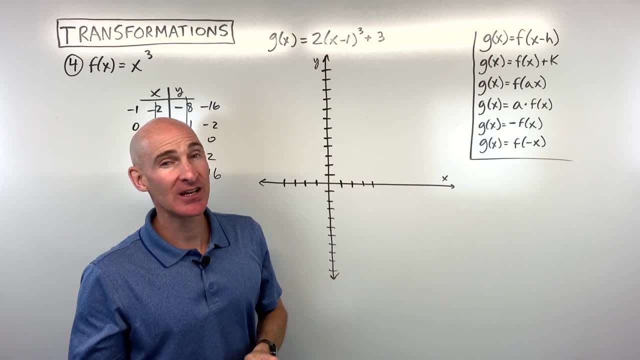 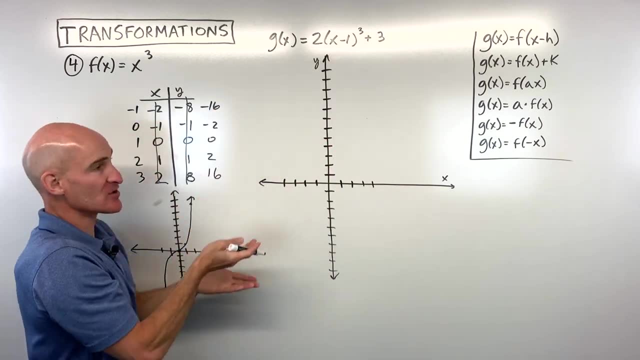 So this is going to have the same effect. And adding or subtracting is a shift, So this is going to be shifting positive 3 up 3, which means that we're going to be adding 3 to our y values, because the y controls the vertical direction. 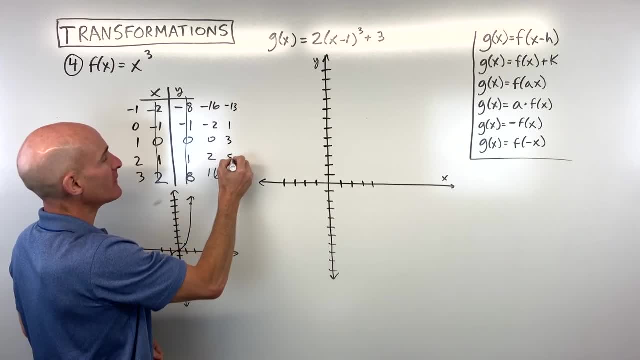 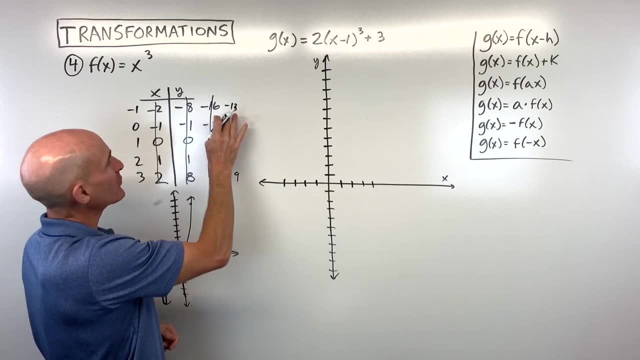 So that means this is going to be negative 13,. 1,, 3,, 5, 19.. Let's cross out those old y values Now. we have our coordinates here that we can plot right. So negative 1, negative 13 might be a little bit off my graph here. Let's start with 0, 1.. So 0, 1 would be right about here. 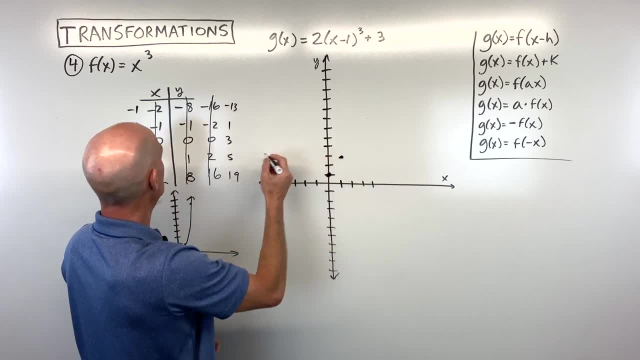 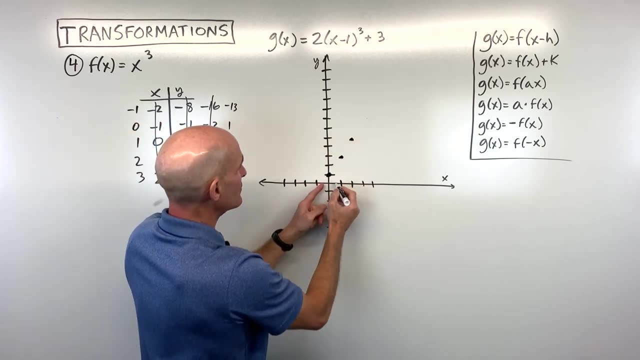 1, 3 is going to be right about here. 2, 5 is going to be right about here. 3, 19 is going to be where 1,, 2,, 3, up, way up here. 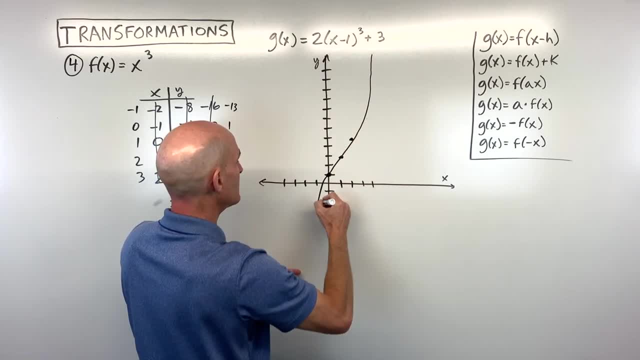 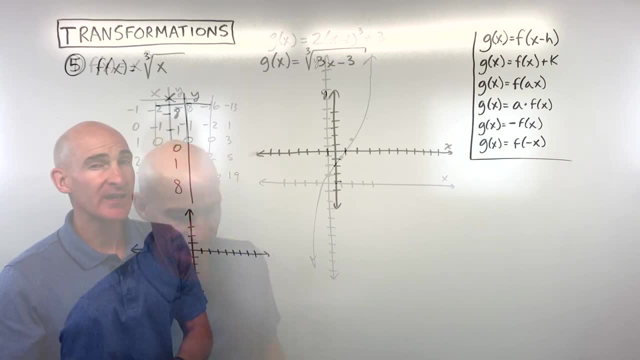 So you can see, this graph is basically going like this And you've got a good sketch of your graph. So let's take a look at another example. Okay, let's look at example number 5 here, which is: f of x equals the cube root of x. 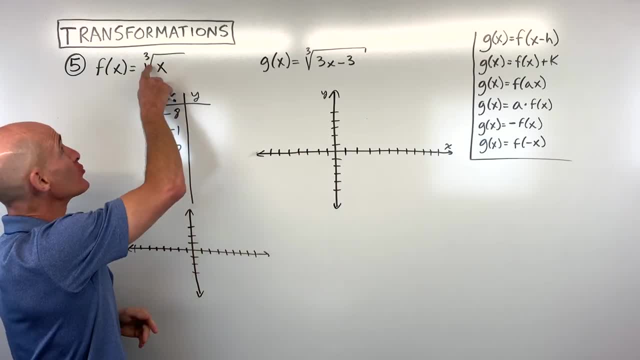 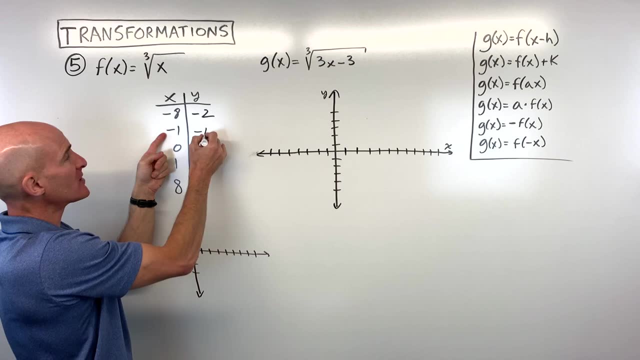 The last problem we were doing was x cubed. This is the cube root of x. So what number times itself 3 times is negative 8? That's going to be negative 2.. The cube root of negative 1 is negative 1.. Cube root of 0 is 0.. Cube root of 1 is 1.. 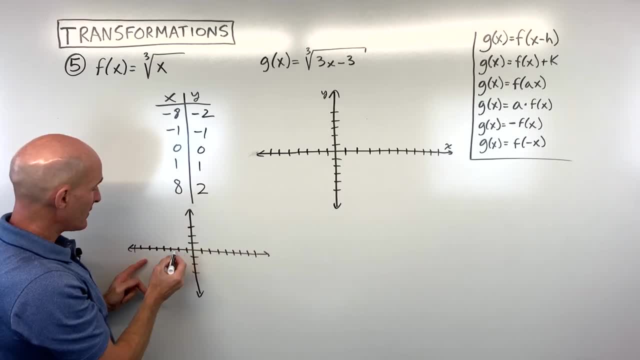 And cube root of 8 is 2.. If we plot this graph, let's see we've got left 8 down 2, which is right about here. Left 1 down 1, 0, 0, 1, 1, 8, 2.. 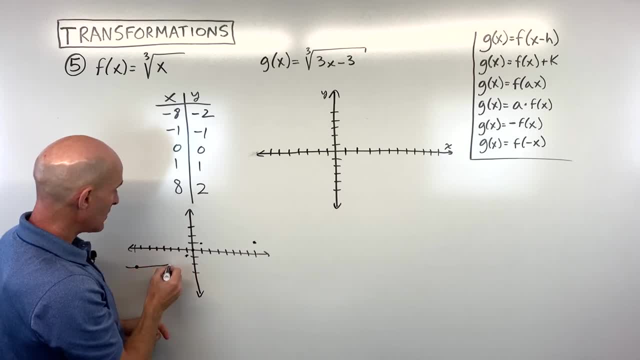 Now sometimes students say: well, do we have to memorize these coordinates or these points? Well, you know you don't have to. You can always go ahead and recreate the table, But what you'll find after a while is that you know you'll end up memorizing them. 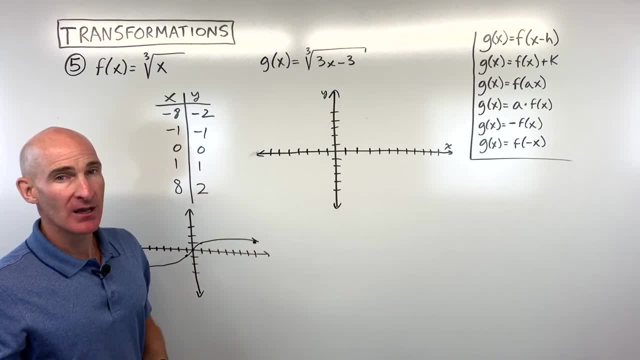 And it's good to kind of know some of the basic ones so you don't have to kind of recreate the wheel you know each time. You can basically just you know, know your key points and you have a starting place. But again, you can always just make a table and start there. 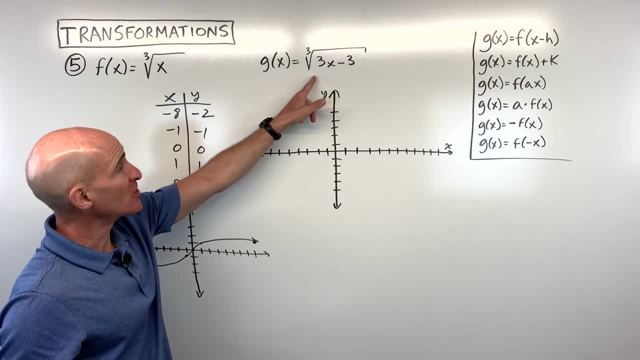 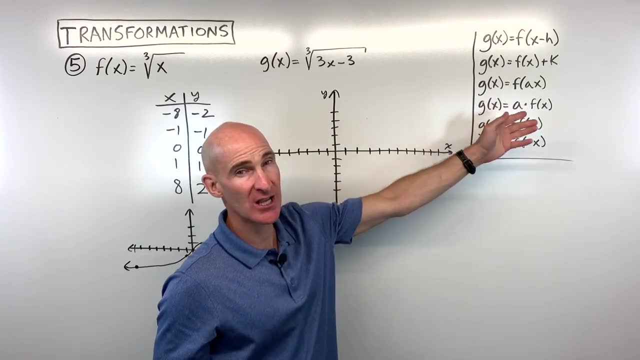 Now we're going to look at this function. g of x equals the cube root of 3x minus 3.. And this is a little bit more challenging of a problem And that's where we're going to start. We're going to start diving into this function notation a little bit. 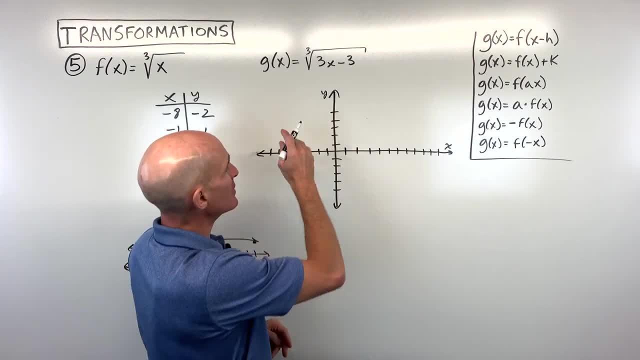 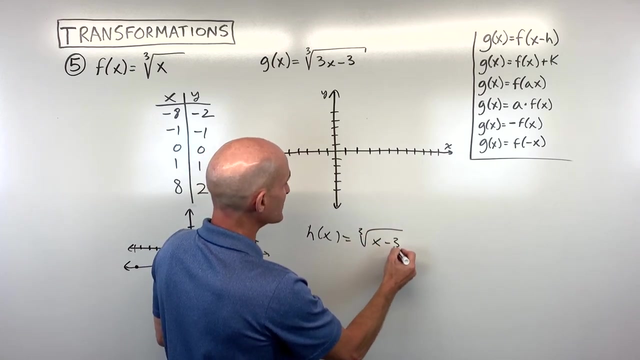 So I want to kind of show you something here. first, Let's imagine if we had a little different function, Say if our function was like this. Say if it was h of x equals, let's say, the cube root of x minus 3.. 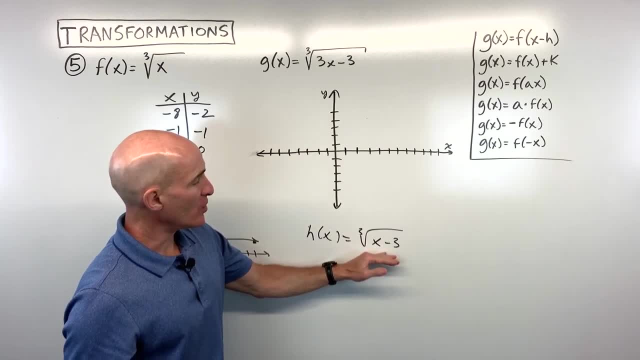 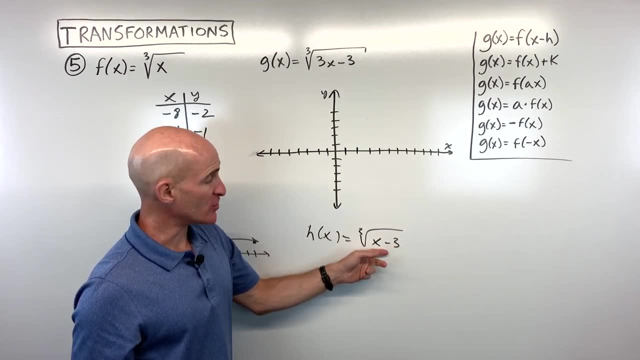 Okay. so if we look at this function, right here, there's only really one transformation, right? You say, well, this minus 3.. What is that doing to the graph? Well, remember, it's grouped with the x, so it's affecting the x values. 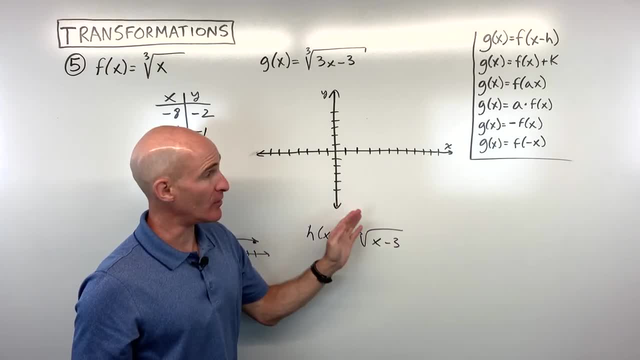 It has the opposite effect, which means that it's going to be going not minus 3, but positive 3.. And, of course, adding and subtracting, we know, is a shift right. Multiplying, dividing is a stretch. So this is going to be going right 3,, shifting right 3.. 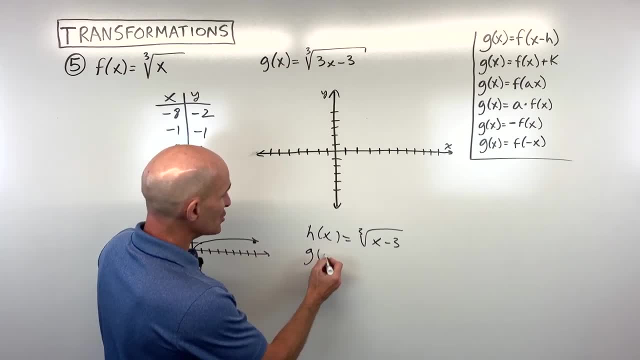 But then let's say, for example, if we have now this function, notation g of x is equal to h of 3x. Now the wave function. So the wave function's work is that whatever's in the parentheses right here, it goes in for x on the right right. 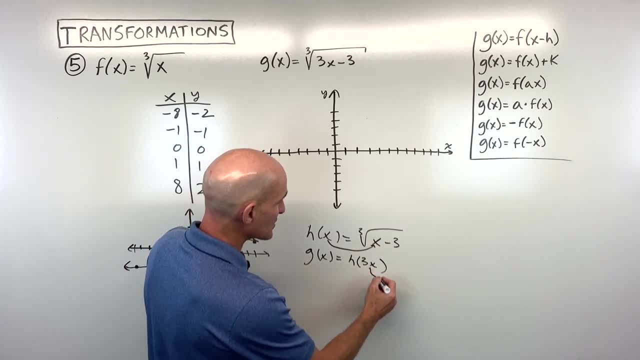 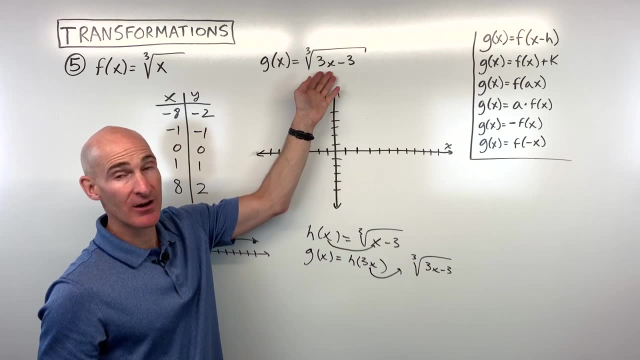 So that means what I'm doing is: I'm going to take this 3x here, I'm going to put it in for x. So if I do that, this is going to look like this: The cube root of 3x minus 3, which is what we're working with right here, right. 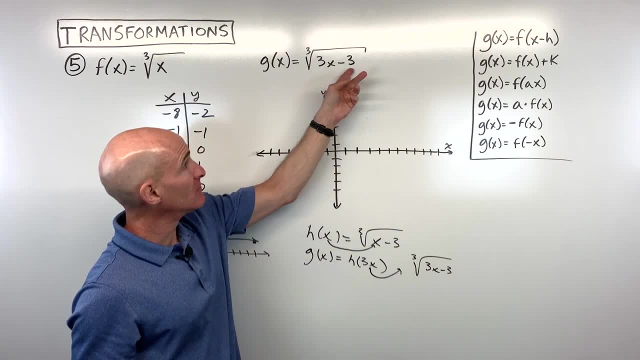 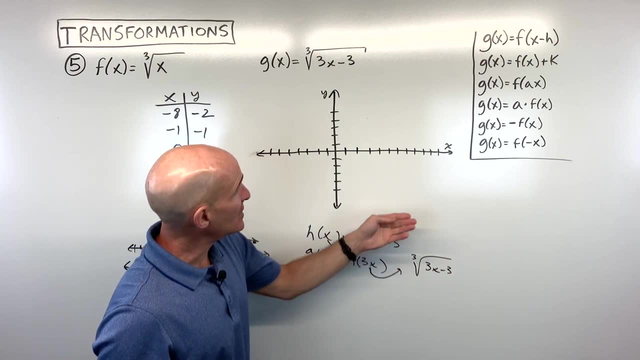 But what happened first? Was it the shifting right 3 or this 3 here? Like? what does this 3 do? Well, we know. See this notation h of 3x. This is this function notation right here, Notice the a is grouped with the x, which means it affects the x values. 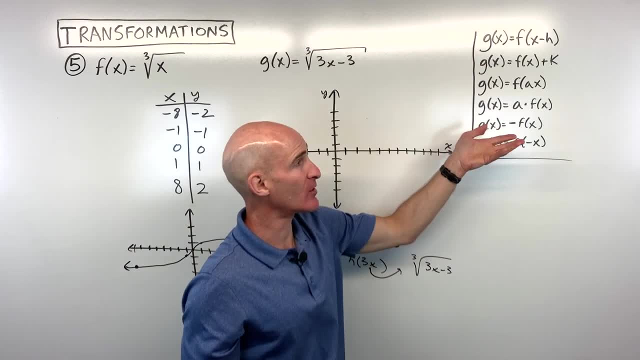 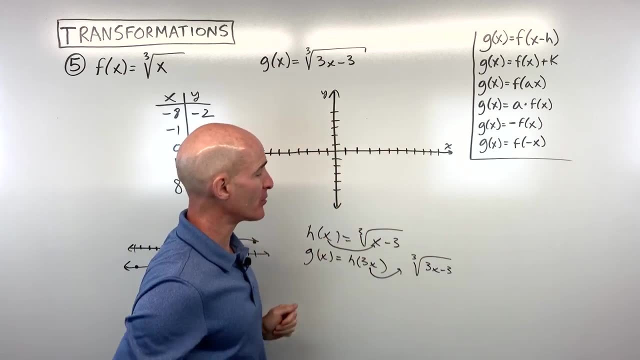 Has the opposite effect, which means we're not really multiplying the x's by 3.. We're multiplying by the reciprocal 1- 3rd, which is going to be a horizontal shrink. Okay, dividing the x's by 3 or multiplying by 1- 3rd. 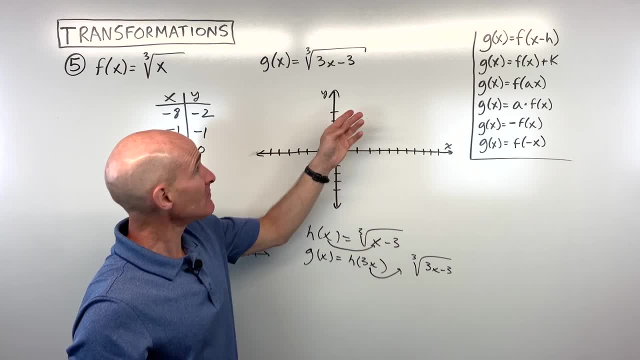 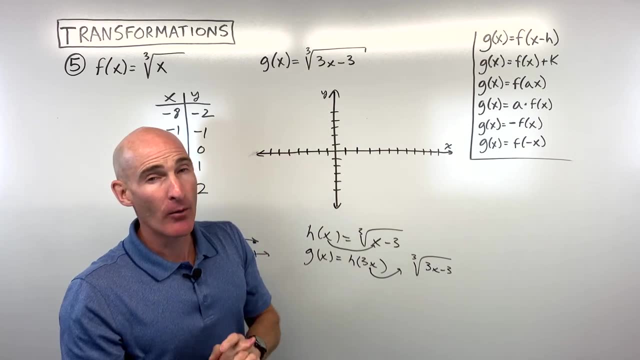 It's the same thing, But what happened? first We actually went right 3, and then we did a horizontal shrink by a factor of 1- 3rd. Now this is where we need to. We need to kind of talk a little bit, because you know how, I said, I work from the inside out. 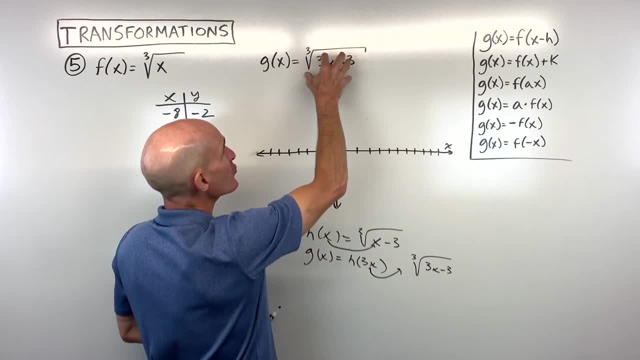 Well, the inside to me in this problem is like what's underneath this cube root? Like if I had a plus 7 over here that would come at the very end, Or if I had maybe a 2 in front. I like to work from the inside here. 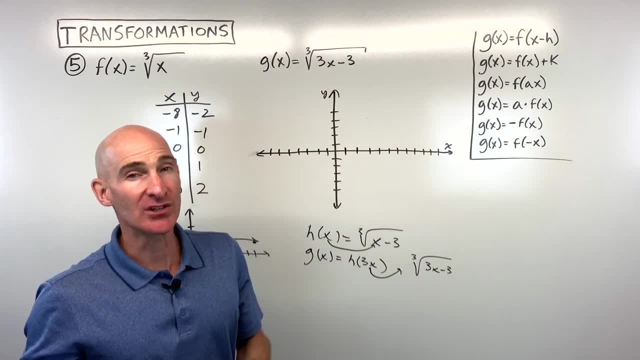 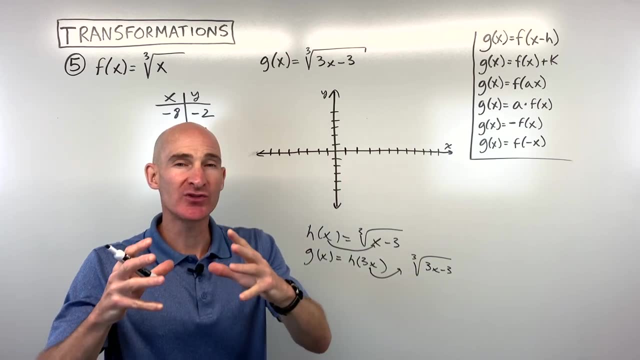 So, but when there's more than one operation- okay, grouped with the x, like that- you want to think about how to build up that function, Kind of like you know those Russian dolls where there's like a doll inside of a doll inside of a doll. 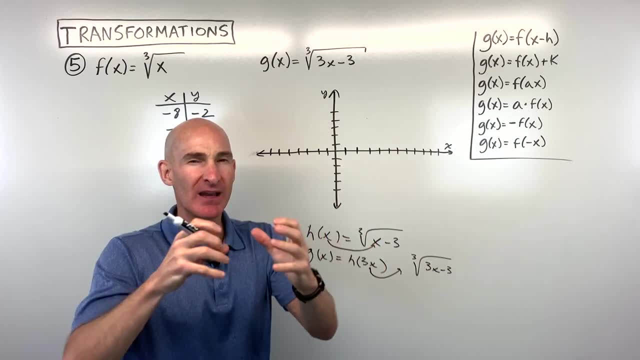 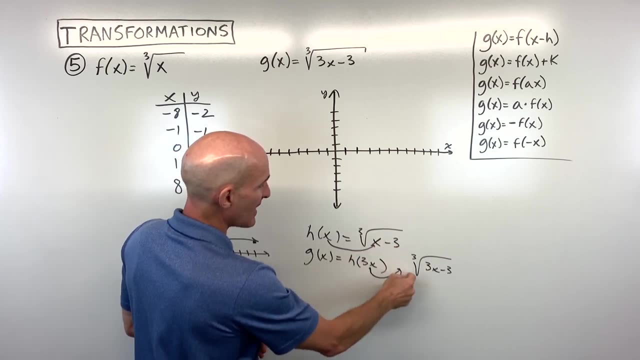 So you kind of have to say, well, what's my outer function, Or what's my inner function, right? In this case, the outer function was this: right here, this x minus 3.. And then what do we do? We replace this x with this 3x. 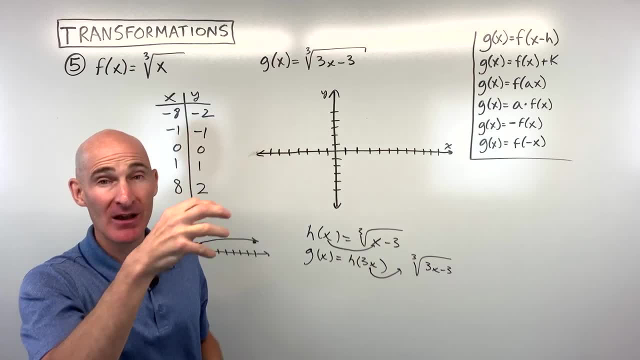 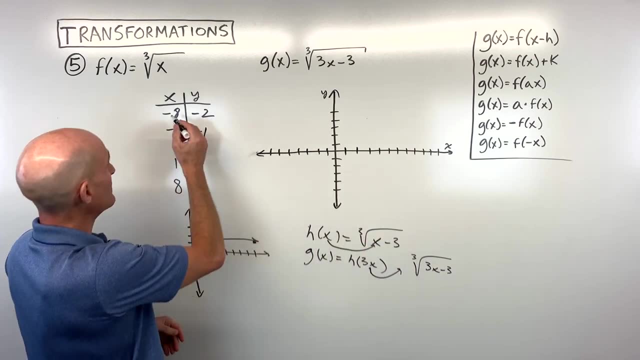 That's kind of the inner Russian doll, the inner one, the one on the inside. That came after that came second right. So here what we're going to do is we said we were shifting right 3, which means I'm going to add 3 to the x values. 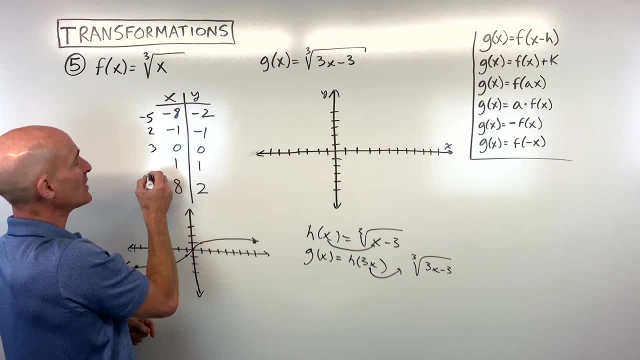 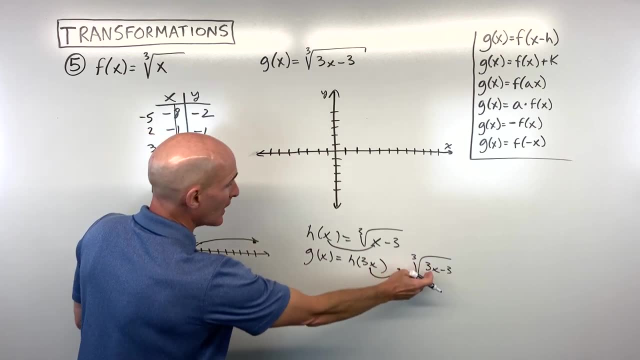 So that's going to be negative: 5,, 2,, 3,, 4,, 11,, right? So let's cross out those old x values. Then we said that we're doing a horizontal shrink by a factor of 1- 3rd, 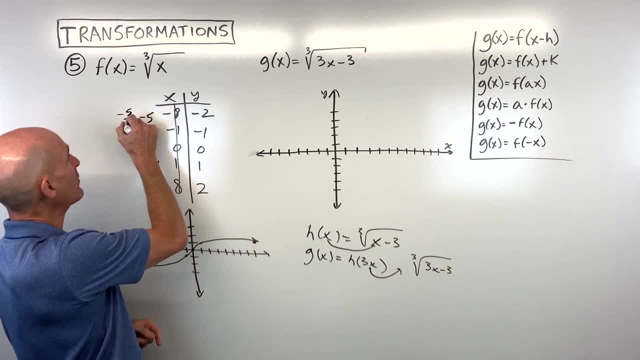 which is going to multiply all these x values by 1- 3rd. So now we have negative: 5 3rds, 2 3rds, 1,, 4 3rds, 11 3rds. 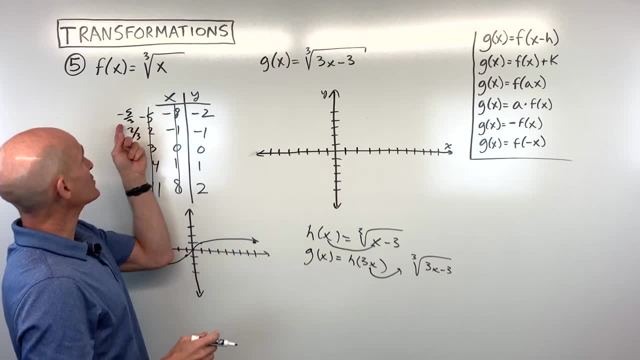 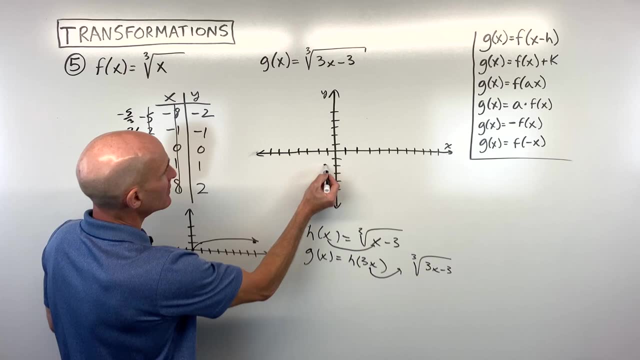 Let's cross out those old x values. Now let's see if we can graph this So: negative 5 3rds, that's like negative 1 and 2 3rds, Negative 2, which is right about here. 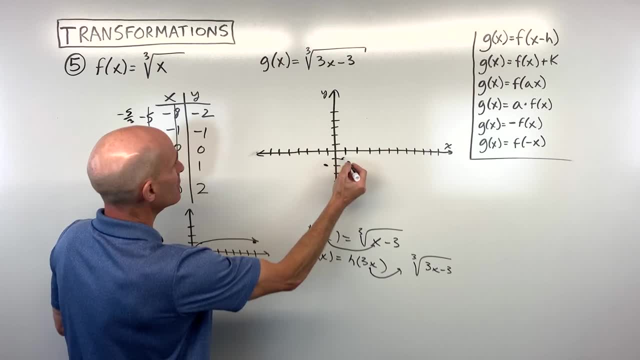 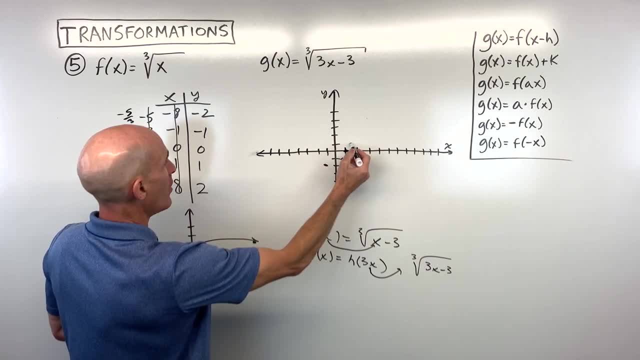 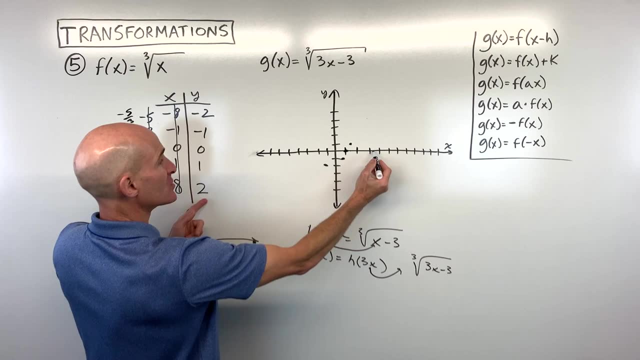 Four thirds, which is like 1 and 1, 3rd up 1 right here, And 11 3rds, which is 3 and 2, 3rds: 1,, 2,, 3,, almost 4, 3, up 2,. 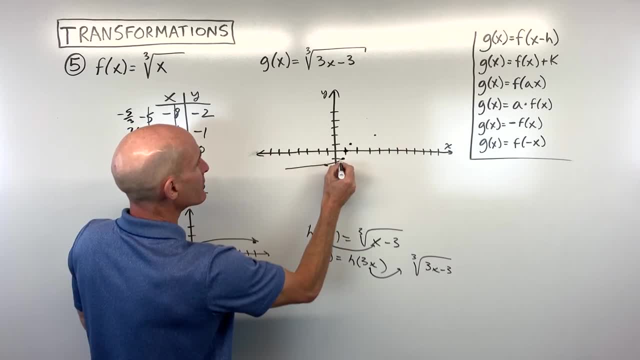 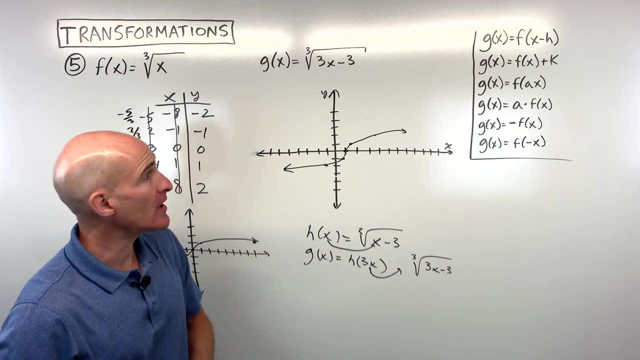 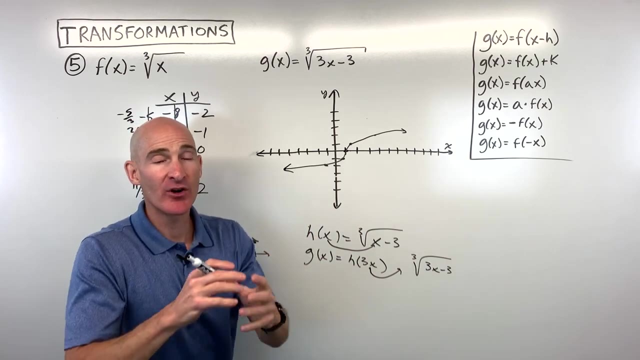 is going to be right about here. So there's our graph, something like that, And you got it. So this one was a little bit more challenging because we had more than one thing going on here. So we want to think from that nested Russian doll scenario. 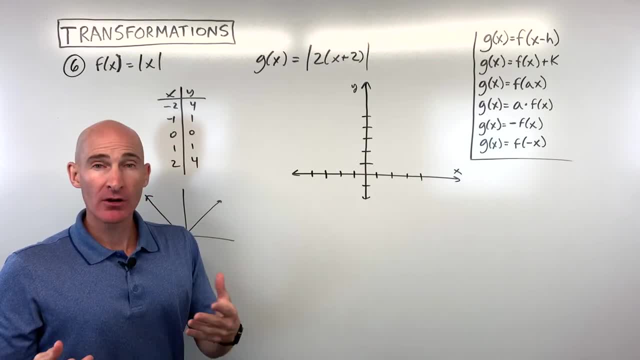 Let's look at another example. OK, now, depending on your class and what you're learning and what level you're at, you might only need to know what we talked about in examples 1 through 4.. And example 5, we got a little bit more challenging. 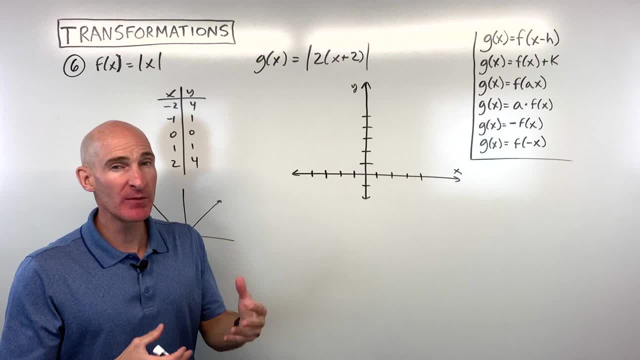 We're going to do some other types of problems as we go through, So you might want to stick with me to learn a little bit some more techniques that you'll be using in the future, Or your class might actually be involved with this right now. 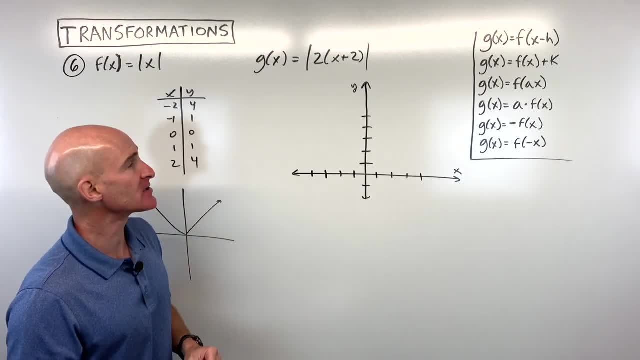 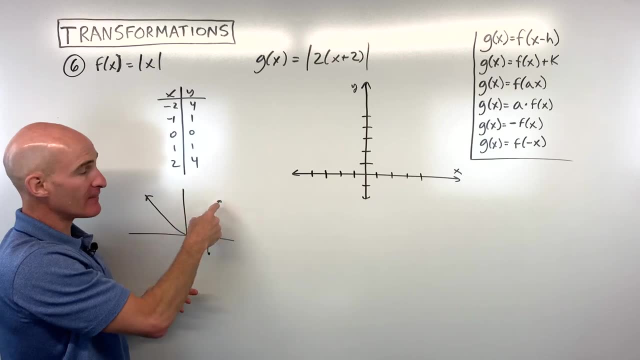 if you're taking like a pre-calculus class or college algebra type class, OK. But let's look at number 6 now. We've already talked about the absolute value graph. We know what our table looks like. We know we have that v-shaped graph. 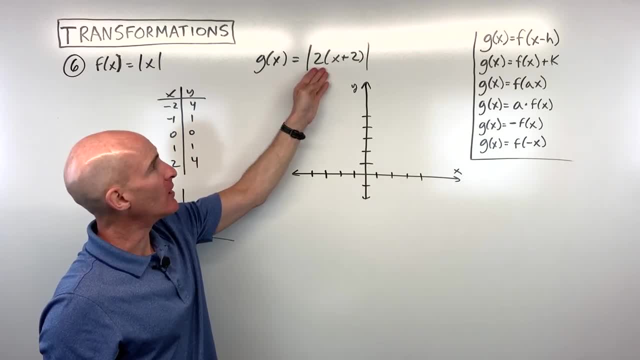 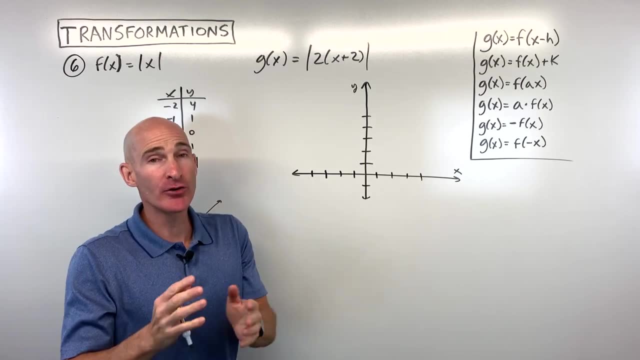 But we want to graph this: one g of x equals the absolute value of 2 times the quantity x plus 2 inside of that absolute value. Now, depending on what level you're at in your learning of transformations, your teacher might say: why don't you just rewrite this? 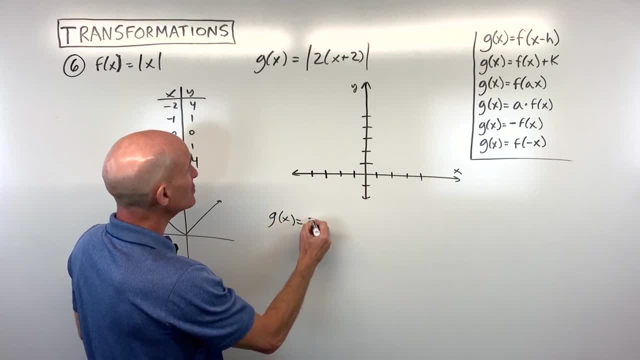 Why don't you just say g of x is equal to the absolute value of 2 times x plus 2? And then the absolute value of 2 is just 2.. And then, see, we've kind of rewrote it, rewritten it in a little bit simpler form. 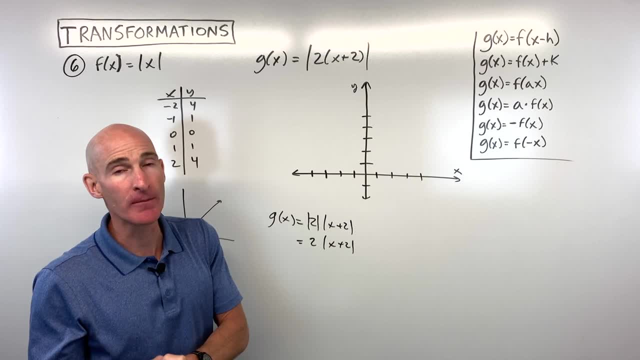 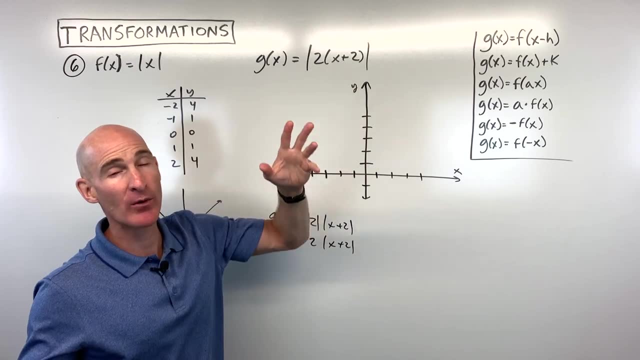 So now you can kind of think about it from this perspective And that might be a lot easier. But your teacher might want you to describe the order of transformations as the function, as given right here. So what I would ask in this problem is: what do you think you would do first? 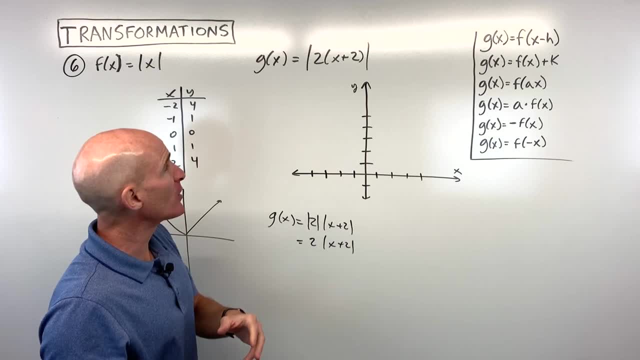 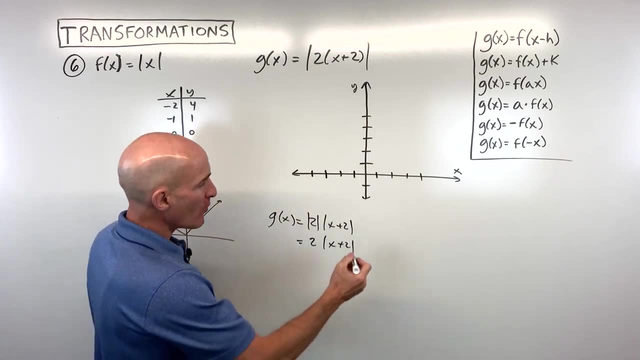 And what do you think you would do? second: Well, another way to look at it is like: what's the innermost function, What's the outermost function And when you're building up this function here, what you might want to think about. 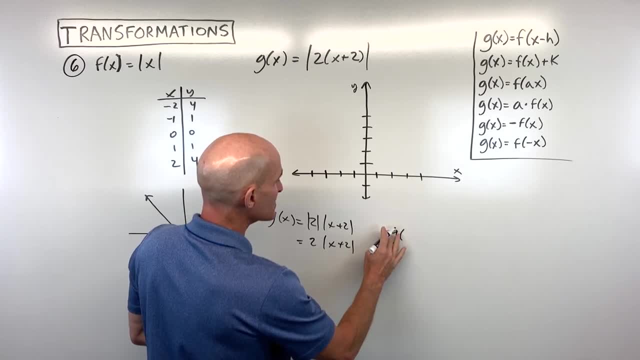 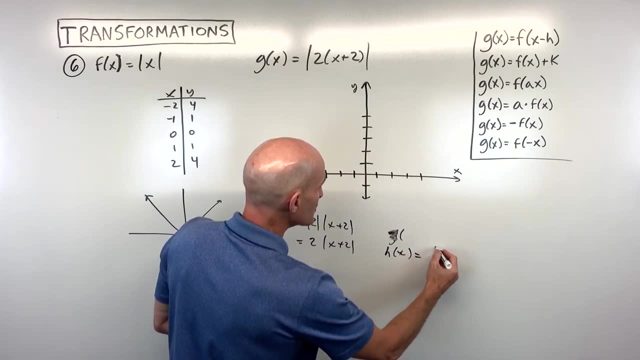 is OK if I had another function. let's just call this: instead of g of x, let's call this h of x. So we'll say h of x is equal to, let's just say it's 2x. 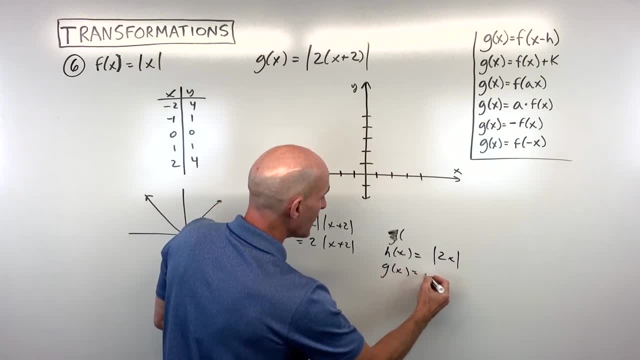 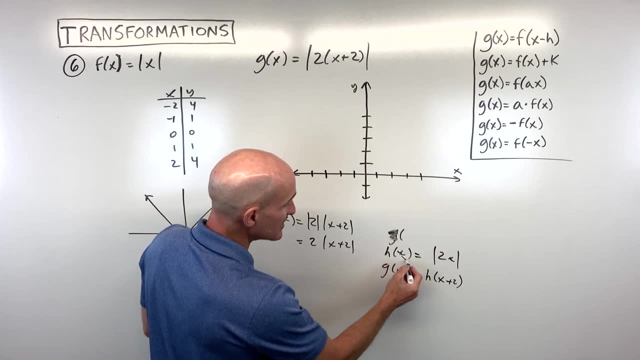 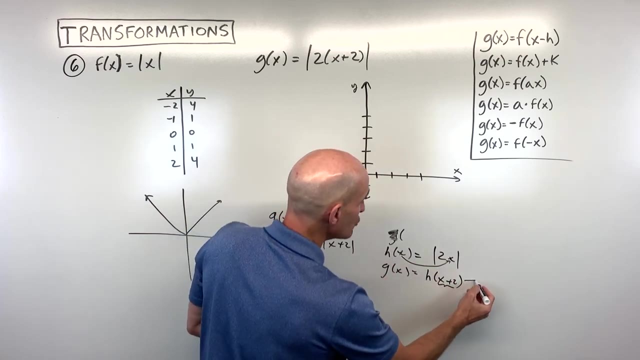 And then we'll say: g of x is equal to h of x plus 2.. Now remember, whatever is in the parentheses is going to go in for x on the right. So what that means is that we're going to be replacing x with this quantity, x plus 2, which 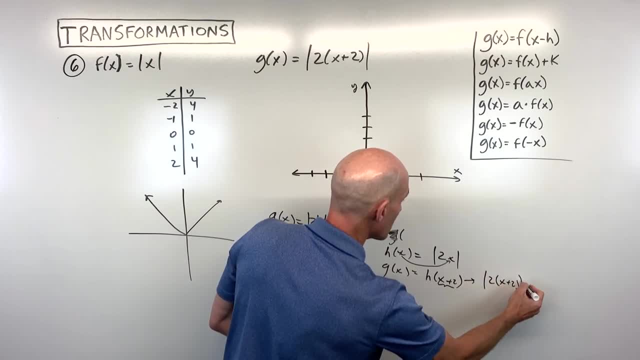 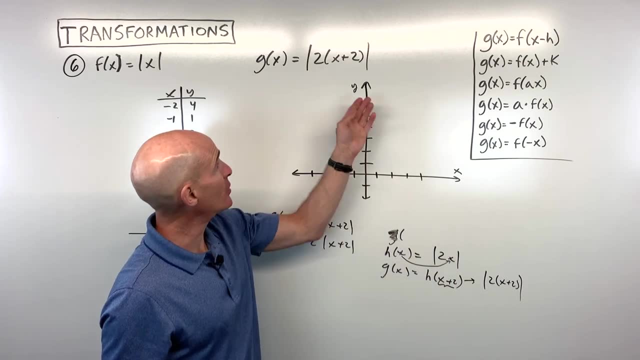 is going to give us this function that we have right here, right? So what happened first? Well, it looks like we're actually doing the multiplication here first, OK. And then we're doing this x plus 2 second, this addition, second. 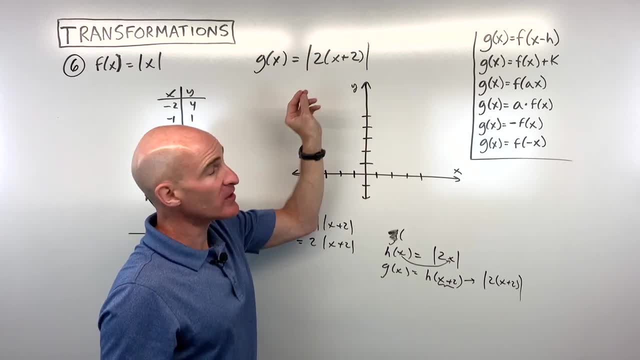 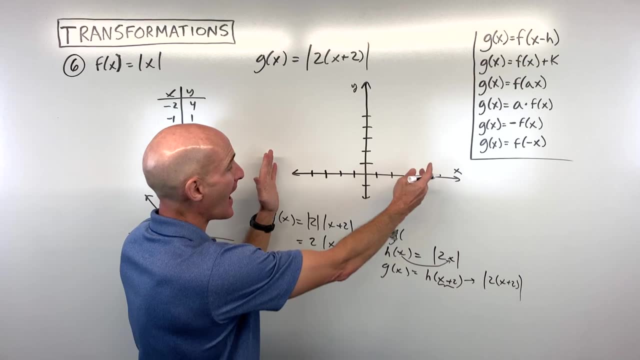 So the 2, notice it's grouped with the x, It's going to affect the x values, But when it's grouped with the x it has the opposite effect, which means we're actually going to be multiplying the x's by a half. 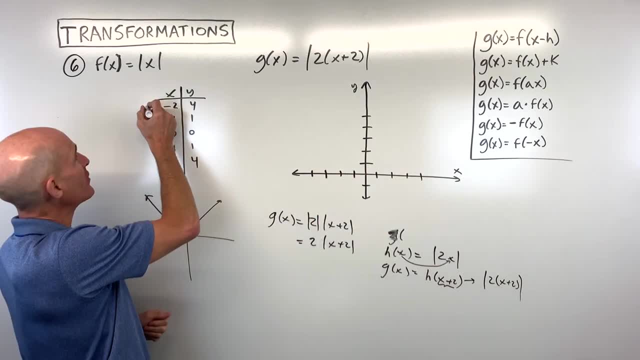 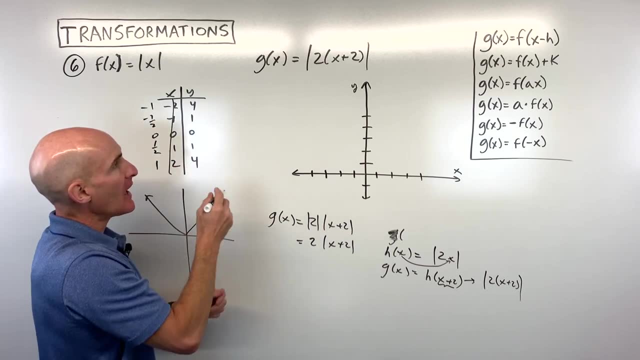 That's a horizontal shrink. I'm going to multiply all my x values in this table by a half, cross out the old ones, And then the x plus 2, it's grouped with the x. It's affecting the x values has the opposite effect. 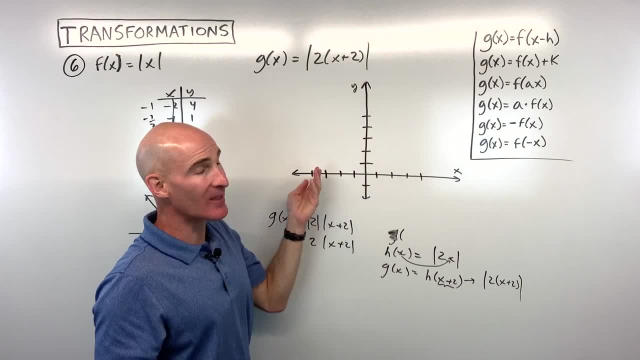 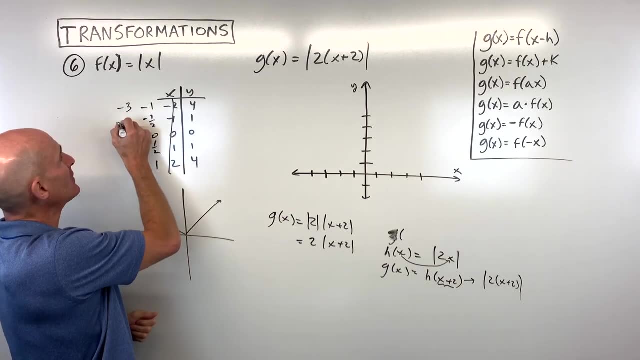 It's going to be actually going minus 2.. We're going to be shifting to the left. 2, OK, And so that means we're going to be subtracting 2 from all our x values. So that's going to make this negative 3, negative 2.5,. 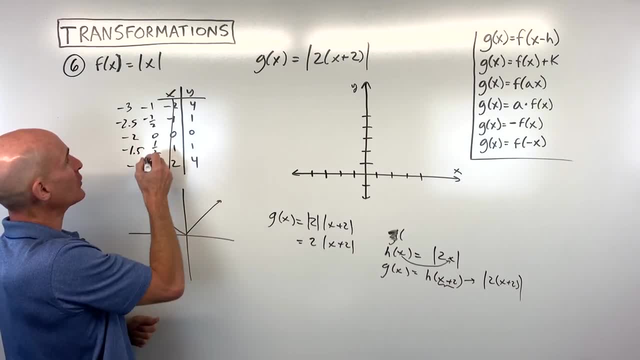 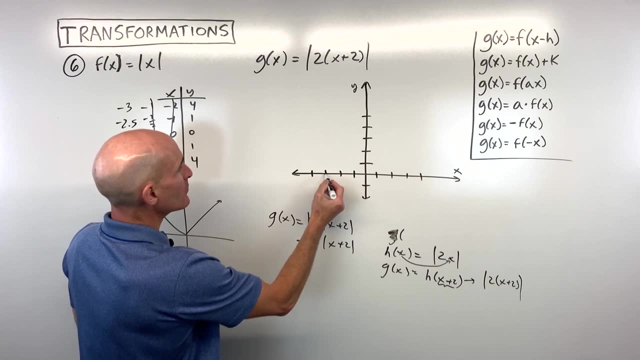 negative 2, negative 1.5, and negative 1.. Cross out those old x values. So if we plot these points now, negative 3, 4 is going to put us right about here. Negative 2 and 1.5, 1 is going to put us right about here. 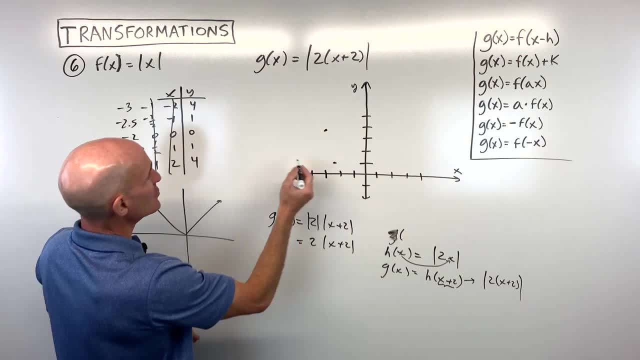 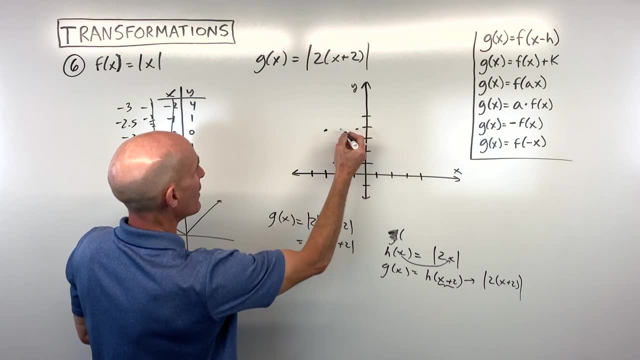 And oh, OK, That's good. And then negative 2, 0 is going to put us right here, And negative 1.5, 1 is going to put us right here, And negative 1, 4 is going to put us right about here. 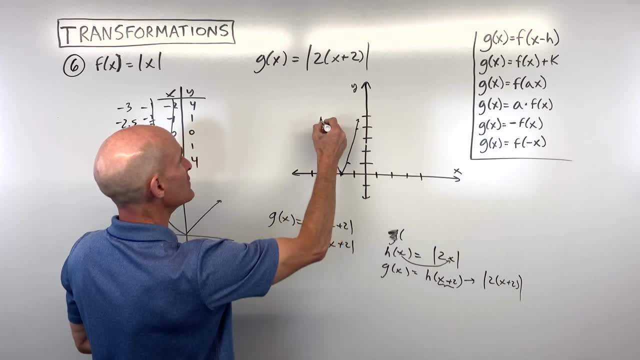 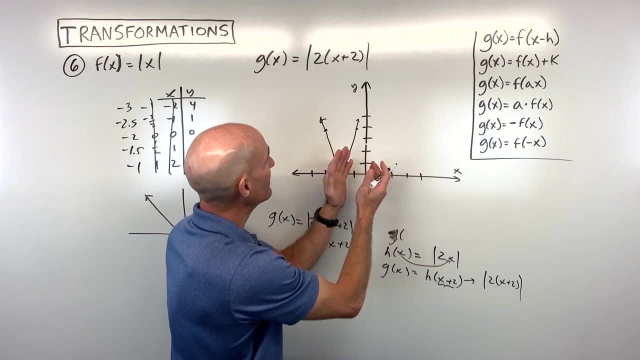 So our graph looks still that absolute value, that v-shaped graph. But look what happened. We did a horizontal shrink by 1.5, OK, And then we picked that graph up and we shifted it left 2.. So that's the idea. 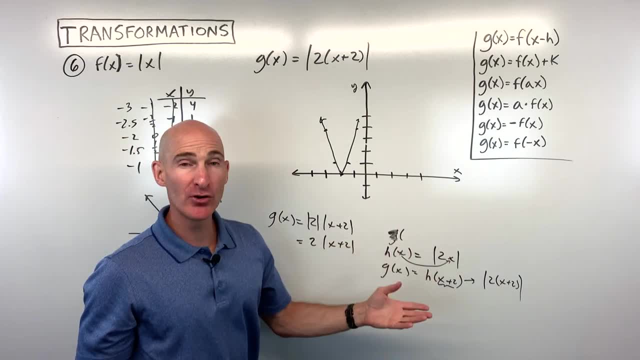 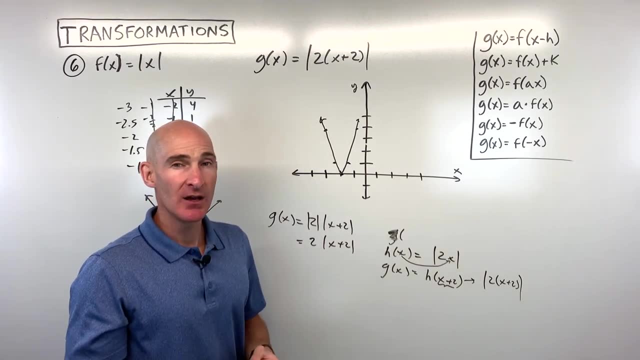 Now again, you can rewrite it or you can think about how do I build up that function, kind of like, if you're doing one step at a time, how would I create this function? Think about the nested dolls, What's the outermost function, and then 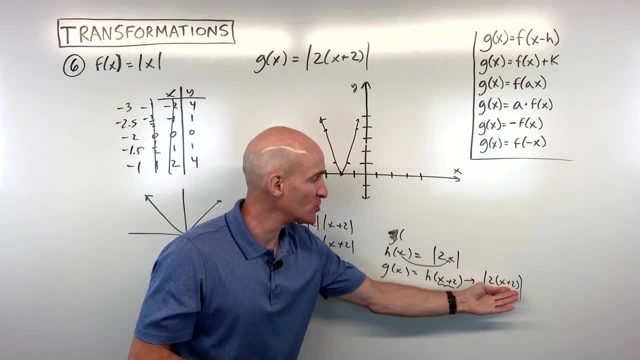 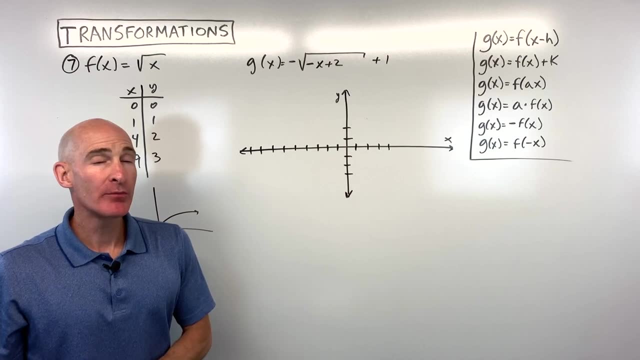 what's the innermost function. Like we're replacing this x with x plus 2. So they actually came second right. Let's take a look at another example. OK, before we do, example number 7, if you're enjoying my videos and you like the way, 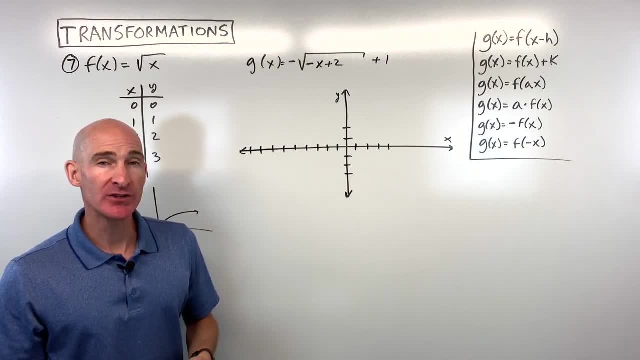 that I explain things and you want to go deeper with me into learning more about algebra 1, algebra 2, college algebra, check out my video course. it's for sale in the description below And if you just want to support the videos that I'm putting up, 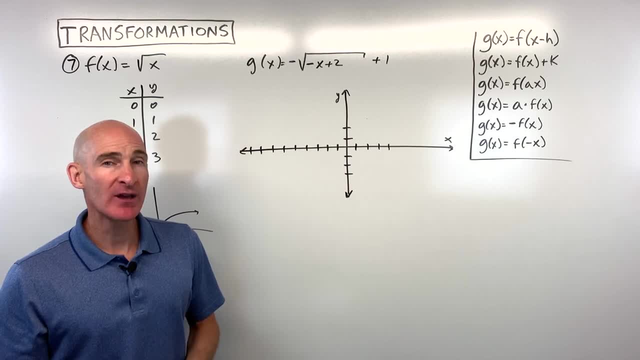 here on my Mario's Math Tutoring YouTube channel. consider supporting me as a channel member So you can join the channel as a channel member and for a few dollars a month you can support the videos I'm putting up here, And I really appreciate it. 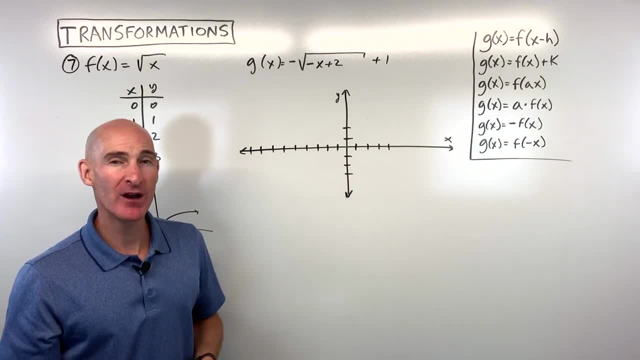 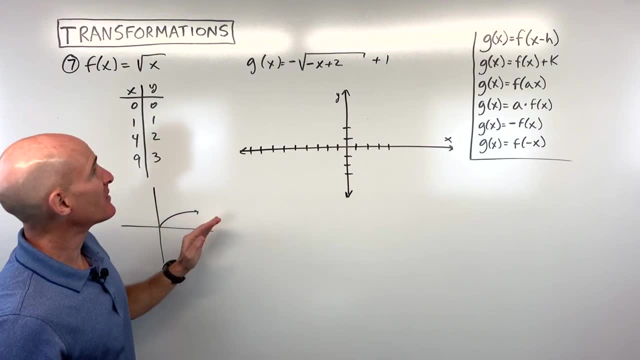 I see the members coming through and I can see who's been a member for so many months, et cetera, et cetera, And I really get a kick out of that and I really appreciate that. So I definitely appreciate that. 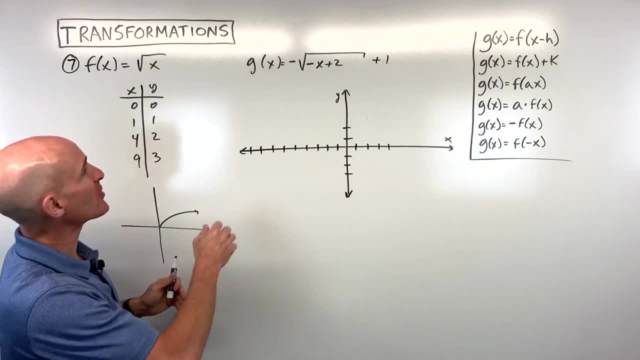 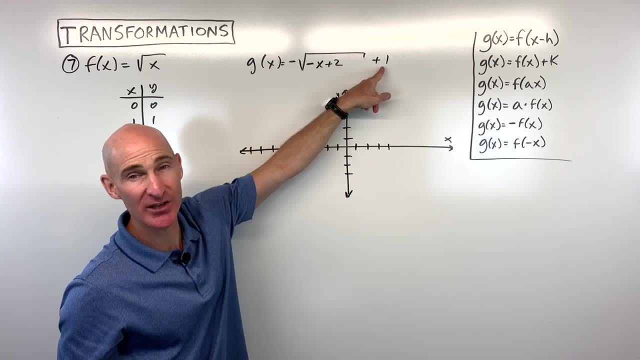 Let's see if we can. OK, Let's do number 7 now. If you want to try this problem on your own, go ahead and pause the video. Notice: we've got a negative square root of negative x plus 2 plus 1.. 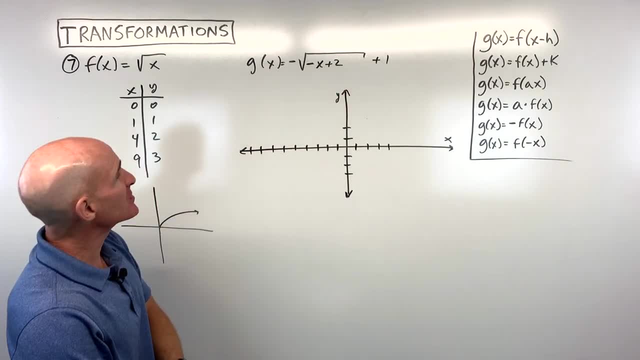 How would you do that one? Well, if I was going to do this problem, I would do like I normally do. I'd start from the inside out, But I would think about those nested dolls again. I would say to myself if I was building up this function. 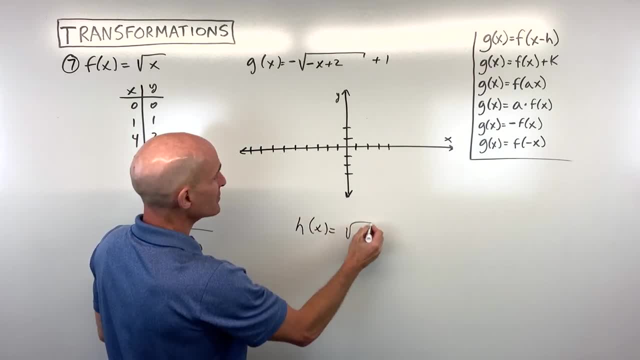 I might say like: h of x equals the square root of x plus 2.. And then I'm replacing this x, let's just say g of x with h of negative x. And remember, whatever's in the parentheses goes in for x. 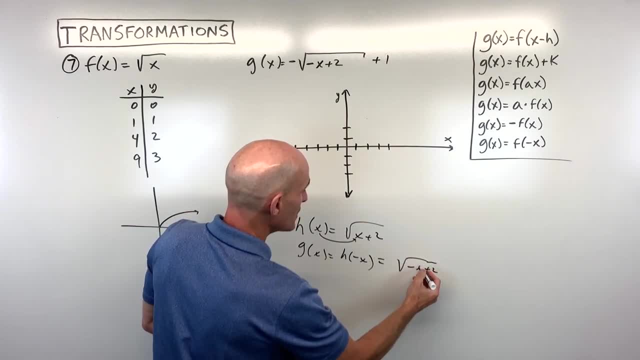 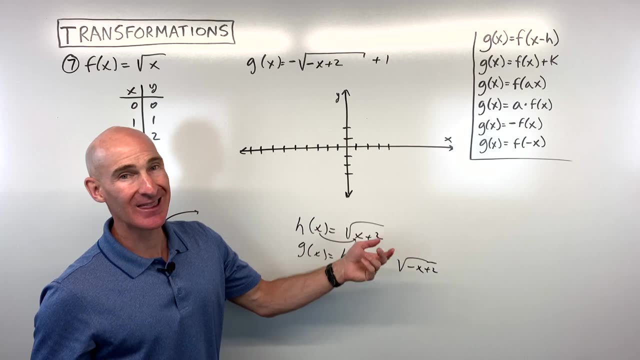 So now what we have is negative x plus 2.. So what came first? What came second? Looks like the plus 2 came first, right. So we're actually shifting left 2, which means we're going to subtract 2 from the x values. 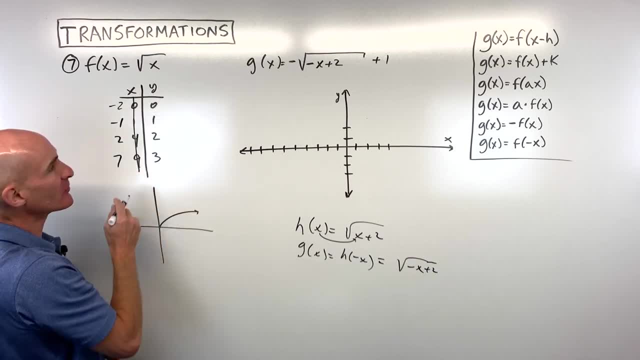 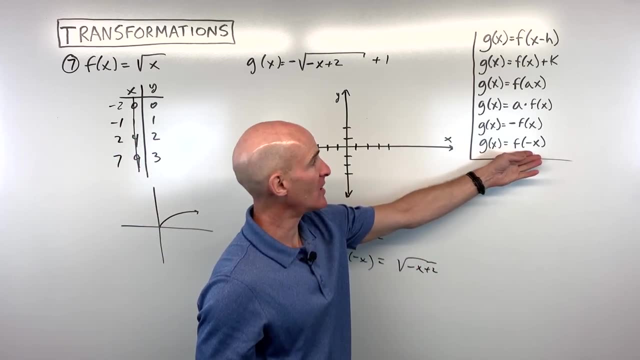 So negative 2, negative 1,, 2, and 7.. Cross out the old ones, Then we're replacing this. We're replacing this x with negative x, which is this function notation right here, When it's group of the x, remember? 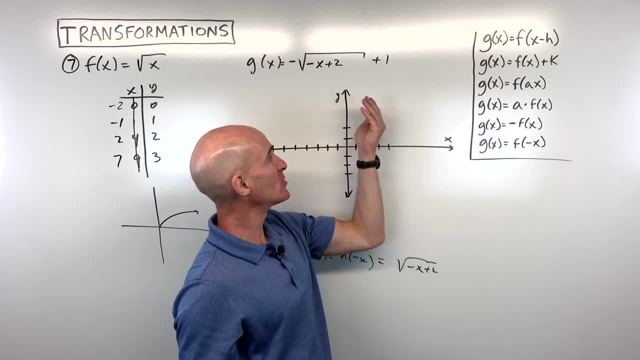 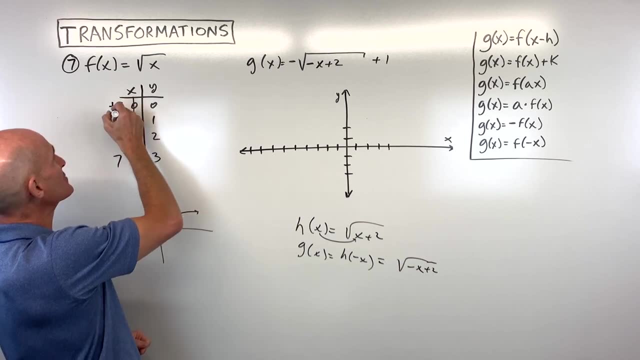 it affects the x values. It makes all the x values the opposite, which is going to reflect it over the y-axis. When you reflect over the y-axis, all these x values are the opposite sign. So this is going to become positive, positive, negative. 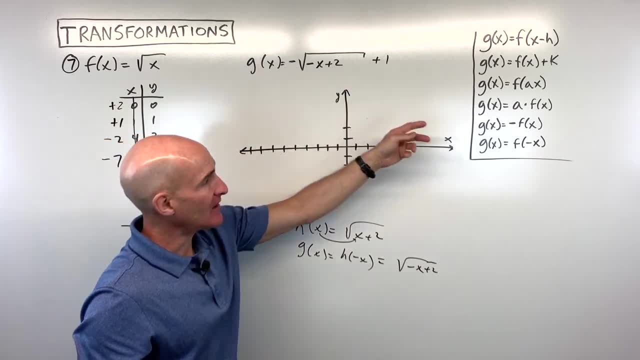 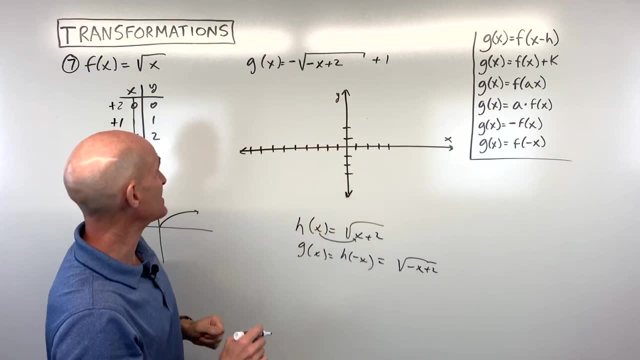 negative. This negative on the outside, that's this one right here. This is making all the y values the opposite, which is going to reflect it over the x-axis. now All the y values are the opposite. I'm going to multiply by negative 1.. 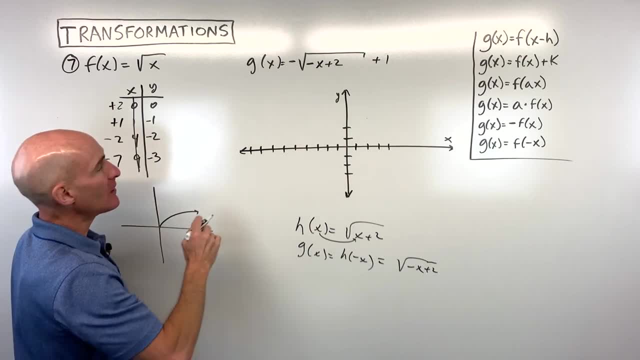 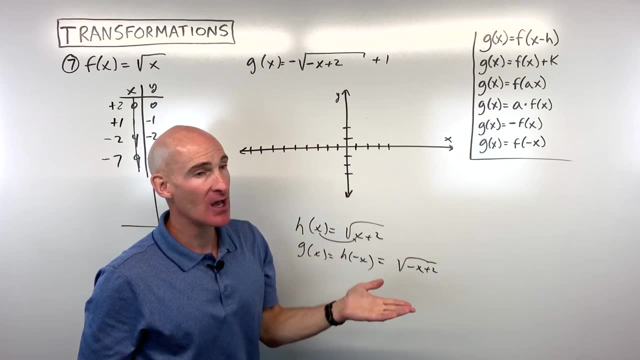 So that's going to be 0, negative 1, negative 2, negative 3.. And then, lastly, the plus 1, that's not group of the x That's going to affect the y values. It has the same effect, which means we're going to shift. 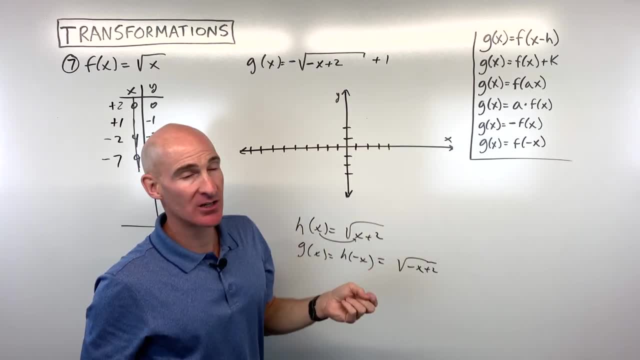 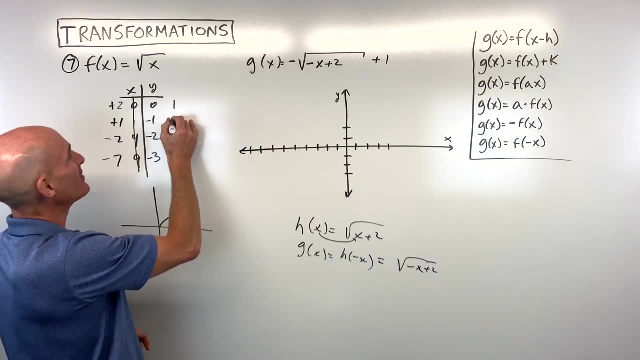 in the y direction, up 1.. Remember, adding is going to be a shift right, Meaning we're picking it up and shifting it up 1, which means we're going to add 1 to all these y values. So 1, 0, negative 1, negative 2.. 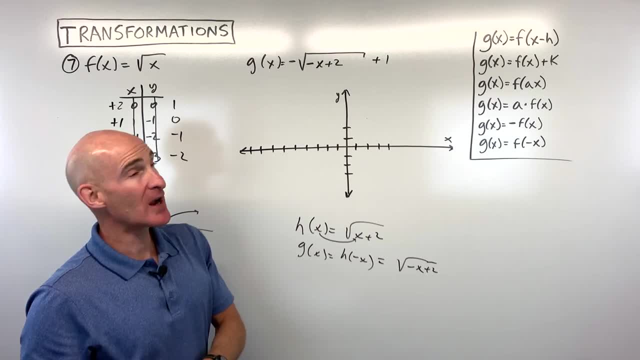 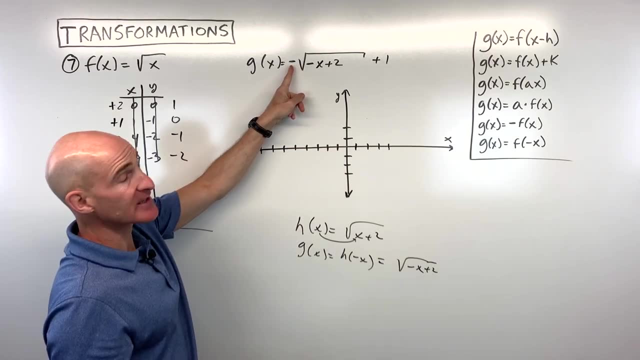 Cross out those old y values. OK, So that's the order of transformations. Now, could we have done this in another order? Sure, We could have done the reflection over the x-axis first, and then shifted left 2, and then reflected over the y-axis. 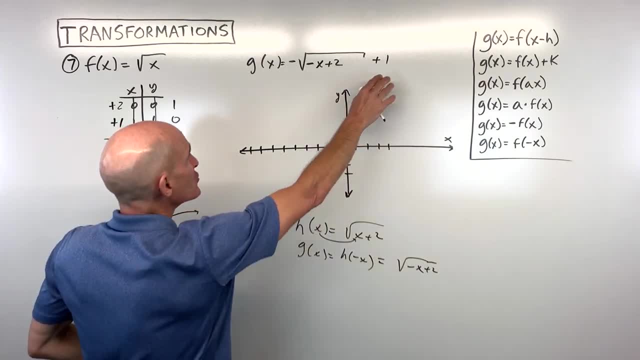 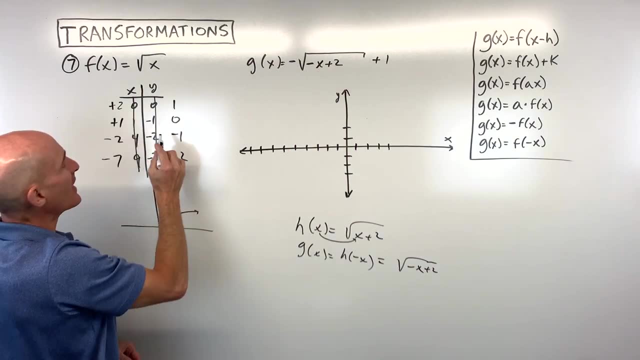 and then shifted up 1.. That's another possibility. You just want to make sure that this comes last Here. the order is important, OK, So let's go ahead and plot these. So we've got 2 comma 1, which is going to be right about here. 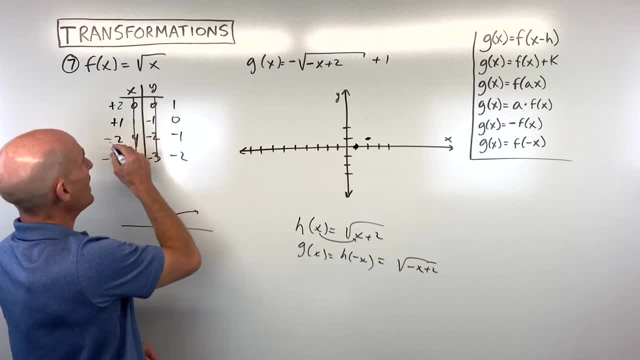 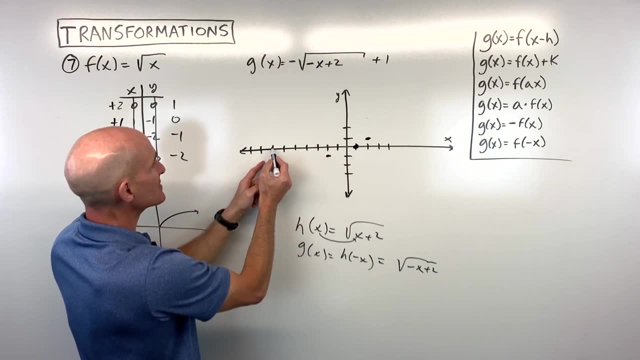 OK, 1, 0, which is right here, Negative 2, negative 1 is right there, And negative 7, negative 2.. Let's see So: 3,, 4,, 5,, 6,, 7, negative 2.. 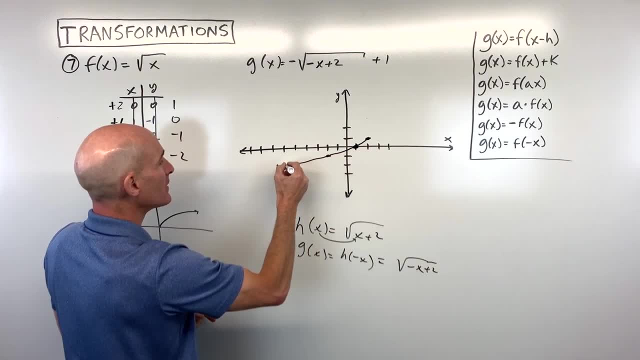 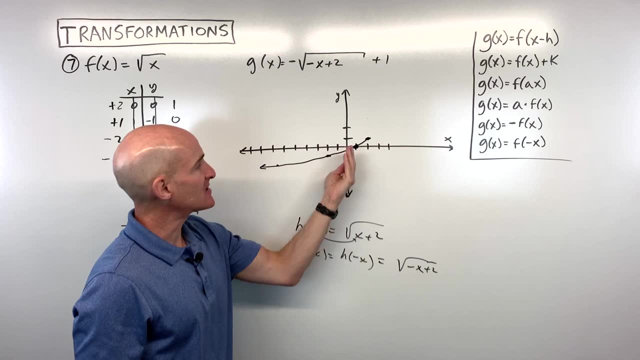 So you can see this graph is bending kind of like that. OK, So domain would be well from negative infinity to 2.. Or you can say: x is less than or equal to negative 2. The range would be: y is less than or equal to 1.. 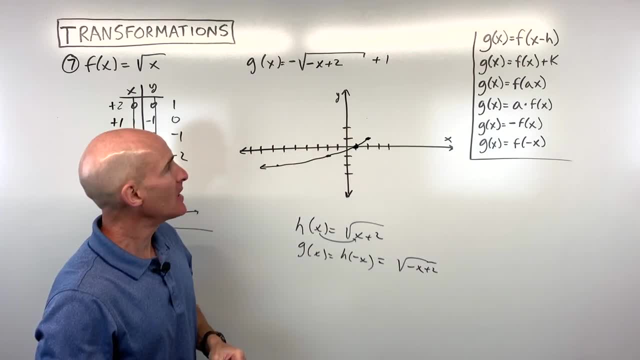 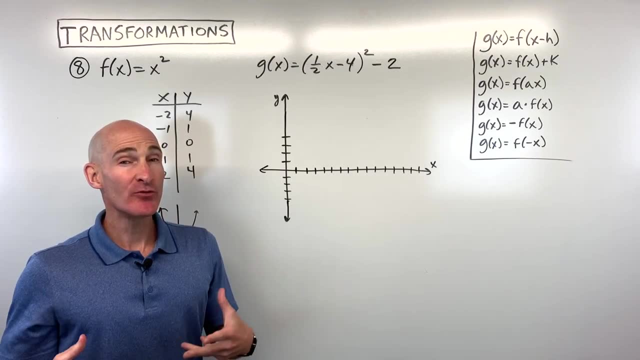 Or you could say negative infinity to 1 if you're using the interval, Or you could say negative infinity to 1 if you're using the interval notation. So great job if you were able to get that one. Let's take a look at a few more examples. 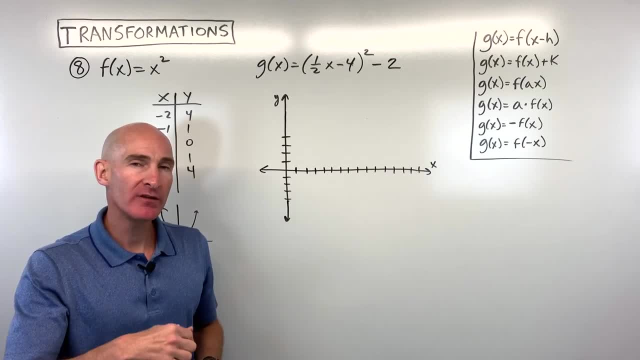 I know these transformations can be really challenging for a lot of students. If you have a question, put it in the comments below And if you're catching on to this, see if you can help some of those commenters out, kind of walking through why these transformations work the way that they do. 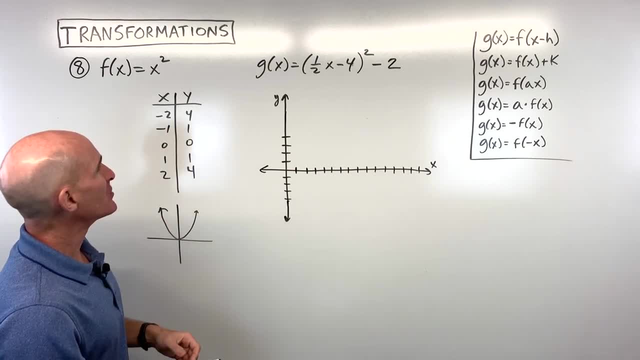 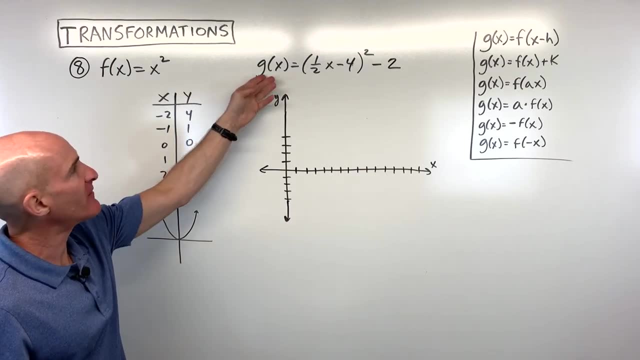 And try to see if you can answer those questions. You learn something through explaining. You kind of learn it at a deeper level. But yeah, Comment below if you have a question. Let's look at this one here. now We've got g of x equals the quantity 1 half x minus 4, squared minus 2.. 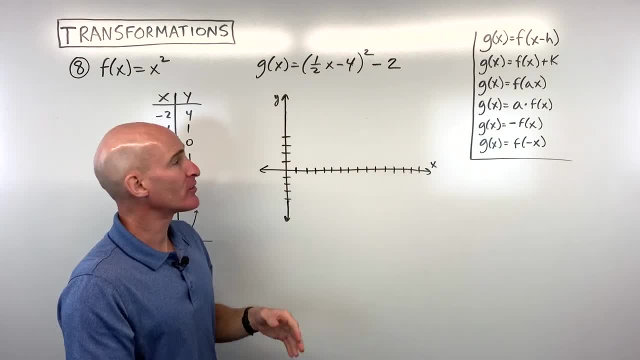 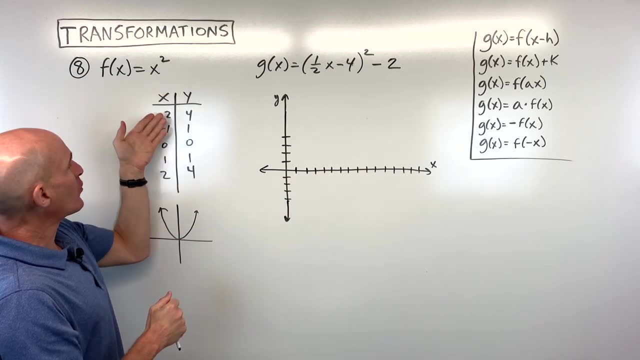 See if you can label the order of transformations, what you would do- first, second, third, fourth, fifth, et cetera- and see if you can get a good sketch of your graph here Now, if I was going to do this problem. we've already talked about the quadratic table. 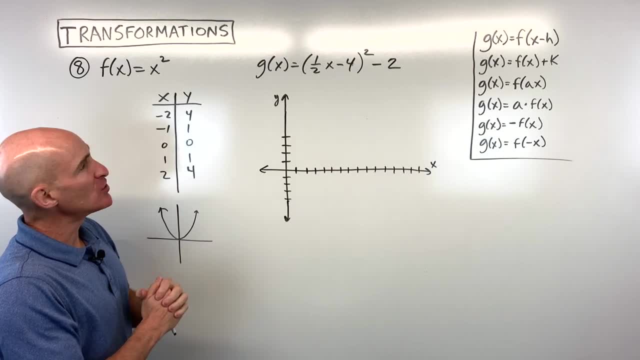 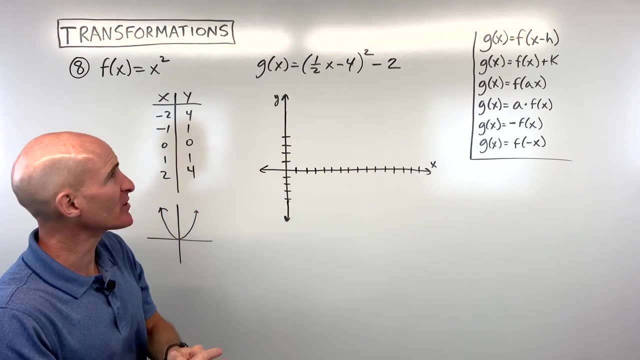 and the basic graph, that basic parent function. So what I would do is I'd say: well, how could I, if I was building up this function, how could I build it up? Now, some teachers, OK, and some people explain this, like when you have more than one quantity. 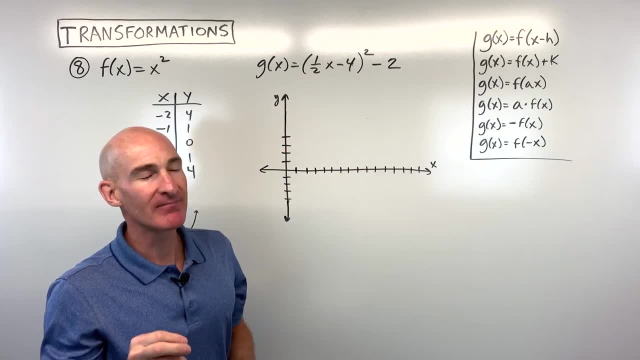 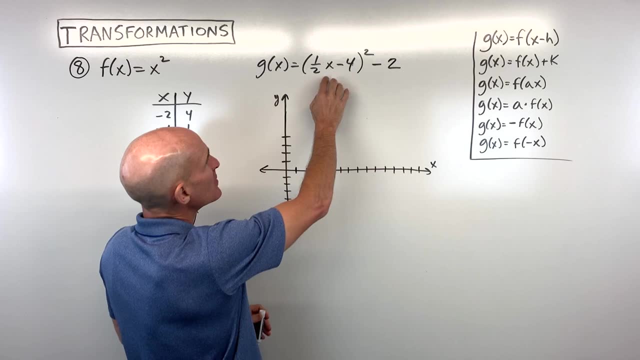 grouped with the x, like this. what they'll say is that it has like the opposite of the PEMDAS. You know how you do parentheses, exponents, multiplication, division, addition, subtraction. So what they would say is they'd say, well, you've got multiplication here and subtraction here. 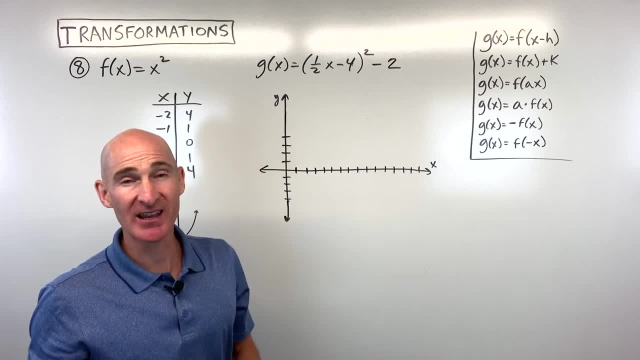 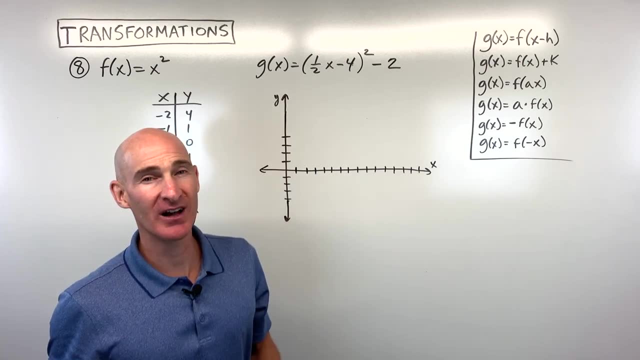 Normally you do multiplication first and subtraction second, right. But when you're doing the order of transformations and it's grouped with the x, like that, you would actually do the opposite direction of the order of operations. You would say: I'm going to do this. 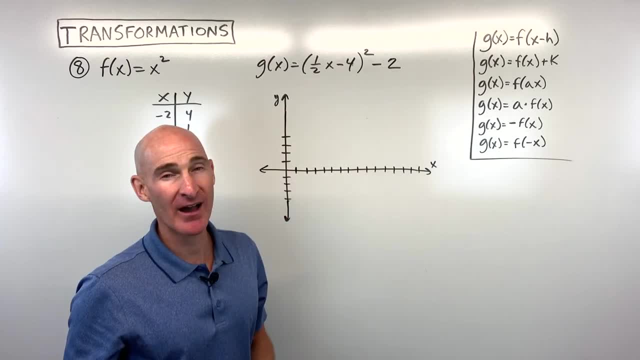 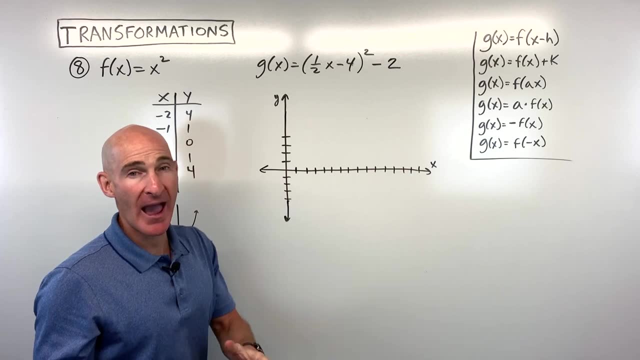 I'm going to do this minus 4 first and then the multiplication by 1 half second. It's like counterintuitive. I find that to be a little bit confusing. It's a good little hack or a quick way of doing it. 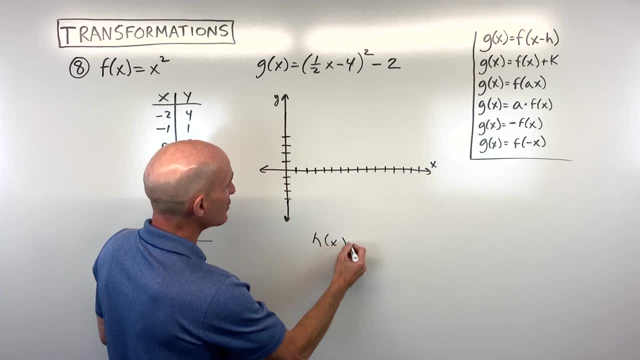 but I like to kind of think of how would I create this function? I might start off by saying h of x equals x minus 4, squared right, And then what I'm doing is I'm replacing this x. let's call this g of x. now. 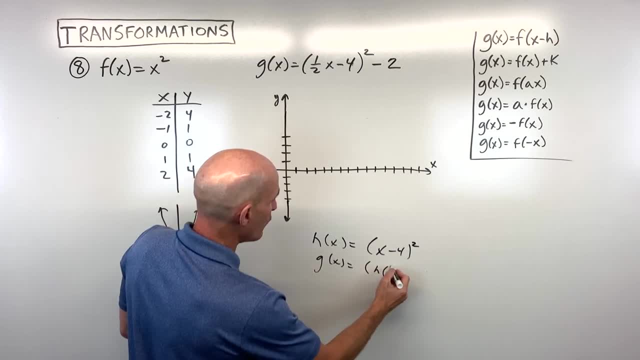 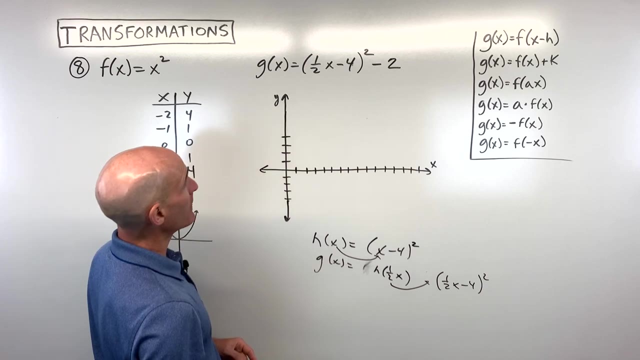 with h of 1 half x. Okay, I didn't need this parenthesis here. Now what happens is, whatever is in parenthesis here goes in for x. So what I'm going to do is I'm going to replace x with 1 half x, like that, right. 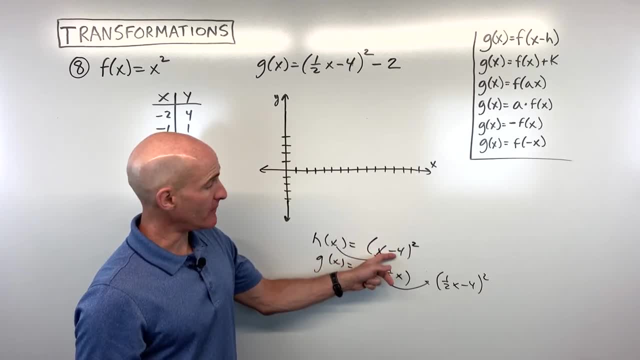 So what happened first? Well, you can see this is kind of like our starting function, The minus 4, it's grouped with the x That's going to shift it right, 4.. So let's add 4 to all the x's. 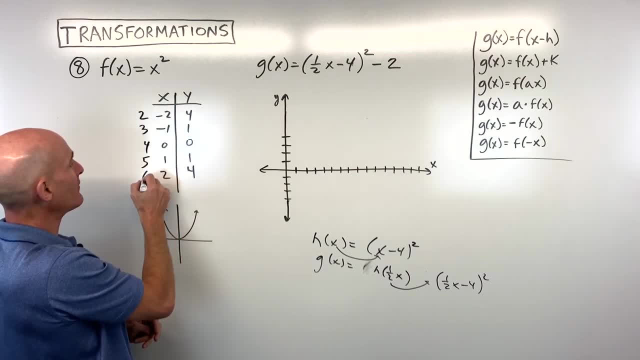 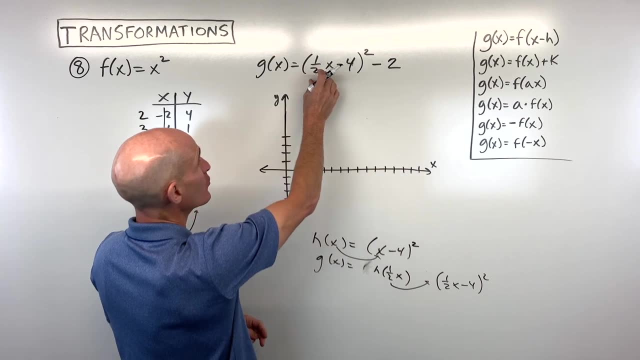 That's going to be 2,, 3,, 4,, 5, and 7.. 6. And then you can see we replace that x with the 1 half x. Okay, so it's grouped with the x, It's multiplied, which is going to be a stretch or a shrink. 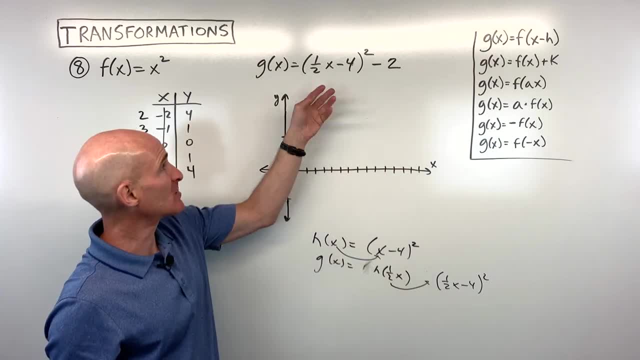 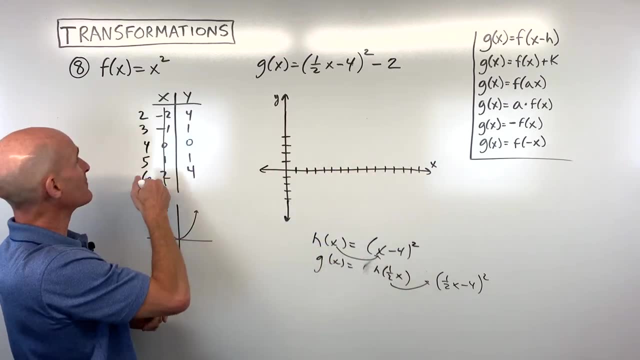 When it's grouped with the x, it has the opposite effect or reciprocal effect. In this case, you're going to be multiplying the x's by 2, which is a horizontal stretch- by a factor of 2,, which means I'm going to multiply all these x values by 2.. 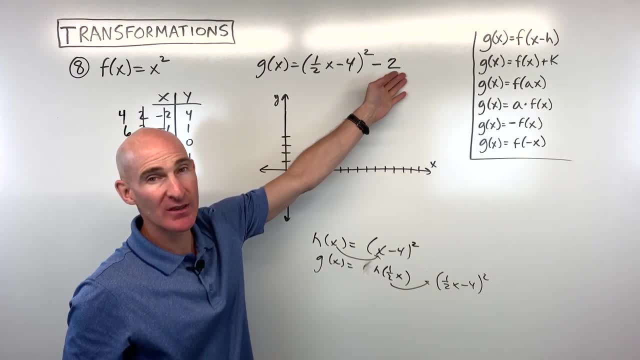 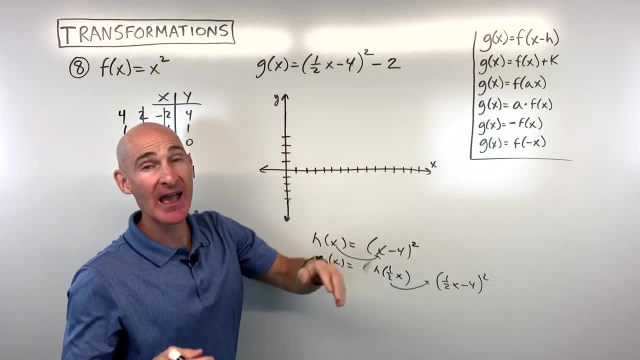 Cross out the old ones. And then, lastly, remember we always want to do that vertical shift Up or down. last, The minus 2, it's not grouped with the x, so we know it's affecting the y values. It has the same effect. 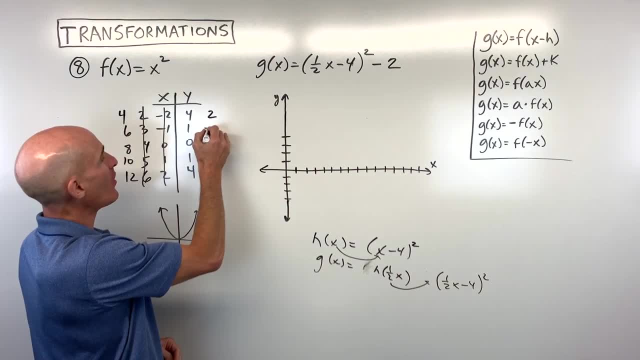 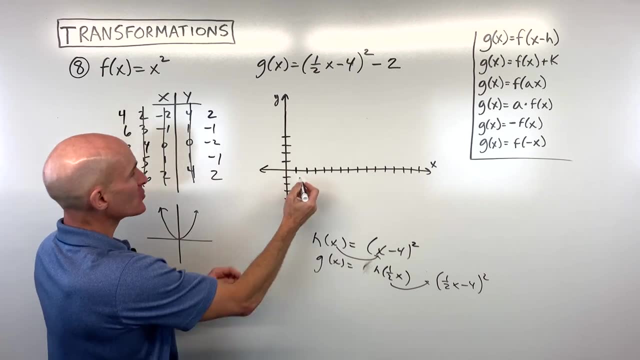 Minus 2 is going down 2.. So we're going to subtract 2 from all the y values, Cross out the old ones, And now we can plot these points. So let's go ahead and do that. So 4, 2 would be right about here. 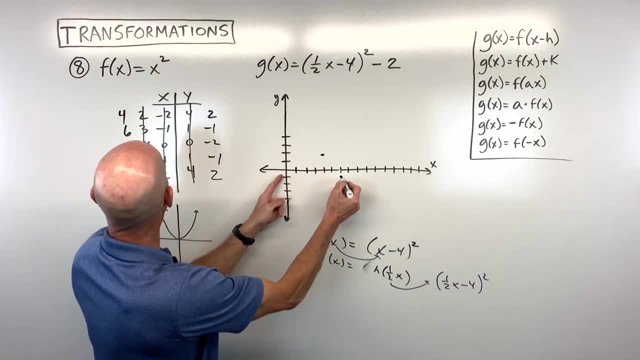 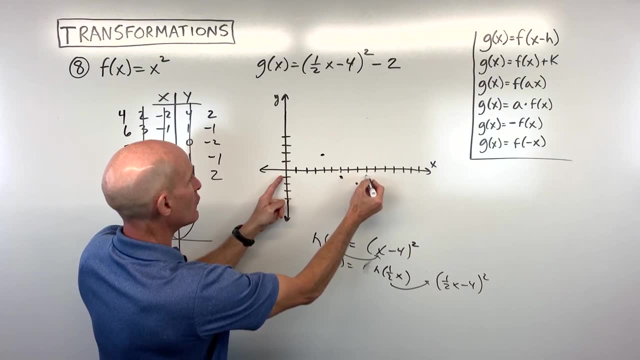 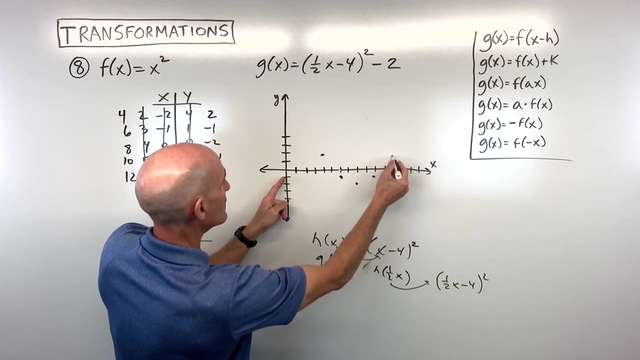 6, negative 1 would be right about here. 8, negative 2 would be right about here. 10, negative 1 would be, let's see 9,, 10, right about here And 12, 2 would be right about here. 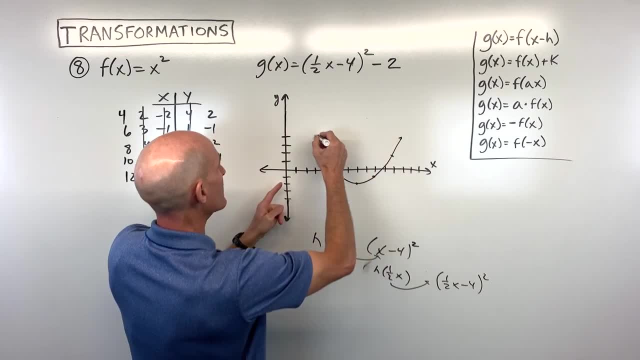 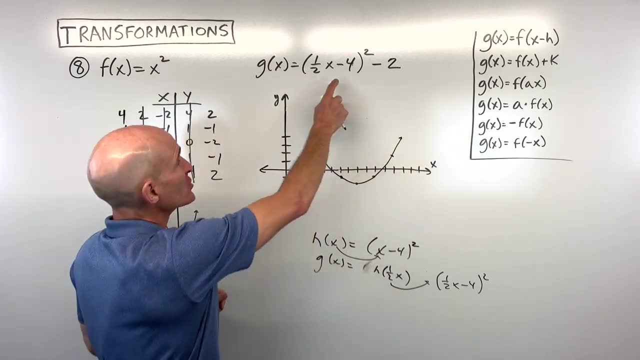 Okay, so this is something like that, right, So you can see that the graph is wider. right, That's what this did. But first we shifted it right 4, okay, which would be right here, But then when we stretched it, see that vertex now. 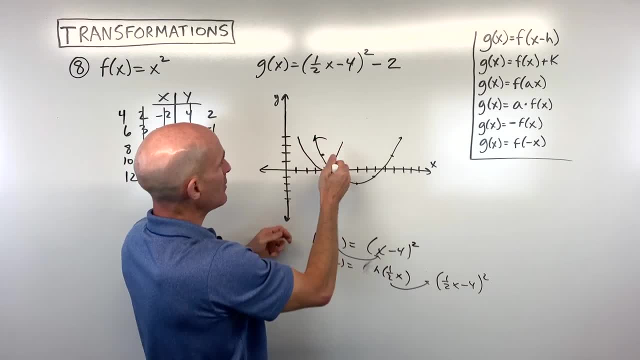 see when we first was at right, 4, like this: when we stretched it, the x is by 2, the horizontal stretch- this point, went over here to 8. Then we shifted it down 2, and that's how we're getting that new graph. 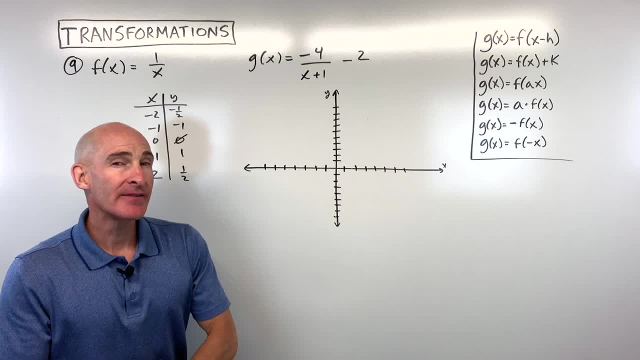 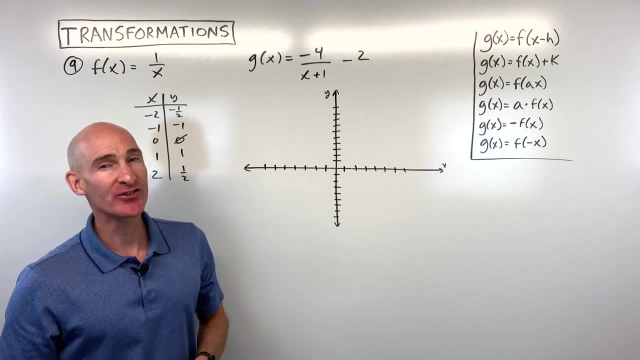 So let's take a look at another example. I like that quote by Madame Curie, I believe it is. She said that nothing in life is to be feared, only to be understood. So I know these can be really challenging, but I hope you're catching on to this. 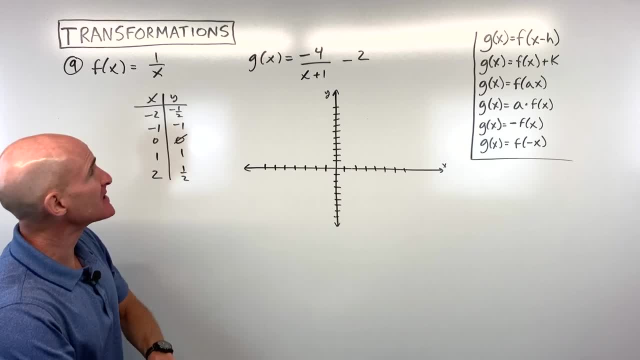 And if you stuck with this video so far, great job. We've got a couple more examples. Let's look at number 9.. We've got f of x equals 1 over x. This is called the reciprocal function, And some easy numbers here to plot would be like a negative 2, negative 1, 0, 1, 2.. 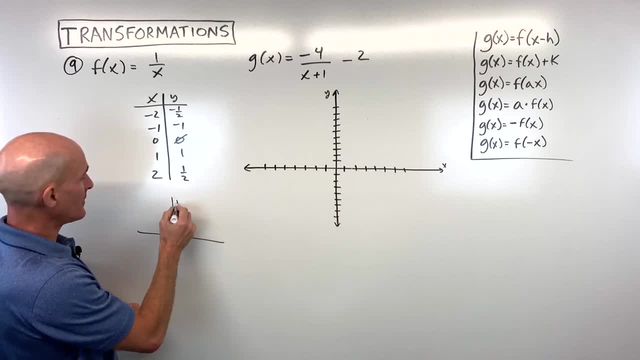 And you're going to get these y values And when you graph it, it's going to look something like this: It's a hyperbola. It gets closer and closer to the x-axis and the y-axis. You've got some asymptotes here, right at the x-axis and the y-axis. 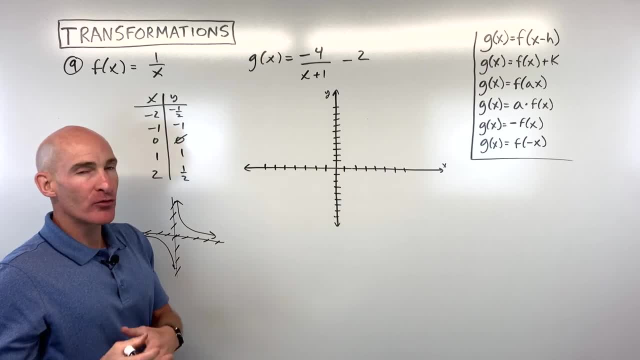 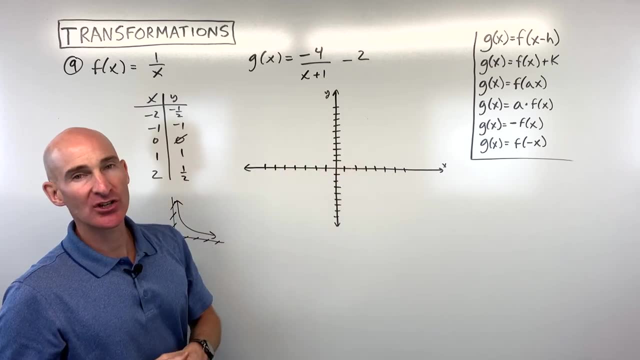 That's your basic graph. So let's see if we can go through the order of transformations. So what are the first, second, third transformations here And how would you graph it? How could you get a good sketch? See if you can do that one. 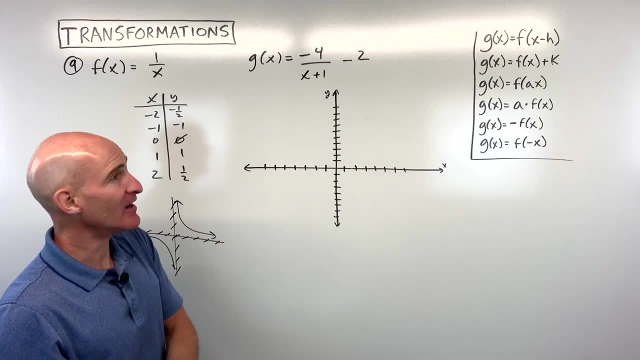 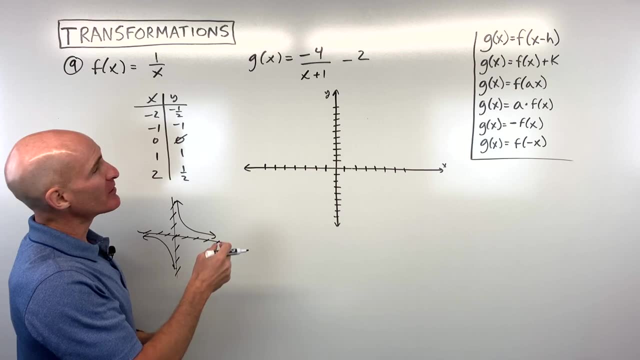 Keep in mind that there's more than one order where you can get the same answer, but there's definitely a wrong way to do it as well. So if I was going to do it, I would think about building it up like we were talking about using these function notation here first, 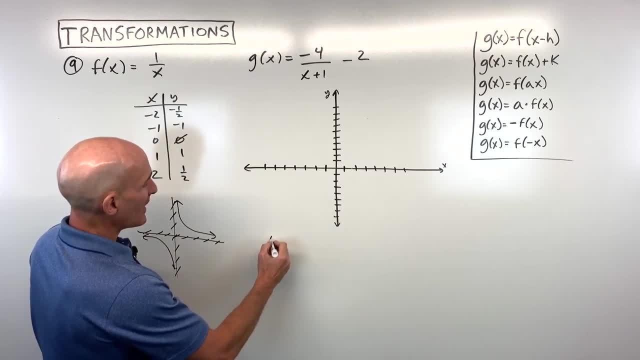 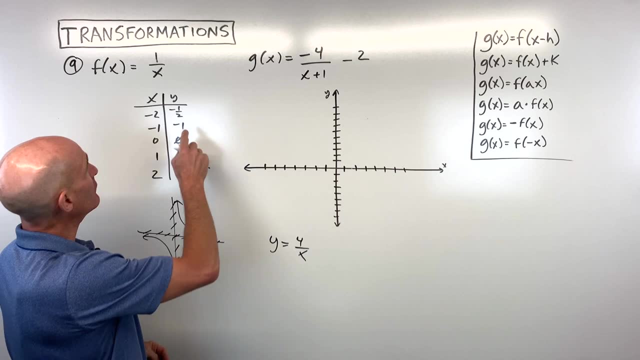 So what I might say is: let's maybe look at a function like this. Let's just say you have y equals 4 over x. Okay, so what did I do to get from 1 over x to 4 over x? Well, it looks like I multiplied by 4, right? 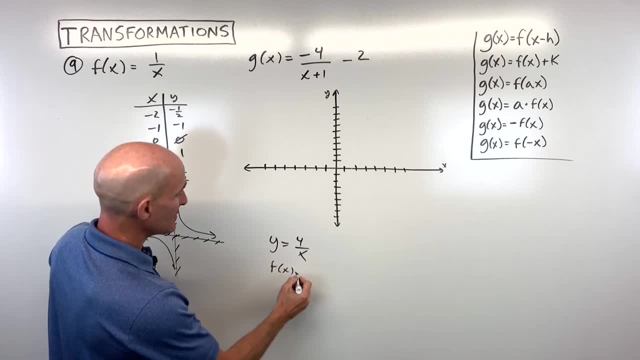 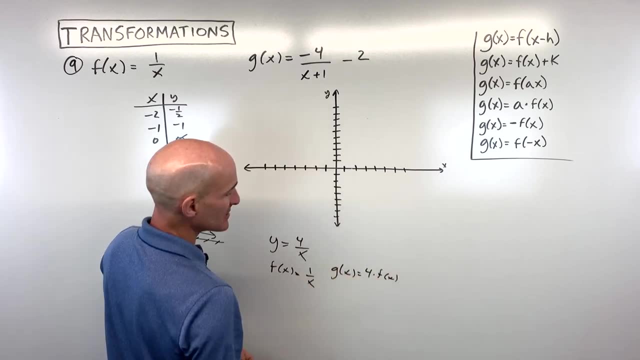 It's basically like if I had my function: f of x equals 1 over x and now let's say I have g of x is equal to 4 times f of x. That's this one right here. So see how it's not grouped with the x. 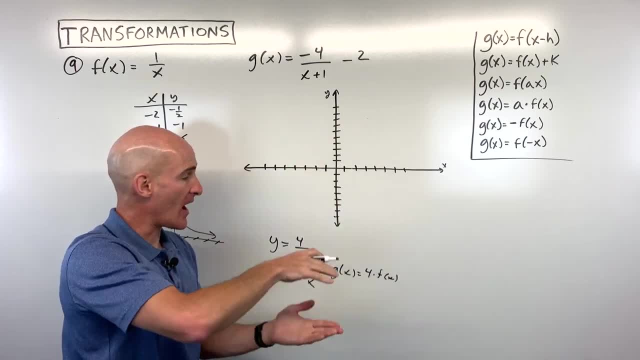 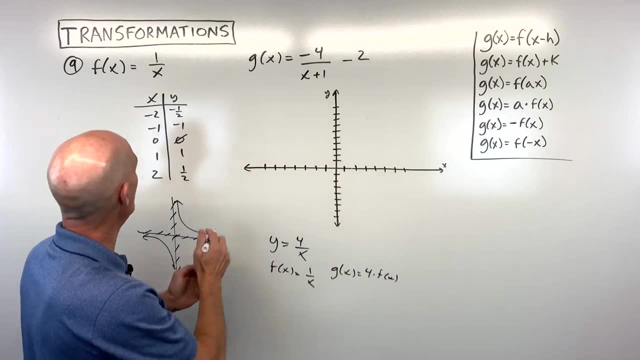 It's affecting the y values. That's a vertical stretch. Remember, when you multiply it's a stretch or shrink. It has the same effect when it's acting on the y. so it's stretching or multiplying the y's by a factor of 4.. 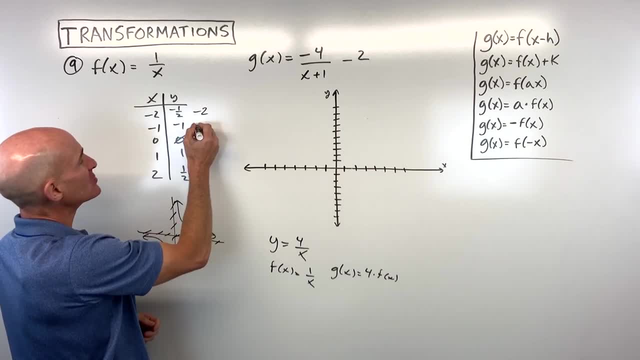 So if I multiply all these by 4, I get negative 2, negative 4.. This is undefined, so we won't worry about that. one 1 times 4 is 4, and 1 half times 4 is 2.. 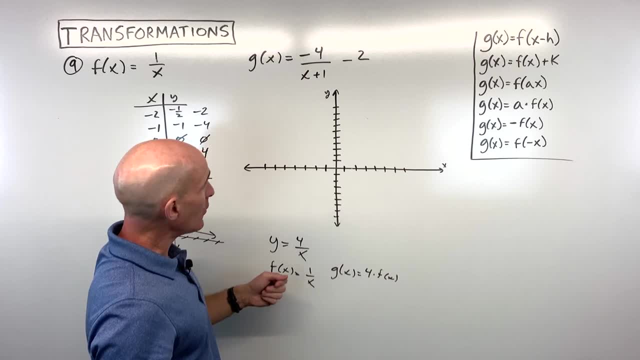 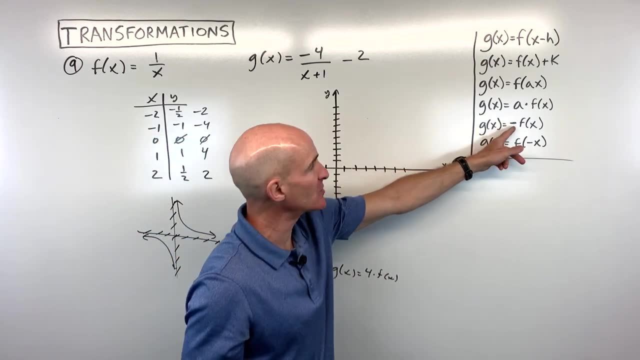 Now, this negative here. what's this negative doing? Well, the negative, you can see, it's taking this quantity here and it's multiplying it by negative 1.. So that's going to be this one, right here. It's not grouped with the x. 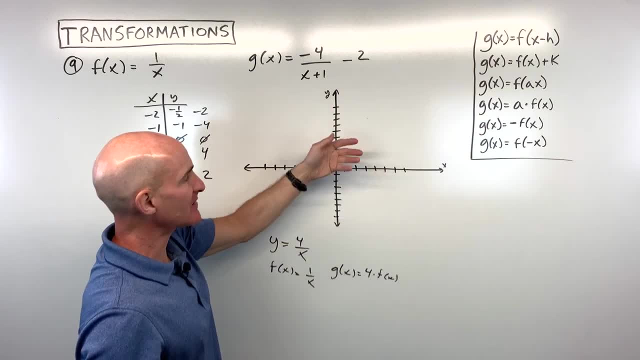 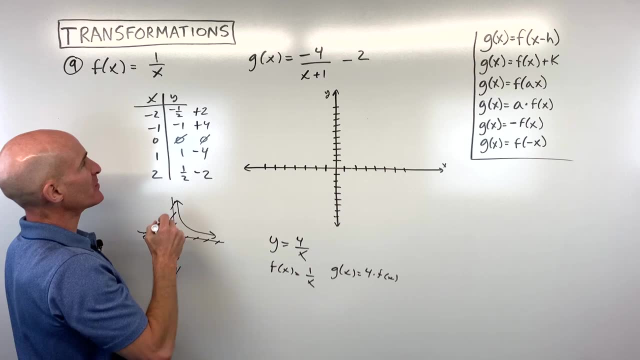 It's affecting the y values, which all the y values are the opposite. That's going to reflect it over the x axis. So we're going to multiply all the y values by negative 1.. Okay, so I'm just flipping the signs. 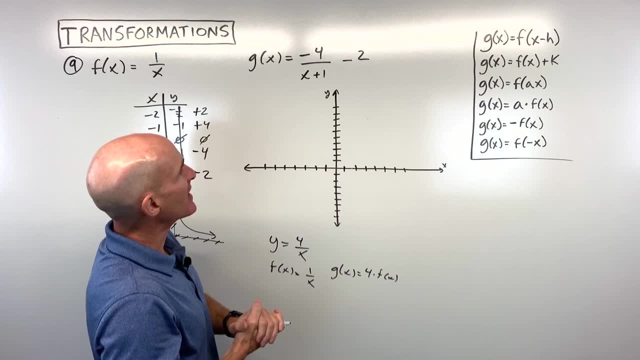 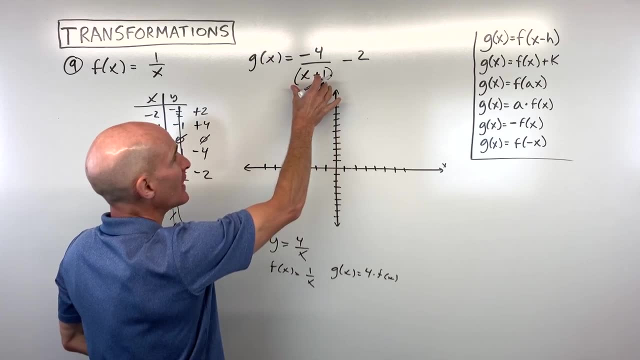 And then now let's look at this x plus 1 here. So this x plus 1 is going to shift the graph left: 1.. See, it's grouped with the x Okay, it's with the x Okay And it's having the opposite effect. 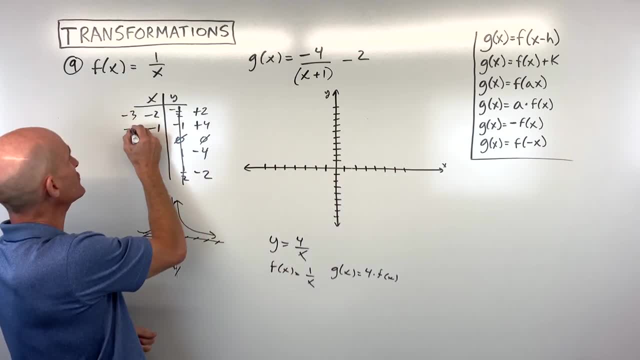 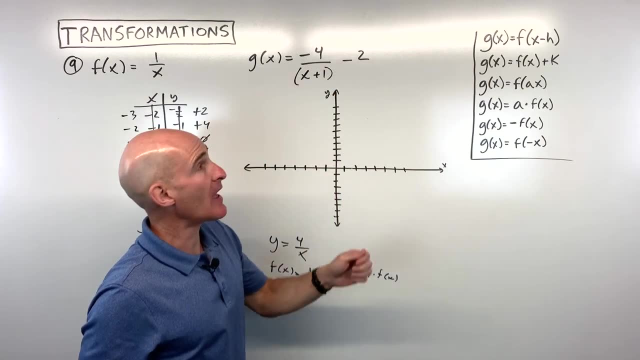 So shifting it left 1, which means I'm going to subtract 1 from all the x values here, Cross out the old ones And then lastly remember we want to do the vertical shift up or down last. So the minus 2 affects the y values. 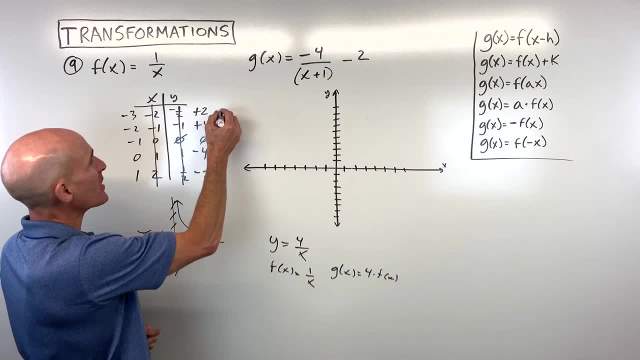 It has the same effect. It's shifting down 2.. So we're going to subtract 2 from all the y values here, So 0,, 2, negative 6, and negative 4.. Cross out the old ones. So let's see if we can plot this now. 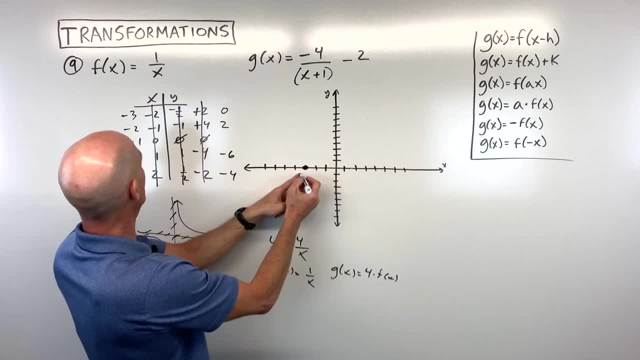 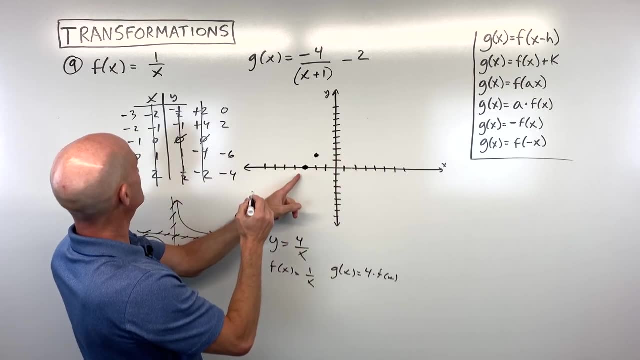 So we have negative 3,, 0. Put a point there. Negative 2, 2. Okay, And 0, negative 6.. 1,, 2,, 3,, 4,, 5,, 6. And 1, negative 4.. 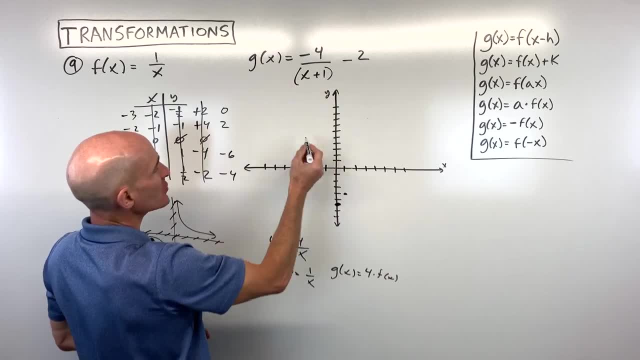 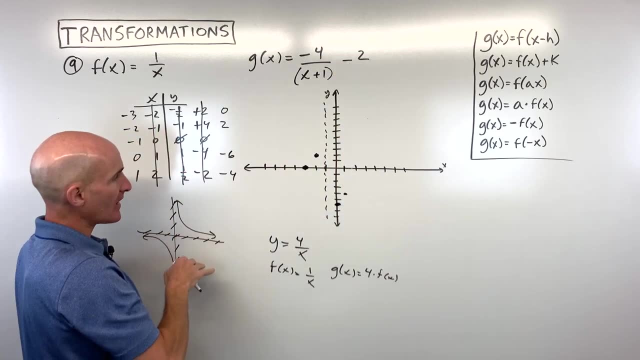 And what's interesting here is you can't divide by 0.. So at negative 1, you would have a vertical asymptote. This minus 2 shifts everything down 2. So this horizontal asymptote is being shifted down 2. So you have a horizontal asymptote at y equals negative 2.. 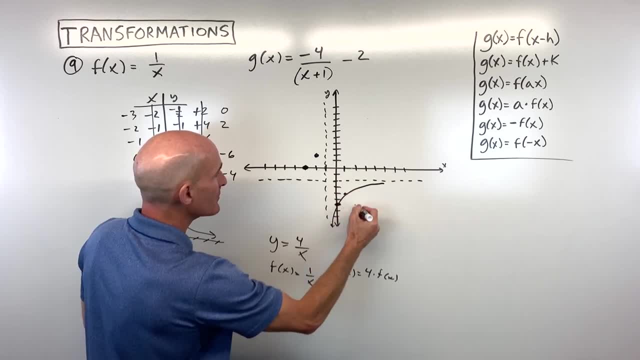 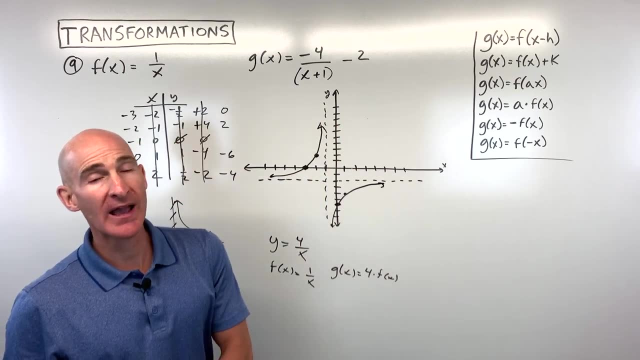 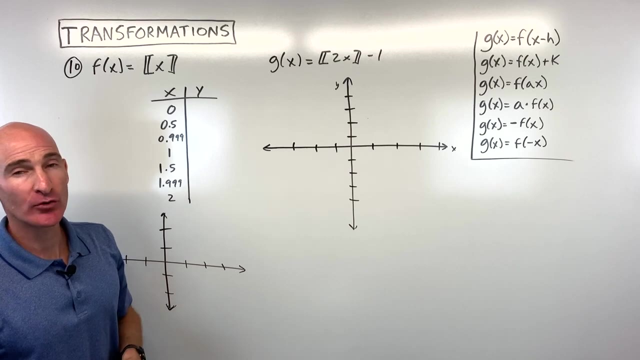 And so your basic shape here of your graph would look something like this. And you got it. So let's try one last example. Okay, we've got f of x equals the greatest integer function. So the greatest integer function. what this does is it always rounds down to the nearest integer. 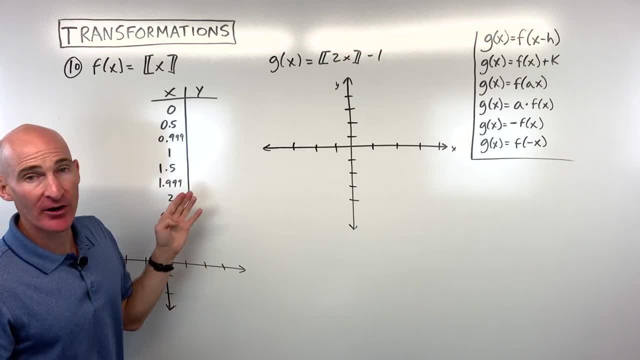 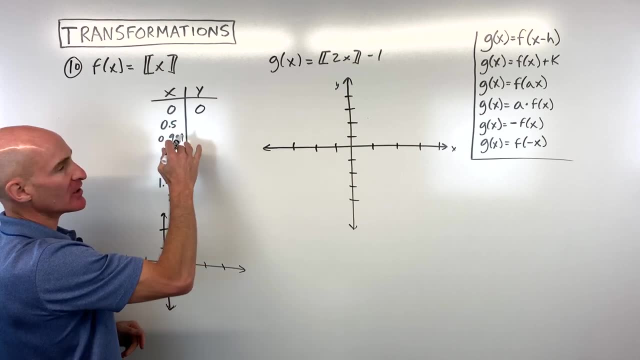 Okay, and it's oftentimes referred to as the step function, because when you graph it it looks like stairs. So here what we do is we put 0 in. 0 would round to 0.. It's already at the integer value. 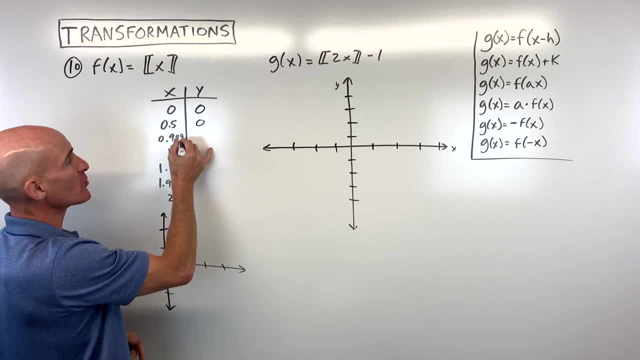 0.5 would round to 0.. 0.999 would round to 0., But at 1, you would stay at 1 because you're already at that integer value. 1.5 would round to the left on the number line to 1.. 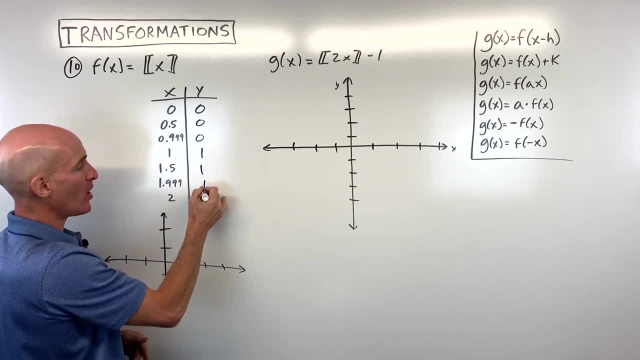 1.999 would round to the left on the number line to 1.. And then 2, you're at the next integer 2.. So if we plot these points see 0, 0 would be right here: 0.5, 0.. 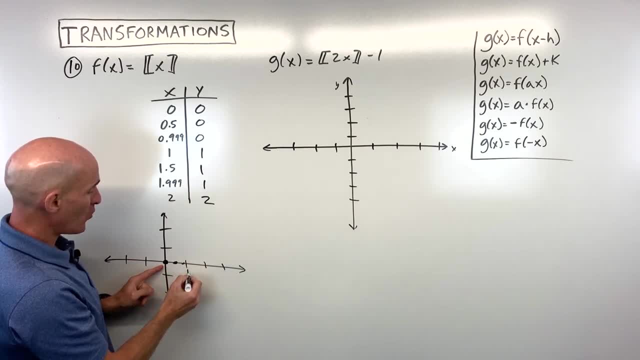 0.999, 0.. But as soon as you get to 1, there's going to be an open circle here and you're going to jump up to the next step or stair. Okay, 1.5 would be 1.. 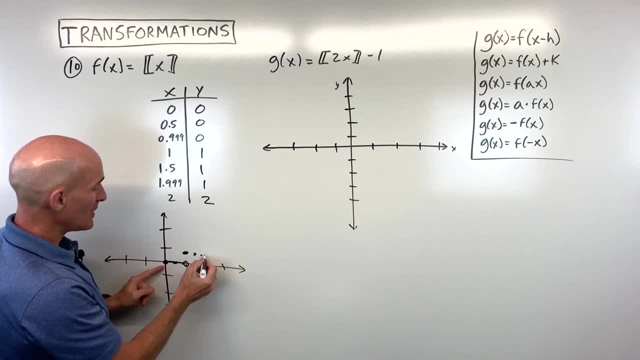 1.99 is 1.. As soon as you get to 2, here there's an open circle and you jump up to the next step at 2.. Once you get a few of these steps, you can repeat it. So, as you can see, it's open on the right and closed on the left. 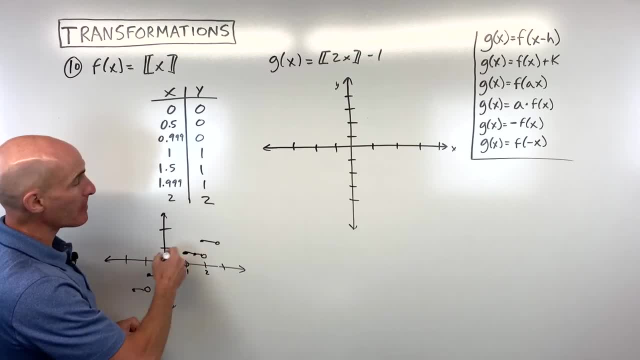 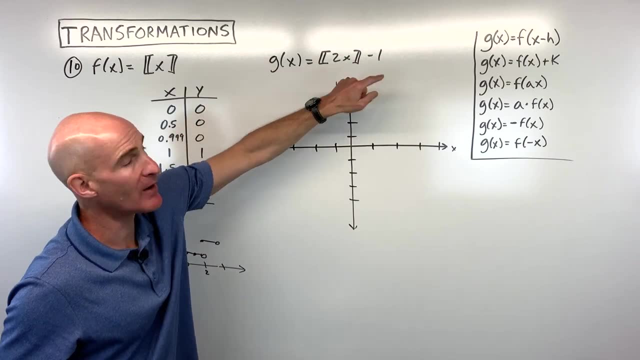 And it just keeps going in both directions like that. So that's your step. So that's your step function, your greatest integer function. But what do you think this here would do? the 2x minus 1? What's the order of transformations? 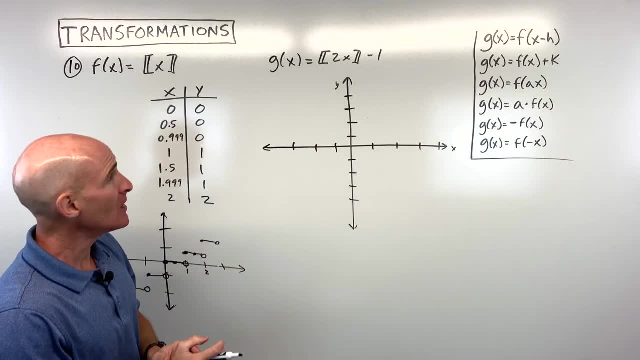 How would you get a good sketch of that graph? Try that one. Well, like I said at the very beginning, I like to work from the inside out. So I would say: hmm, this 2 is grouped with the x. That means it's going to affect the x direction, the horizontal direction. 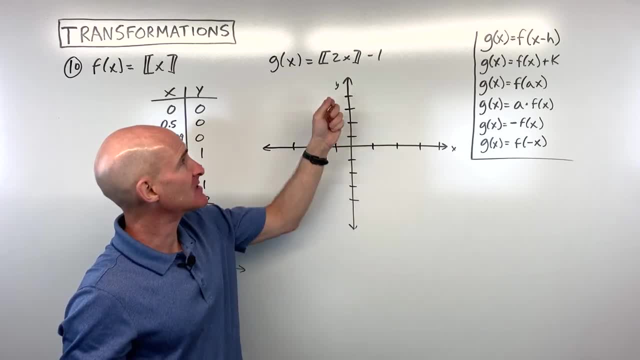 When it's grouped with the x, it has like the opposite effect. What I mean by that is, if you know you're multiplying by 2, you're actually going to divide the x's by 2 or multiply by 1 half. 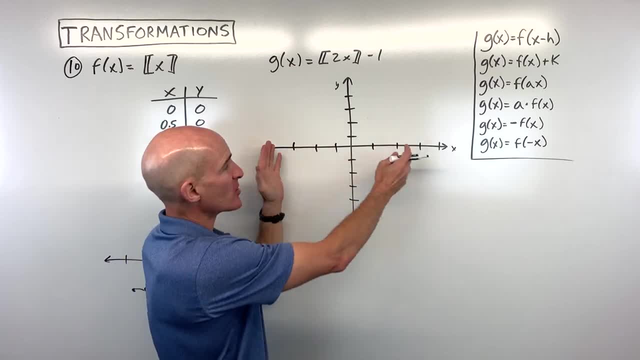 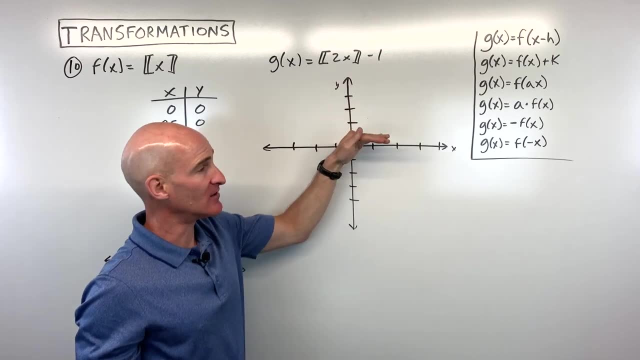 Either one, it's the same thing, And when you're multiplying and dividing that's a stretch or a shrink. So this is actually going to be a horizontal shrink by a factor of 1 half, And then the minus 1 is going to shift it down 1.. 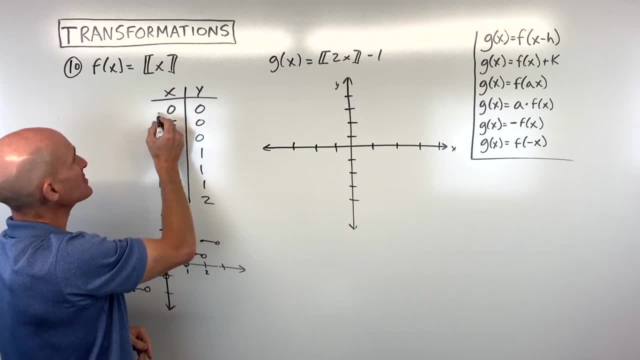 So horizontal shrink by a factor of 1 half means I'm going to multiply all these numbers by 1 half. So this is going to be 0.. This is going to be 0.25.. This is going to be like 0.499.. 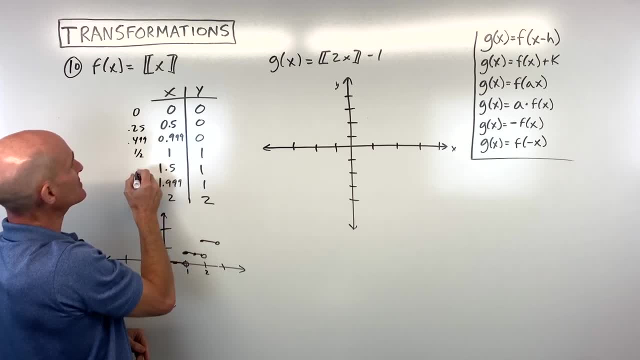 This is going to be a half. This is going to be 0.75.. This is going to be like 0.999 roughly And this is going to be 1.. Okay, now the minus 1 is going to shift everything down 1,. 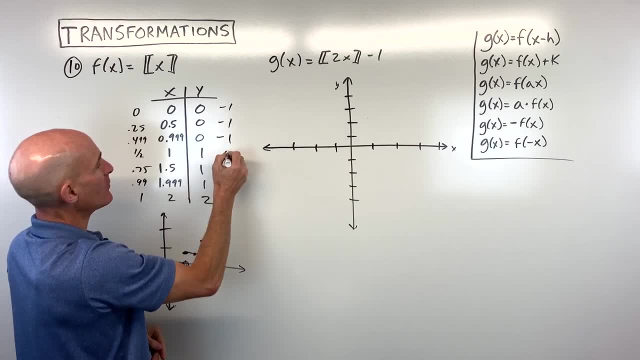 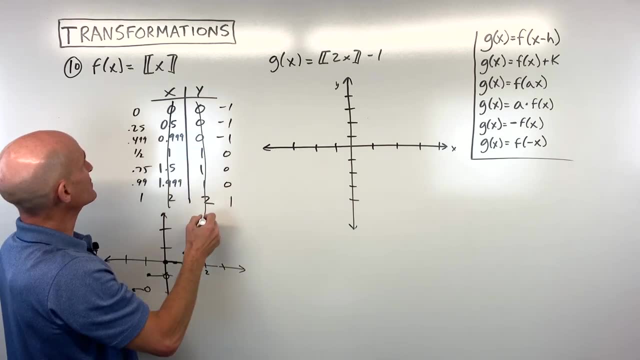 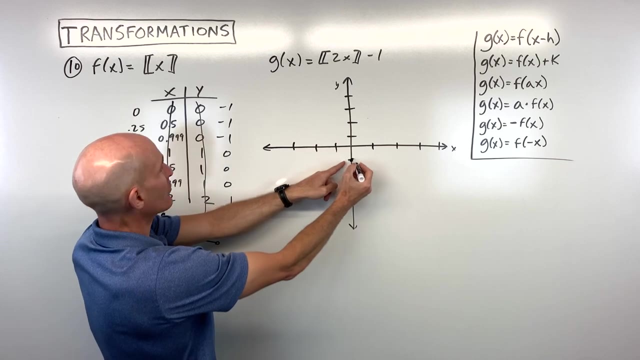 which just means I'm going to subtract 1 from all of these y values. Okay, so now, if we plot these, let's see what this looks like. So we have: at 0, we're at negative 1.. At 0.25, we're at negative 1.. 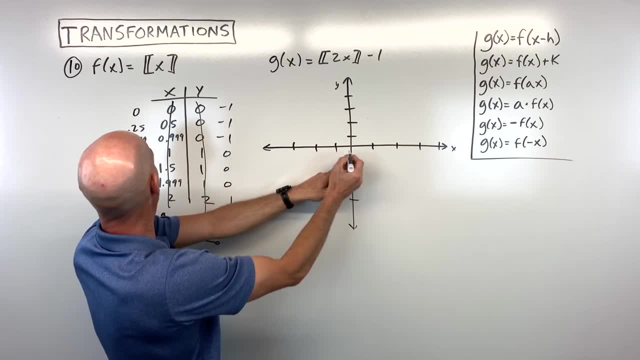 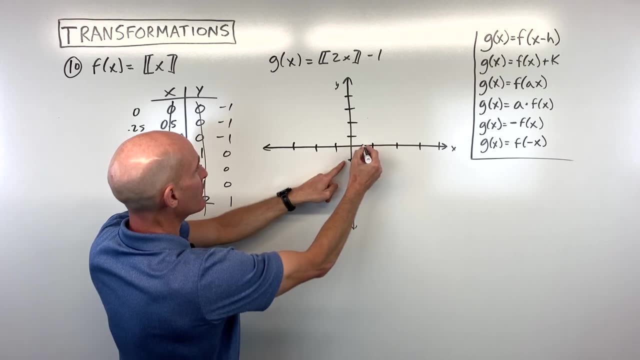 At 0.499, we're at negative 1.. At a half, we're at 0.. So what happens is that, right, you go all the way up to a half and then you jump up like that, Okay, and then you can see 0.75, I'm at 0.. 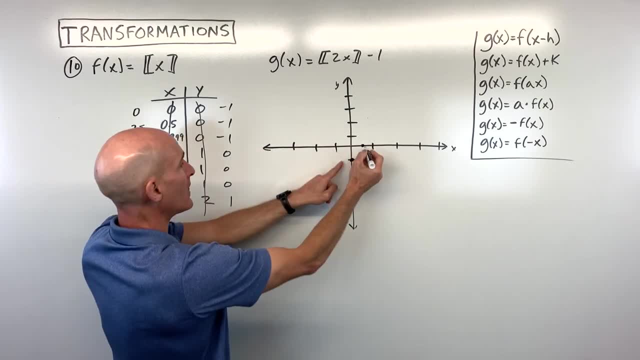 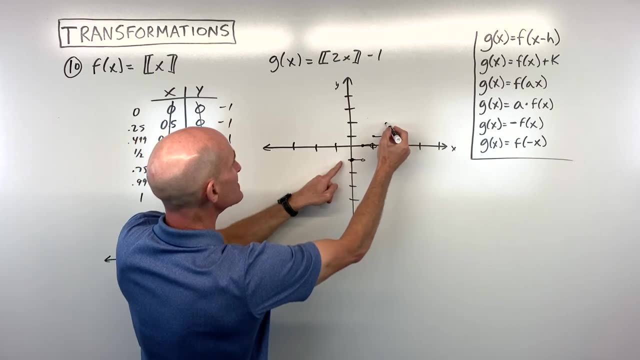 0.99,, I'm at 0. And as soon as I get to 1, I jump up to 1.. So that means it's going to be open here and I'm going to jump up like that. So what's happening now? if you can see this, 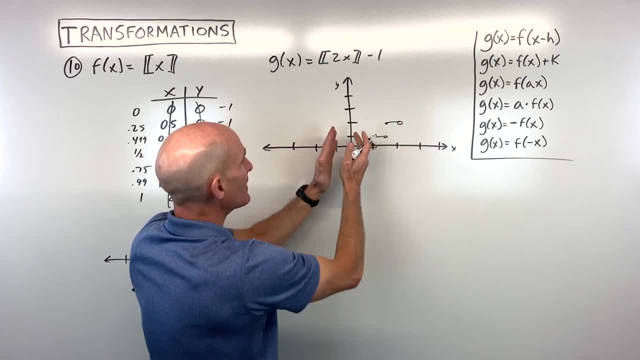 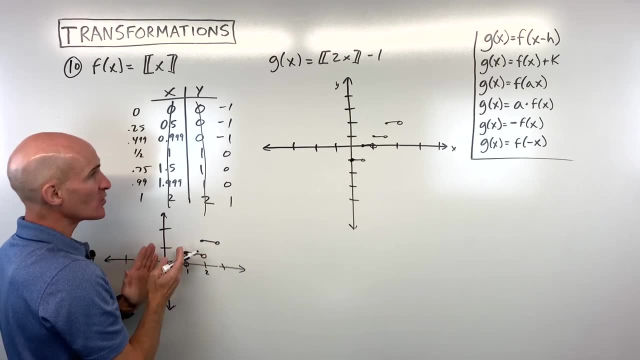 is the 2 divided the x values by 2, so that it made all these stairs like half as long, right? So if you squeeze it towards the y axis they're half as long. And then the minus 1, we shifted it down 1.. 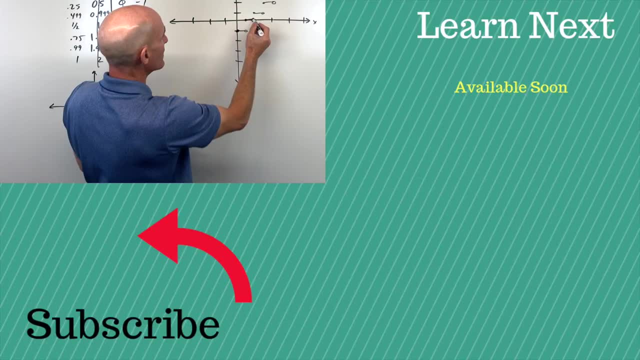 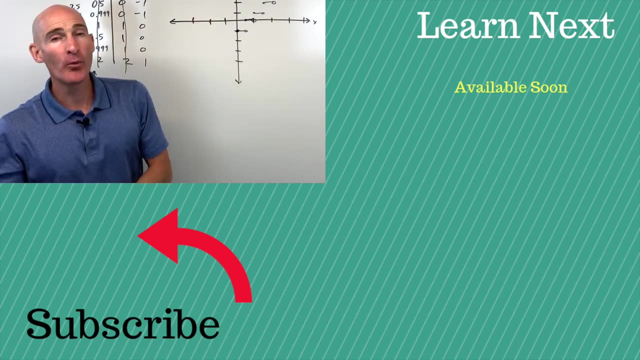 So basically, every half on the x is jumping up, as opposed to every 1 integer it's jumping up, So and it continues. So great job. I hope this made transformations a lot easier for you to understand If you want to get more.